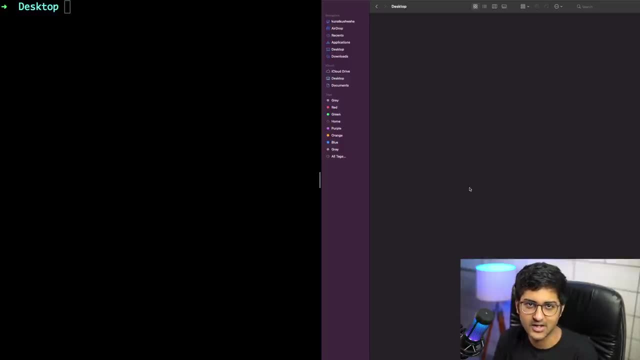 back in the past. So let's say you have an application and you want to collaborate with it. in the past you know in that code base in which my application was running. I wish there was some sort of a way to you know, click a picture of that code base and whenever I want the picture like: 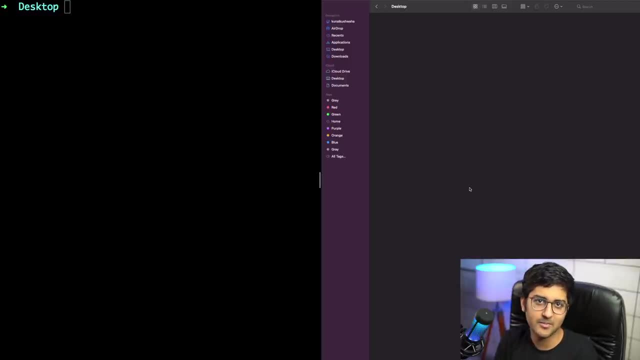 that exact code base as it was during that time in the past. I could have that. So basically saving the history of your project like on, let's say, first July, your project looked like this. second July, your project looked like this. third July, your project looked like this, like some additional. 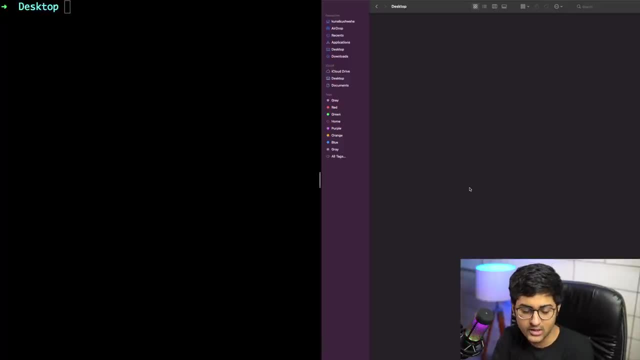 files, code changes or whatever. You want to go back to how your project looked on first July. your project looked like this. third July, your project looked like this: like some additional july- you can do that. you want to go back to how your project looked on second july, you can do that. 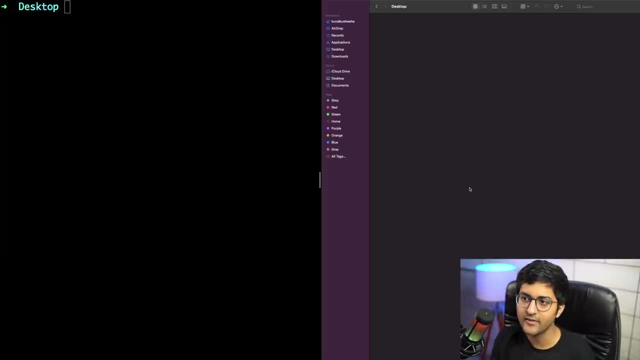 that's another. that's a use case that you can think of. another one can be: you are contributing to open source, for example, or you and your friends are contributing to one project. now imagine that a hundred people are contributing to just one folder. that is what happens in like. 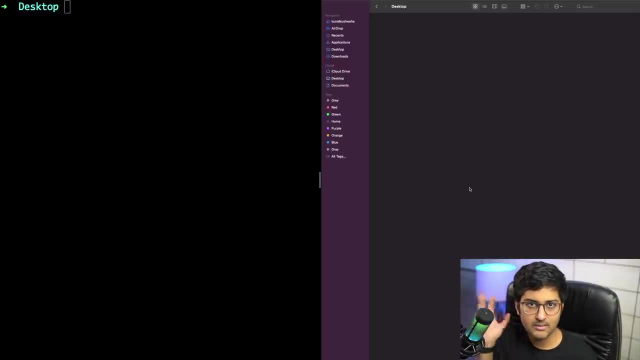 open source projects as well. there's one main folder and so many people are from around the world contribute to that project. now you might be wondering: how do these people share their code? if you want to share a code in some you know open source project, you want to add your own. 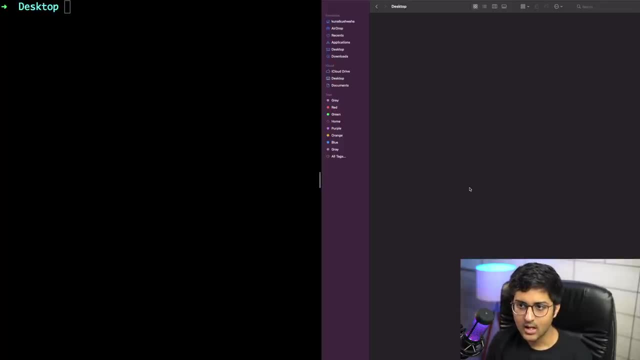 functionality or share some changes you made. how can you do that? we can do that via git and github. so git and github allows us to maintain this history of the project. at what particular point of time, which person made which change where in the project. git helps us in doing that. what is github? github is platform, an online website that allows us to host our git repositories. now you might be wondering: what is a repository? we'll look more into that shortly. repository is basically just a folder where all the changes are saved. do not worry, if you don't know about it, we'll cover it in detail. 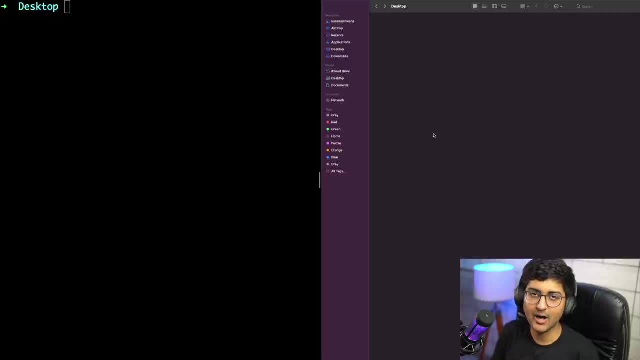 shortly. you can think of it as somewhat like this: so you have the email service right, so you use email and you have the email technology behind it and you know there's like the server and everything happening in behind the back end so that you can relate to with git. now what are? 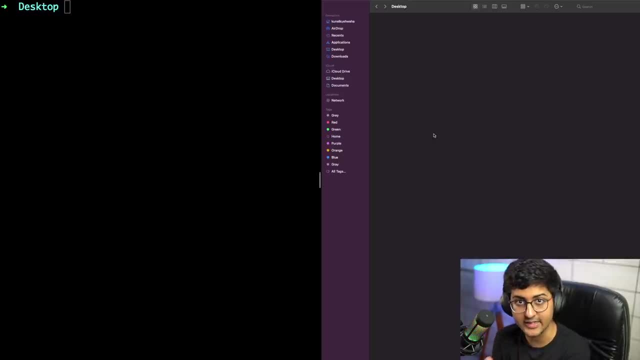 so many platforms that are providing you sort of like an interface to use this service to send emails to people around the world, to have, like the nice you know, gui, where you can see all your emails and everything- gmail, outlook, yahoo mail, so and so on and so forth- that you can relate with. 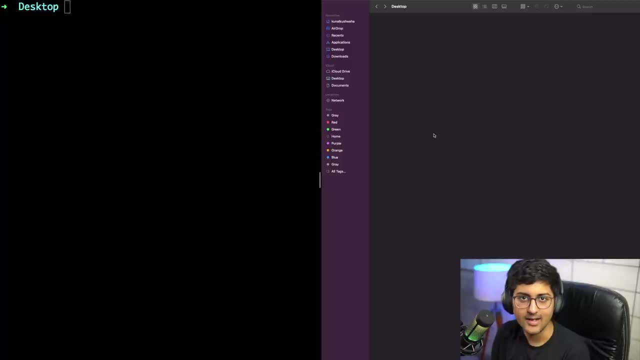 github or other platforms that allow you to do the same thing, like bitbucket, gitlab, for example. so git is like the- you know- version control system, like the tech, and there are so many other online platforms that allow us to host these folders or repositories, or our projects online. 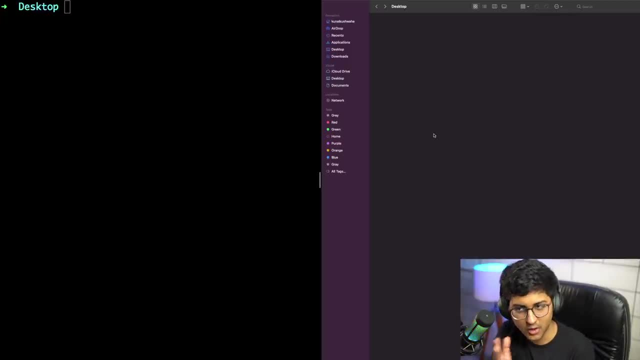 so that other people from around the world can share, look, contribute, and these are known as, like you know, github, bitbucket and gitlab. we will be using github because it's one of the most popular ones and, yeah, so it has a lot of nice, cool features. so that's the whole idea of why we are. 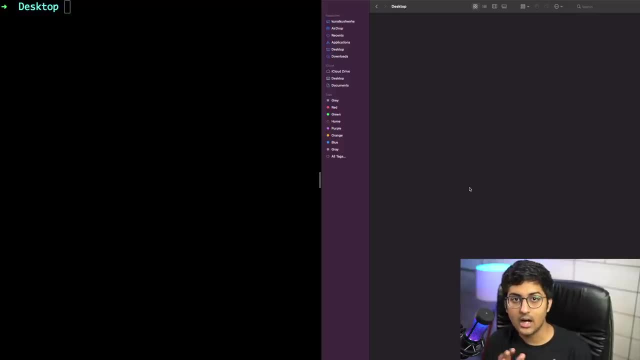 using git and github. not worry if you don't don't understand how we are using it, because that is going to be covered just for now. understand why we are using it: maintaining the history of the project, which person made which change in which project, when, and so on and so forth. like also sharing. 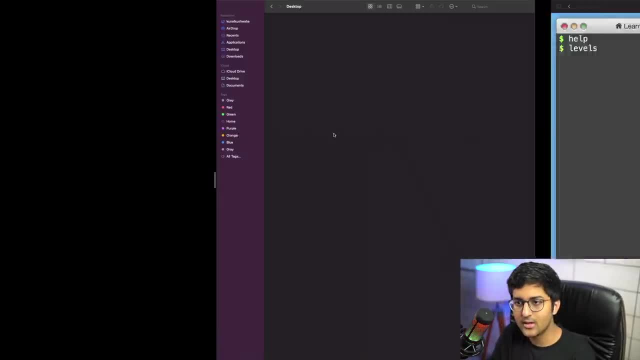 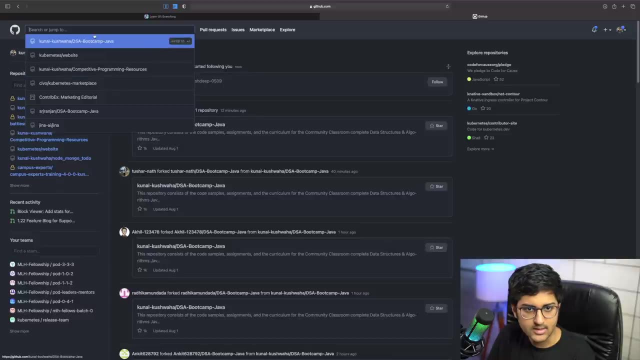 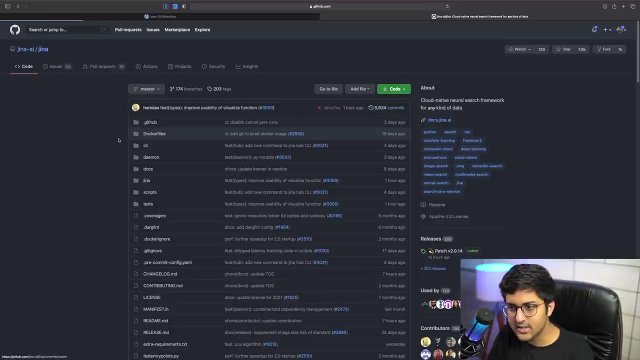 your code on github, sharing it with people around the world. so if i look into any project on githubcom, okay, let me look into any, let's say gina ai or whatever. i can see 5 900, so you can see, don't worry about what these things represent, we'll cover into it. 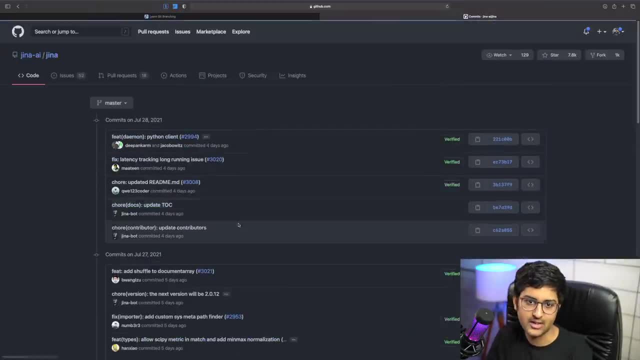 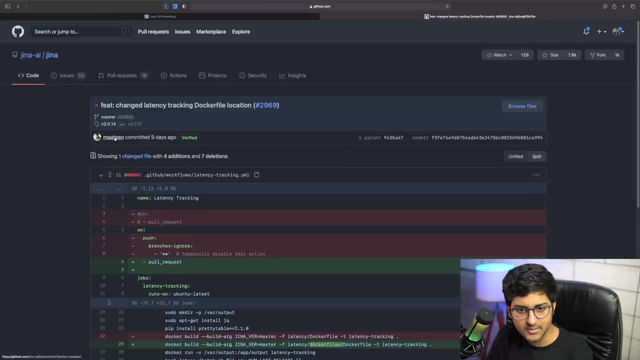 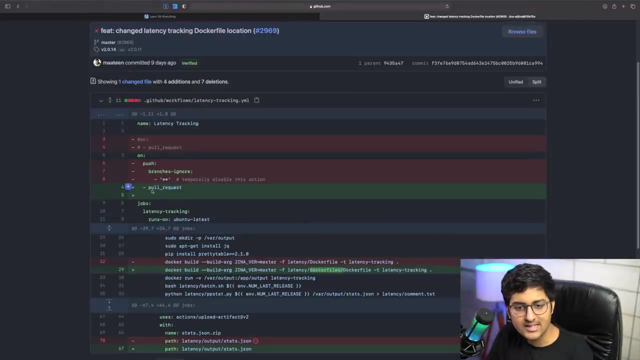 later on. these are base. this is basically the history of the project that i was talking about. history of the project, as you can see. so basically, uh, this person made these changes in the code base. red means that this line was deleted. green means that this line was added. so this person nine days. 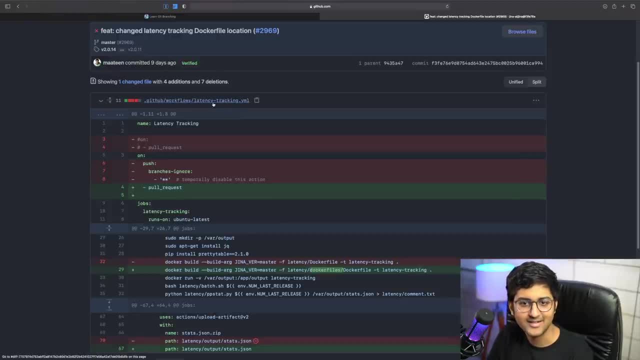 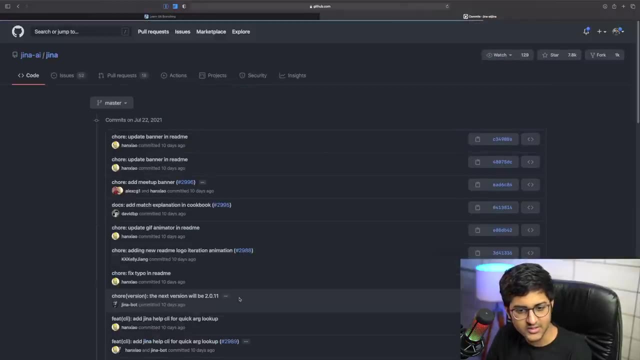 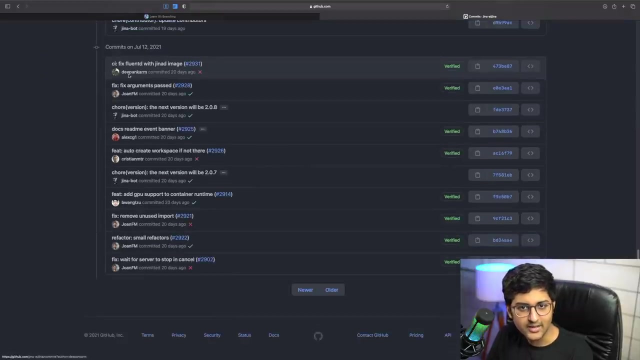 ago, made these changes in this file, so you can see the history of the project, and this goes on and on. you can even see the older history: on 16th july, these changes were made by someone. on 12th july, these changes were made by a lot of. 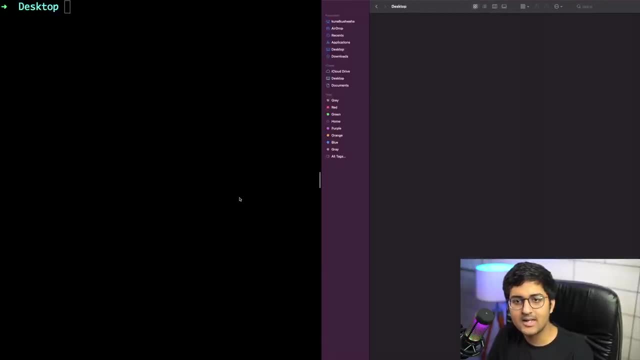 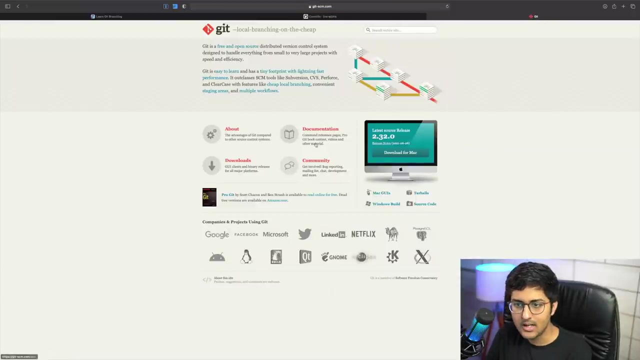 people. so that's basically the idea and that is what we're trying to achieve here. now let's look into how we do it cool. so first thing you need is you need to download git so you can go to git src, mcom and here you can download it. so you can download either for mac os, for windows or linux. 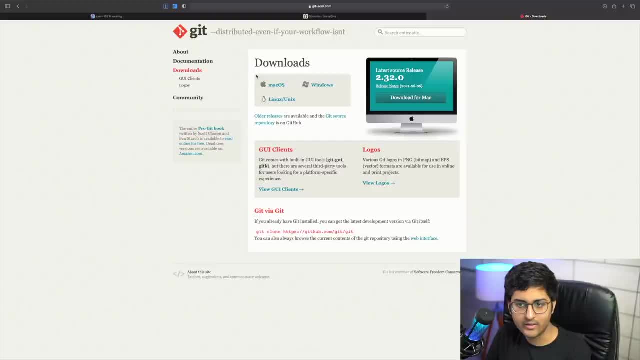 i would not recommend downloading the gui clients because we will be heavily focusing on the command line, like this terminal thing, so do not worry about the gui. i would recommend you to download it, the command line. okay, so you can download this and it's pretty easy to set up and 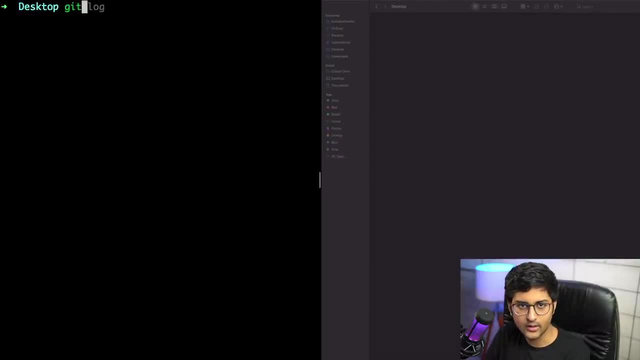 yeah, once you are set up, you can just write git over here and you can see. if you get the a list like this, it means that git is currently installed. okay, before we get started with the tutorial, now the hands-on part. so what is this structure over here on the left hand side? you? 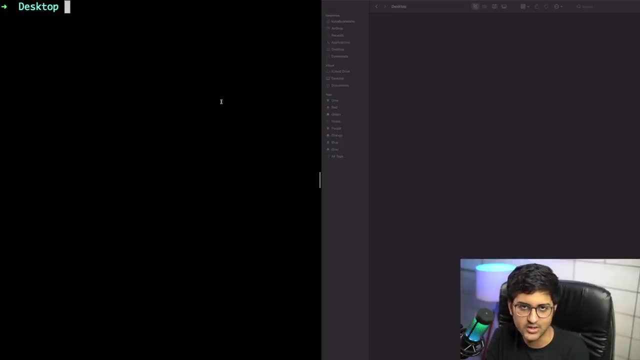 can see my terminal, normal command line shell. you can use cmd, windows, terminal, whatever, whatever you like. on the right hand side we have a folder, okay, so my terminal is currently in my desktop folder and this is just very basic commands and um what basically terminal allows us to do. if you're a 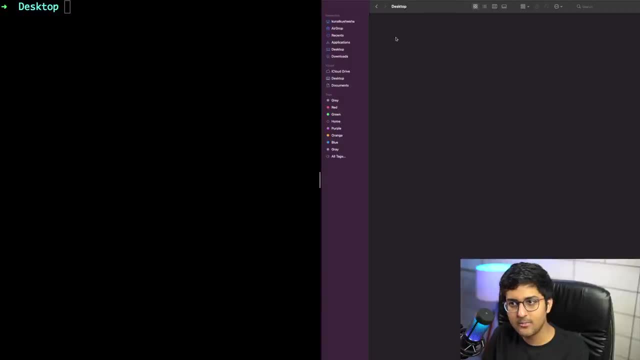 you know, you don't know much about it. it allows us to manipulate the file structure using commands. okay, that's basically what it's trying to do. so here you can see, this is the desktop folder. currently it's empty, and here, if i do list command, basically list all the things that are in my 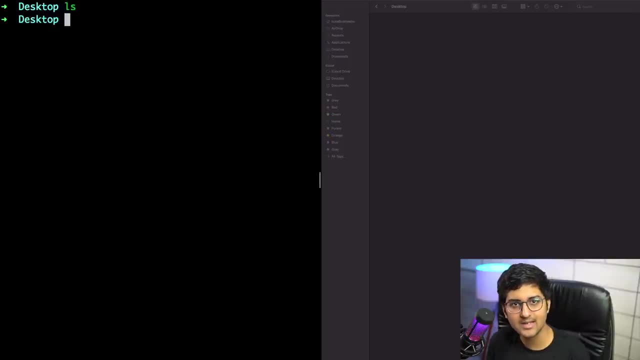 desktop folder empty. this does not show me anything. imagine, let's say, i want a project. we mentioned that we need a project in order to maintain the history of that project and do all sorts of things. share about it on github, you know. share it with other people, let other people contribute to it as. 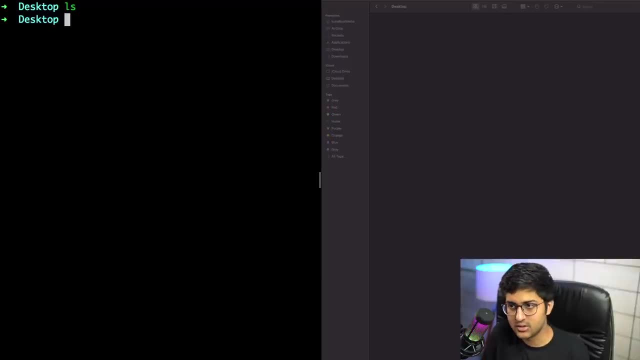 well, you want to do that, then how do we do that project? so you can either, you know, click right, click new folder, or there's a command for that mkdir make directory project. so you can see i made some change over here using a command and it was visible in my folder. project folder is being. 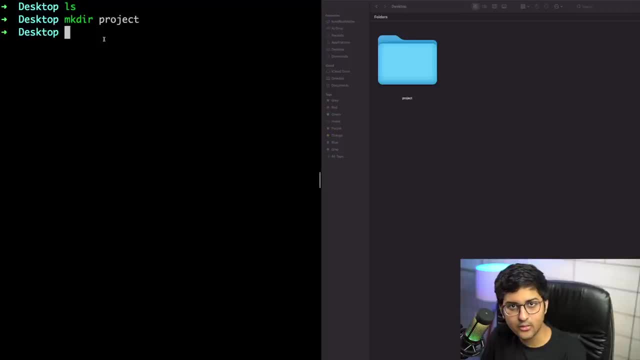 created. currently it's empty. i can change directory into it. now what do you mean by change directory? kunal, change directory means something like this: double clicking on it. now i'm inside this folder. how do i double click in the command line and go inside the folder? if i do list, you can see. 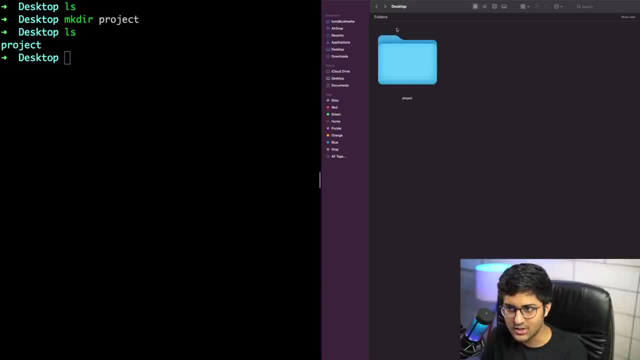 desktop should contain project. that is true, because desktop contains the project folder, and here also i'm seeing it. this is just a list command. i can also go inside this folder: change directory project. now i am inside the project folder. this is the view round, if i do. 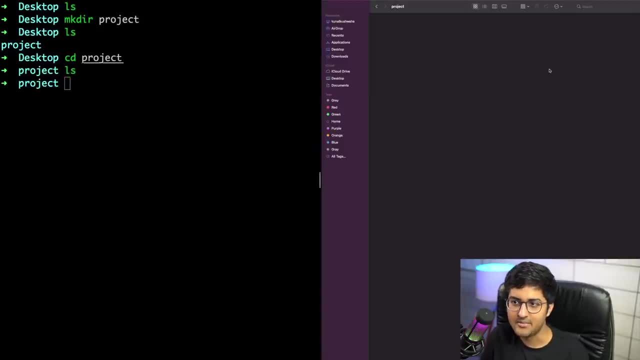 list. again, i can't see anything because this is empty. so now we have our project. let's say, now we want to maintain the history of this project using git. where is this entire history being stored? i create a new file that will be in the history. i make some changes in the file that will be in. 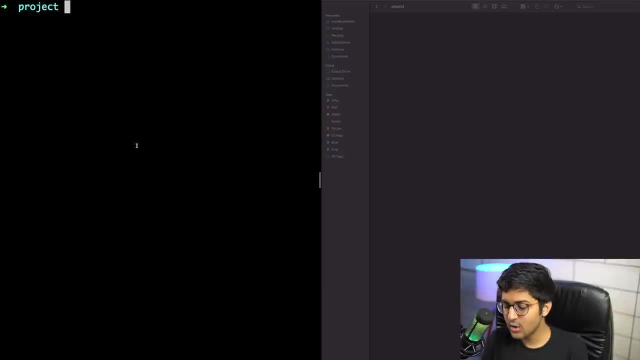 the history. i delete the file that will be in the history, so all of these histories are basically stored in another folder that git provides us. this is known as a git repository and it's named dot git. that is the name of the folder dot in. like linux systems and like mac os and stuff. 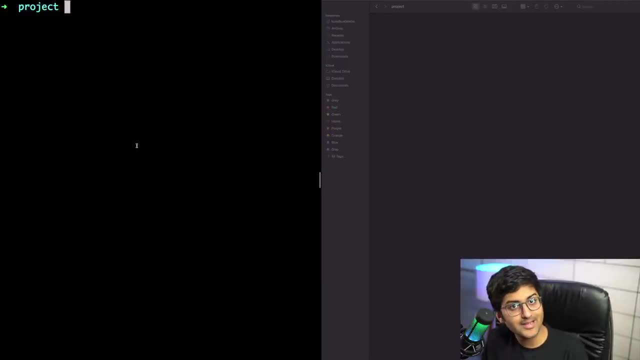 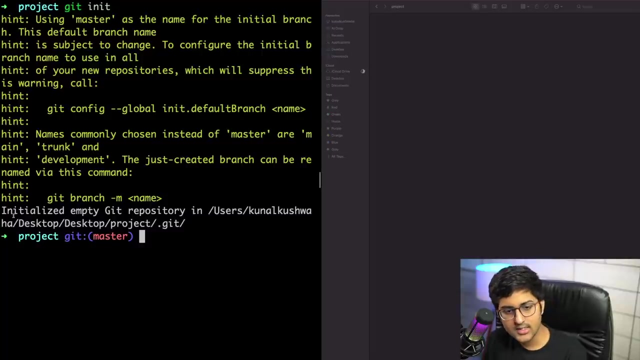 these are files that are hidden. and how do we get this dot git folder? how do we get this folder where all the history is being saved? just write the command git init: initialize an empty git repository. repository means a folder. okay, so you can see. it says: initialized empty git repository. 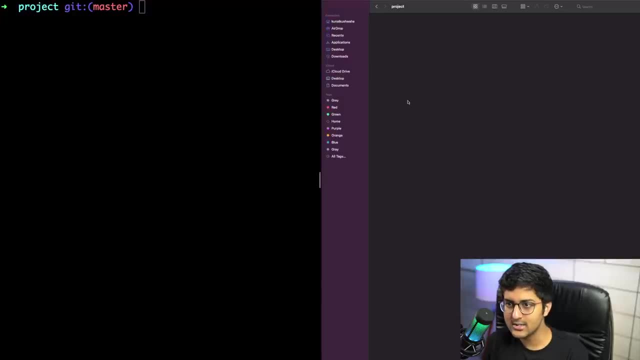 in my project folder. now you might be asking: hey, kunal, i can't see anything over here. how are you so sure that there's a git folder over here? as i mentioned before, you can do list. you will not be able to see it right now. it shows empty, but it is there. you can do an, a tag, a. 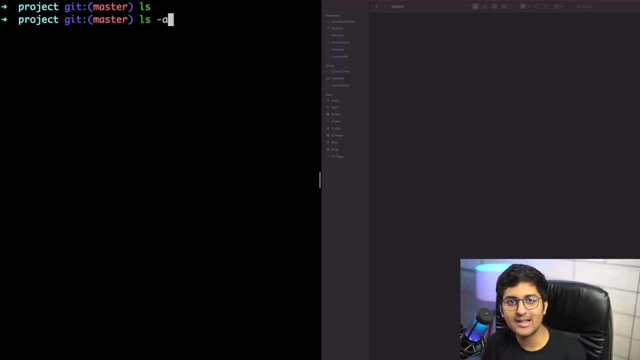 basically means show me all the hidden files. any file that starts with a dot is hidden in mac os and linux. so you can see dot git is here. you can also see what is inside this dot git folder. i can say a list, list what is inside the dot git folder. 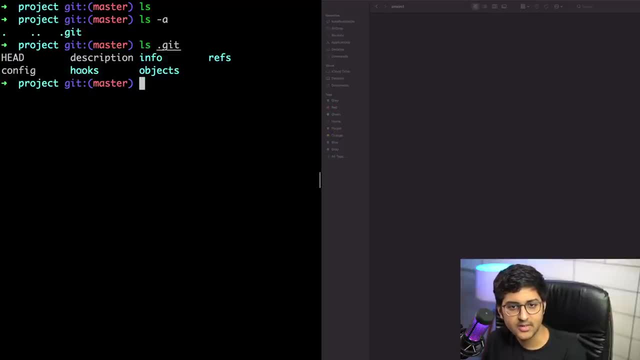 it contains something called head, something called objects, something called hooks, refs, config, description, whatever. don't worry about what these things represent right now- we'll be going through it shortly, okay- and don't worry about what this master is or whatever. so this is what we have. we. 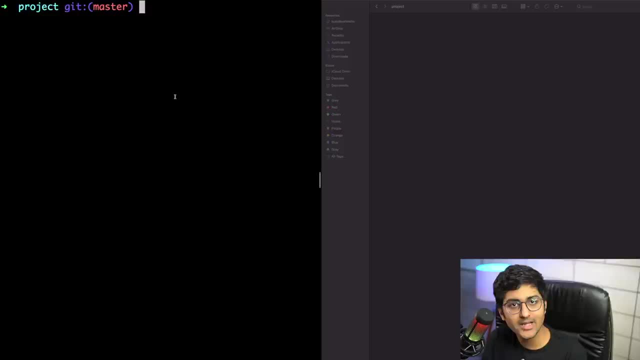 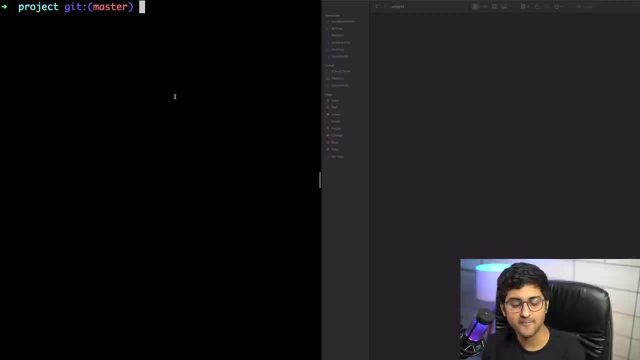 sure you click a photo of it so that other people are aware that you made this change. let's make a change. let's say currently. let's say i create a new file. to create a new file, another linux command is called touch. i can create touch names dot txt. so nametxt file is being created over here as you. 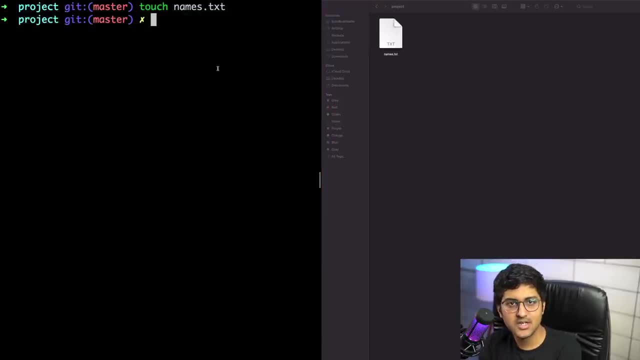 can see. has there been a change in my project? does anyone in the world know that kunal created a names dot txt file? is there a change my project? does anyone in the world know that kunal created a namestxt file? this history maintained in the git repository right now. is this history maintained anywhere? 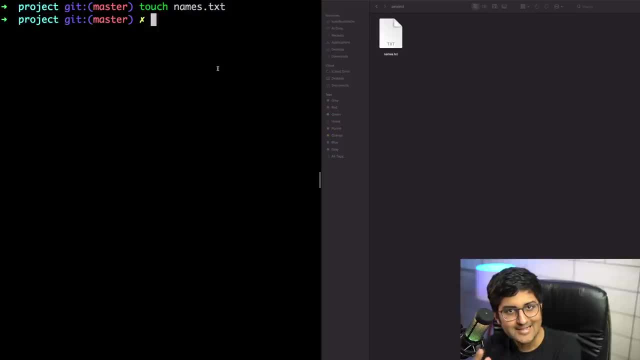 no, how do we see what all files have been changed or modified, or added or deleted? in short, how do we know what changes have been made in the project that are not currently saved in the history of that project? like no one knows, those changes are being made. a command for that is called git status. 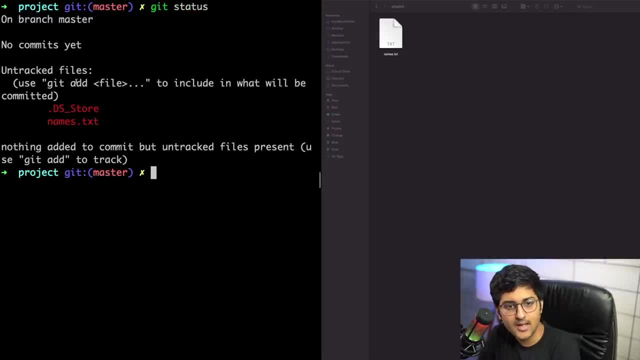 git status basically says: hey, you have these two files. this is some extra, you know, mac os file, don't worry about it, i can remove it. so here it's saying: hey, kunal, there's a namestxt file someone has added and it is currently untracked. means if you share this project with someone, like you know. 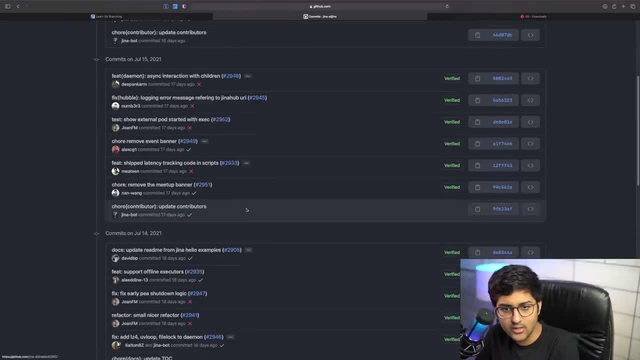 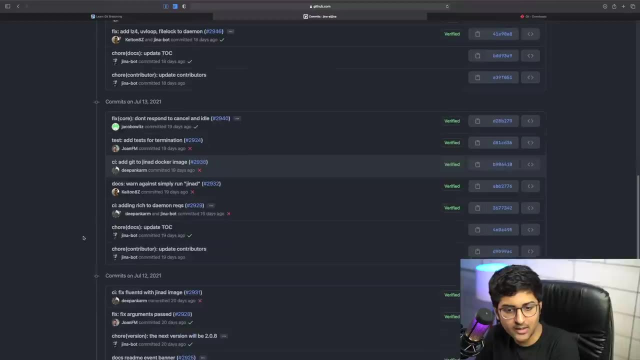 we have some projects shared over here. this is a gina project, so here you can see all the changes being made. let's say, some file rate change is being made, so here you can see all the changes removed or added or you know whatever. all of these are maintained over here. people know what. 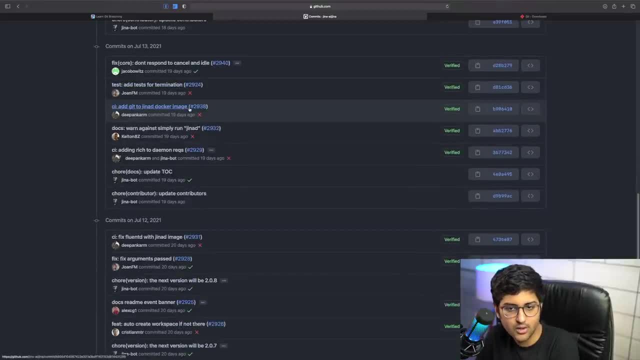 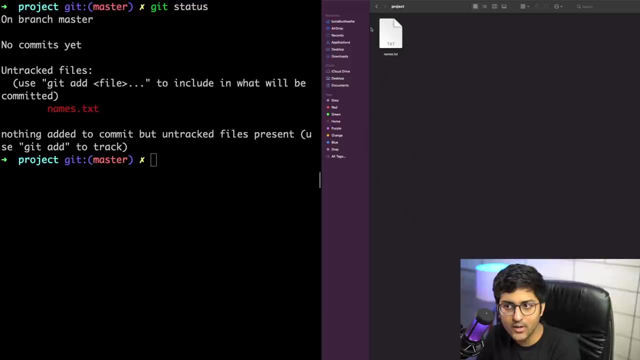 things were added like add test for termination, add git to docker image or whatever. currently, if i share this git repository on my github or this project folder on my github, no one knows. that namestxt file is added here by kunal on 1st august. no one knows that. okay, so that is basically. 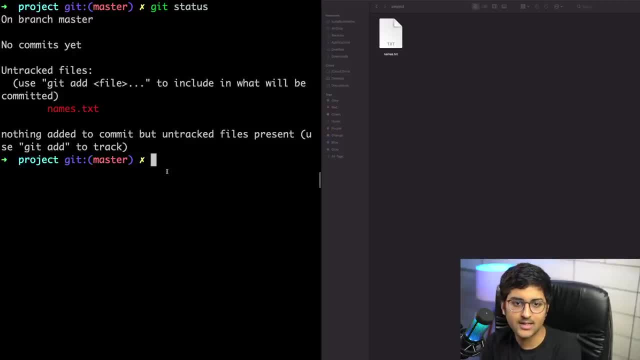 what we want to do. so this is the git status command that tells us that, hey, these are all the changes that are being made in the history of the project. so this is basically what we want to do. so this is the git status command that tells us that, hey, these are all the changes that are. 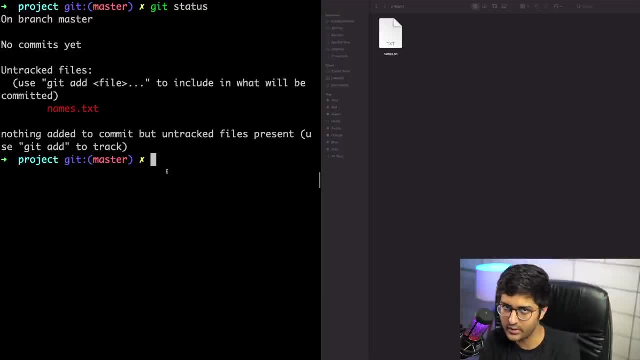 currently not in the history of your project. no one knows about it. okay, now we want to maintain these changes. we actually want these changes to be in our project's history. people should know that kunal created a commit that created a new file, or changed a new file or deleted a file. how? 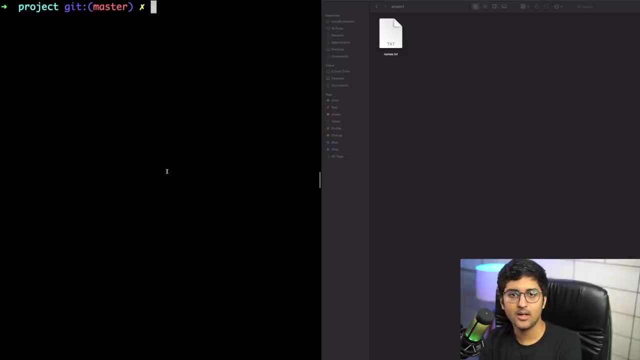 do we do that? we can do that very easily. um, imagine that you are at a wedding. okay, now, when you are at a wedding, let's compare this example to a wedding example. now, when you are at a wedding, you, the, you know the, the couple, they are on the on the stage and people, uh, people, take their. 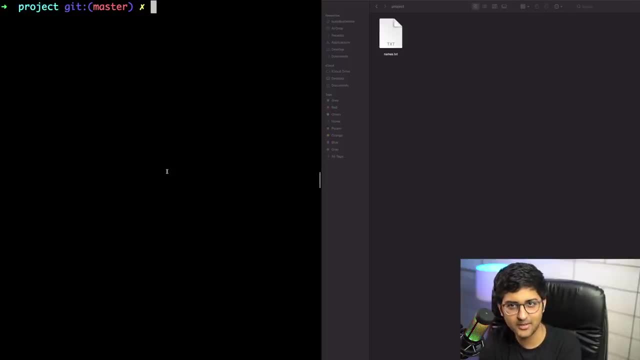 photographs, like all the guests, to take their photographs with the couple. so how does that entire scenario play out? the guests, they will go on to the stage. that's the number one step. the photographer will then take the picture of the people, or let's? let's give it a bit more detail. 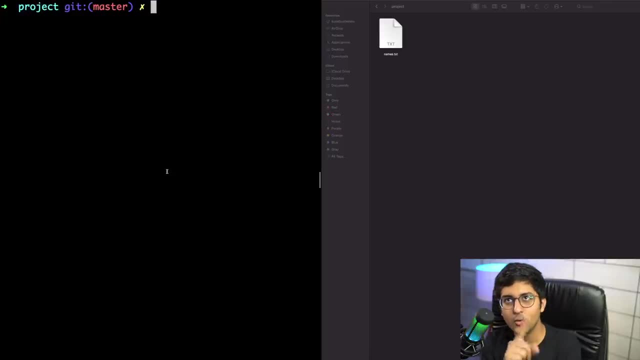 the couple's first step is going to be the couples whose photograph has not been taken. they will go on the stage, okay, then the photographer will click their picture and then they will exit the stage and now their picture will be stay, will be saved in the history of that. 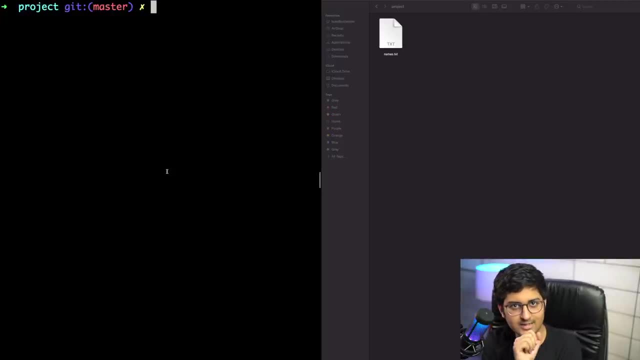 wedding in a photo album. this scenario makes sense: couples who sorry, guests whose photo has not been taken. they will go on to the stage, photographer will click the picture, they will come out of the stage and their photo will be permanently saved in the history of the wedding in a photo album in the 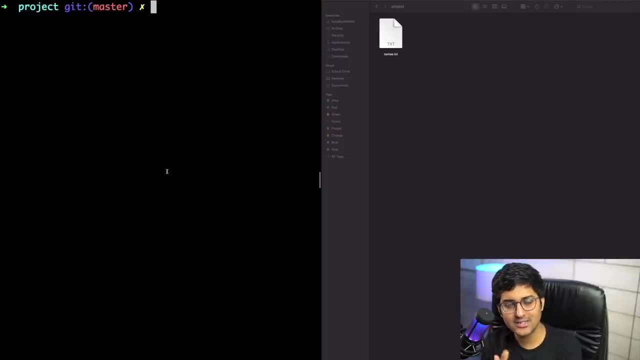 second step is about how does git relate the guests whose photo has not been taken yet. they are known as this thing: untracked files. okay, what is the next step? we need to take a photo of these files so that we can save it in our git repository, or the git history, which is known as the photo album in this example. okay, 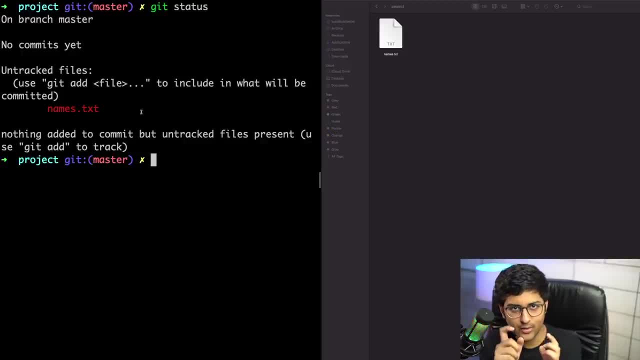 only step that is remaining is placing all these files whose photo has not been taken yet, means whose history is not being saved in the project yet, onto the stage. how do we do that? there's a command for that called git add. you can either do dot. dot means everything in the current directory. 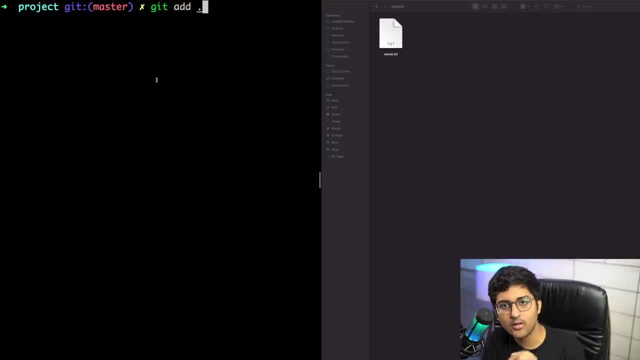 everything in the current project directory that is currently not having its history or that is untracked means all the red files that you saw previously. put all these files in the staging area on the stage, basically so that a photo of them can be taken. you can also write individual names of the file. let's say you have a few files. 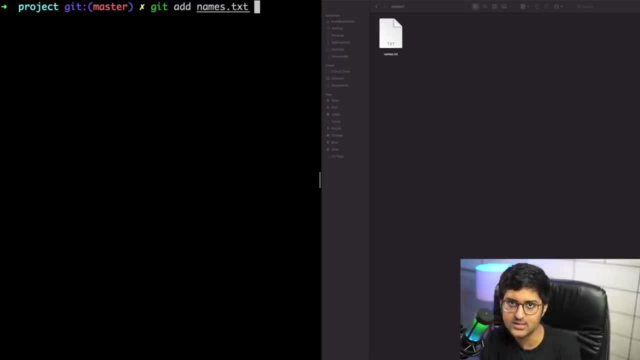 that you changed, but you only want to maintain the history of a few files, not all the files. you can also individually add the names. now, if i do git status again, you can see it's now changed to green. it means that these people whose photo has not been taken, or some changes. 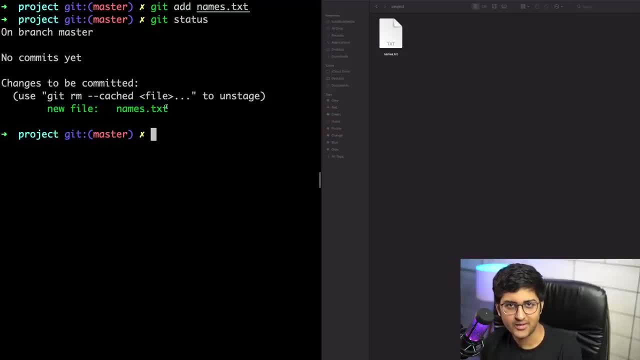 have been made. let's say, they got some new outfit or whatever and they want to take get their picture clicked again. sometimes that happens. so in that case, um, these people are now on the stage and we can now click their picture. so now i'll be like, hey, photographer. 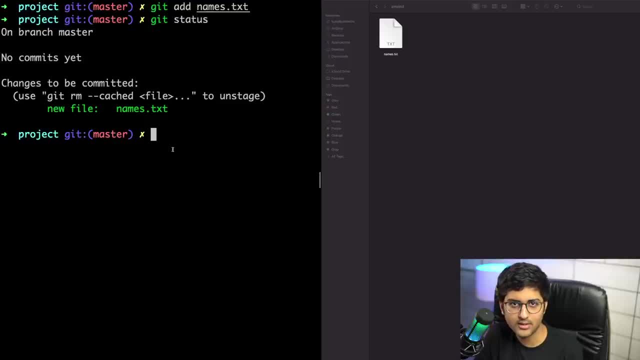 please click their picture so they are permanently saved in the photo album or the git history, like this, like this: how do we do that? there's another command for that git: commit dash m. dash m basically means message, provide a message. message i can provide is something like anything you like i can say. 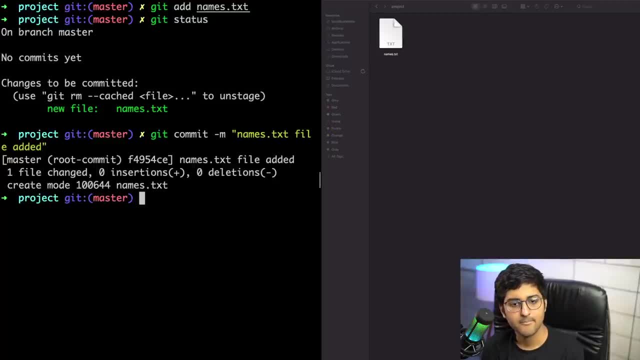 namestxt file added. now, don't worry about all these things. what is master? what is this thing? what is this thing currently? this is very simple. one file changed: zero insertions of lines of code, zero deletions of lines of code. that is true. i did not make any. 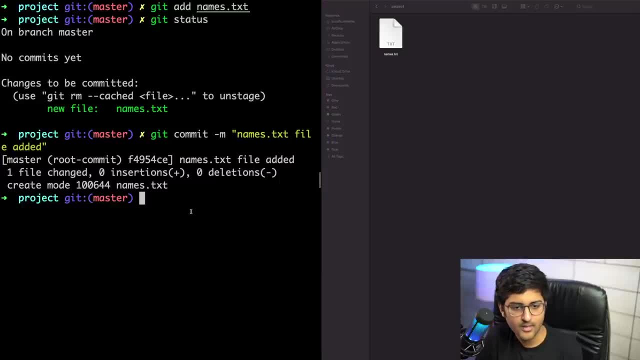 insertions of code. all i did was create a file. that is true, okay. so now, if i do git status again, now it's going to say: hey, are there any more people whose photograph has not been clicked yet? you tell me, tell it to yourself. if you said no, then you are right. 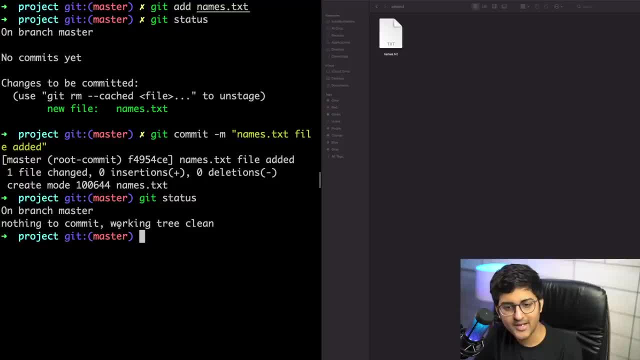 nothing to commit working tree clean since i took the last photograph. was there any other change made in this project folder? no, there wasn't. that is why it's saying no, no other new person is there whose photo needs to be clicked. i hope that makes sense. now another 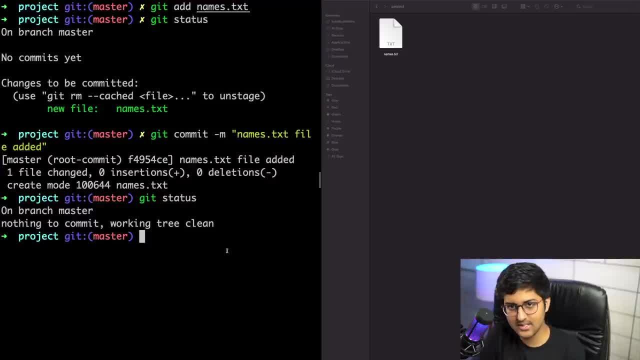 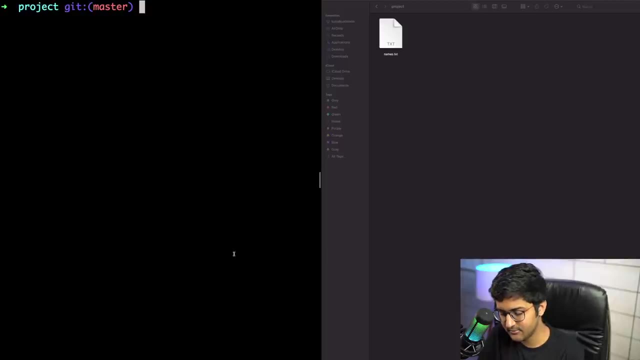 question you may have is: so these are the basic commands: git init initializes the repository, git add git status and git commit. as simple as it gets. now you might be wondering: hey, let's make some other change, let's say i add something in this file, so i'll go in my vim. i'll add: 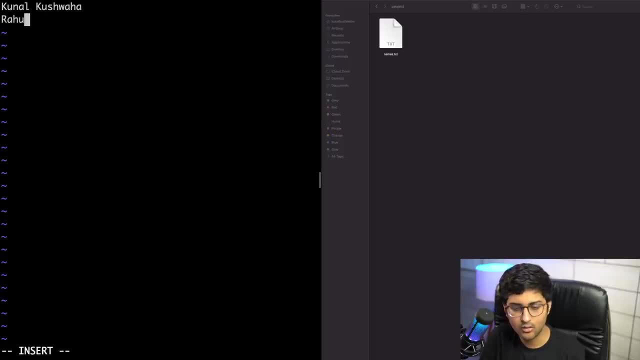 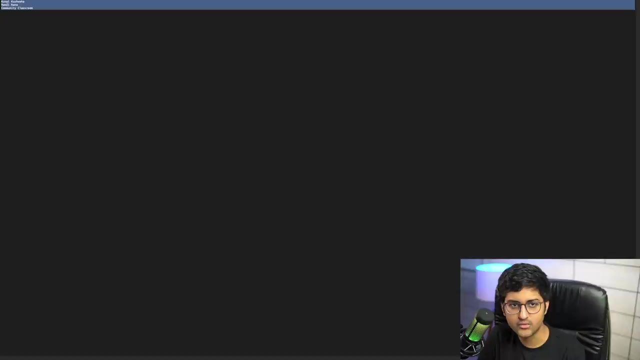 kunal kushfaha, and i'll add rahul rana and i'll add, let's say, community classroom or whatever. i have made changes in this file. you can also double click it and see. if i double click it, i can see rahul rana, kunal kushfaha, community classroom is. 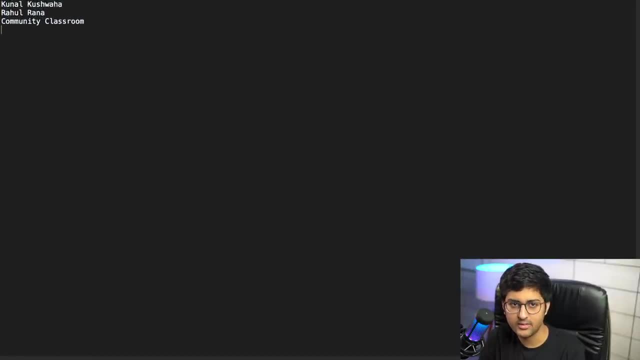 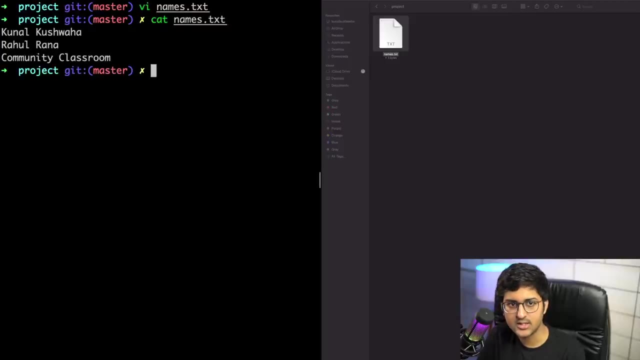 in this file. so you can see here it is available. okay, there's also another command for this. there's the cat namestxt. it basically displays whatever things are available in the namestxt file. okay, three lines are available, since i took the last picture or made the last commit. 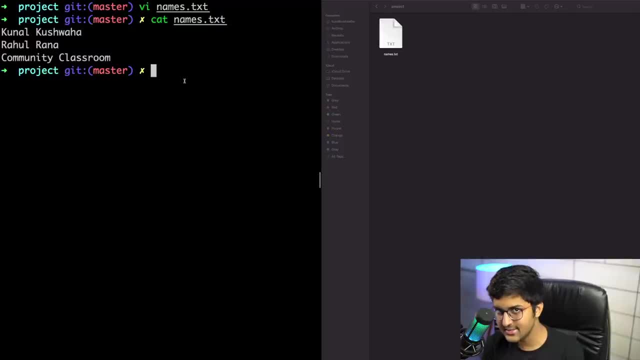 have there been any changes in this folder structure? yes, namestxt file has been modified. how do i know that git status modified so you can say you modified namestxt- cool again. let's take a picture of this. let's get all these people who have been modified on the stage. 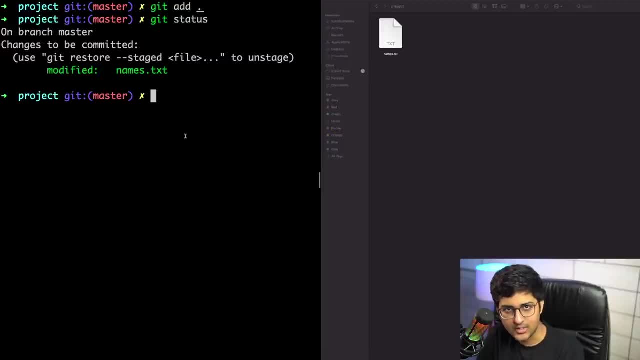 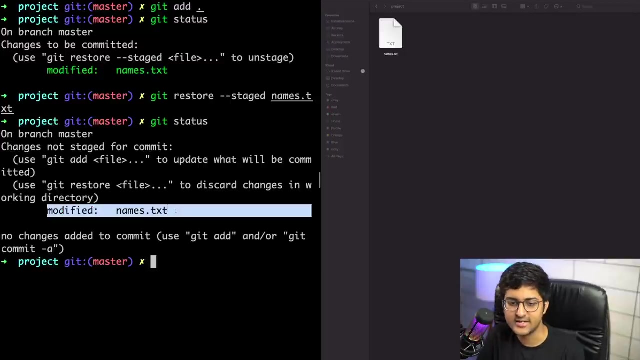 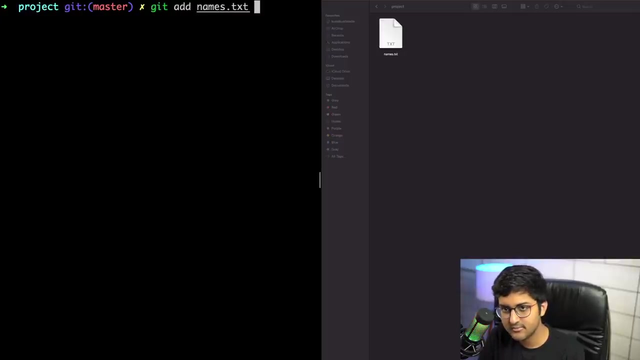 get add dot. get status. it basically says hey, so you can do git restore dash dash staged names dot. txt. they are now again outside the stage. you can see the red fold, red thing. okay, let's say we want to git add namestxt. you can see they are now on the stage. i can take a picture. 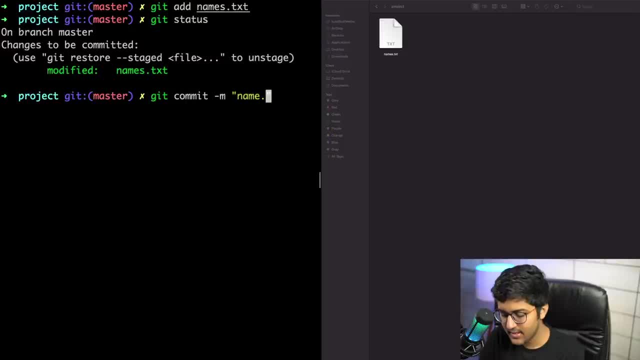 i can say names: dot. txt. file modified. now it's saying one file changed. three insertions were made. that is true. i added, i added three lines over here. that is true. another question you may have is: hey, kunal, where can you see this entire history of the project, all the commits that were? 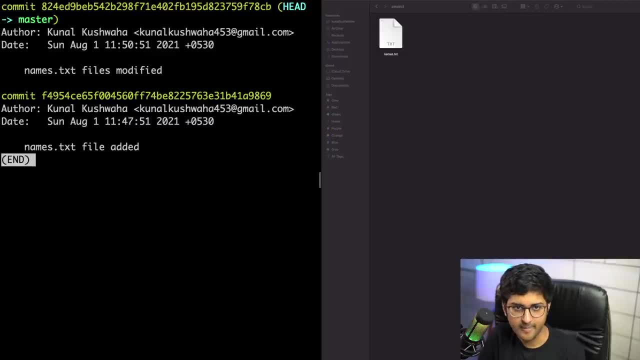 made in the history git log. so currently we only have two commits. kunal kushwaha. you can see that we have made three insertions over here. that is true. i added three lines over. made a commit on 1st august at 11 am. namestxt file was added. kunal kushwaha again made a commit. 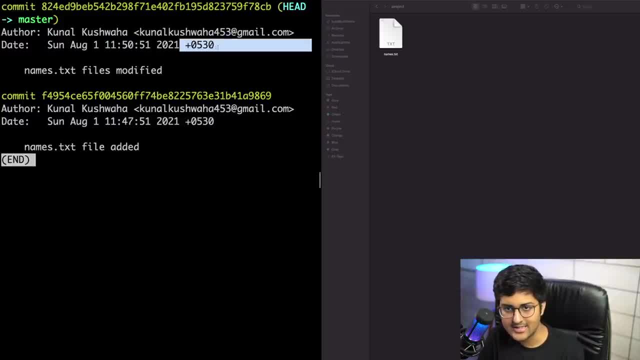 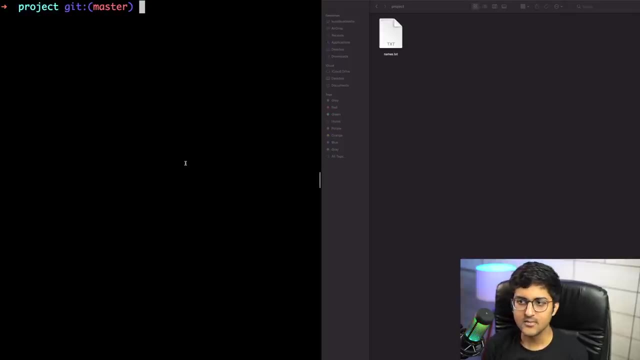 on 1st august, sunday, 11: 50 ist time zone plus plus 5: 30 is ist time zone and namestxt file was modified. i hope that makes sense and that was pretty much about it. okay, those are the basics of it. let's make a few more commits. don't worry about what the master is. 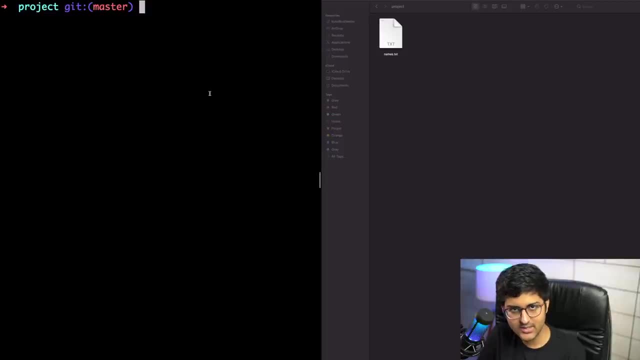 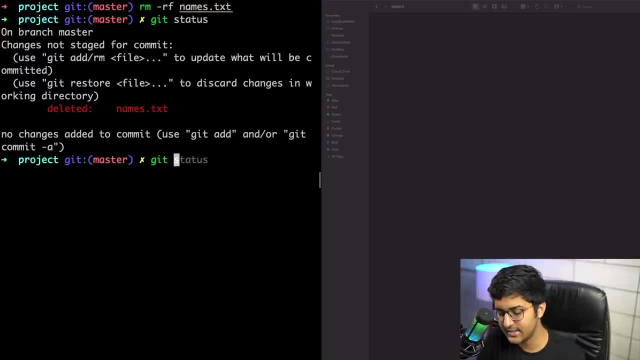 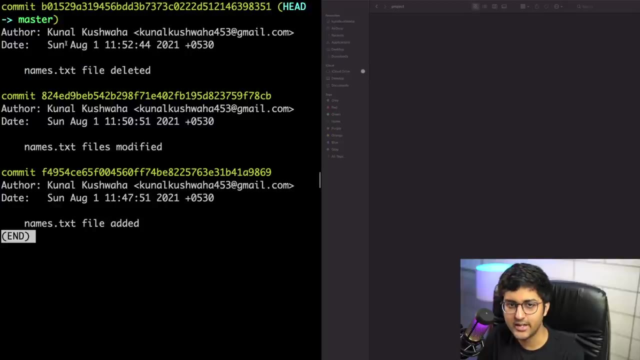 file has been deleted. so i'm going to be like: okay, uh, let me add this git. add namestxt. or dot git commit minus m: namestxt file deleted. that's it git log. you can see namestxt file was deleted on first august this time. imagine you did this by mistake. imagine you were like, hey, i did this. 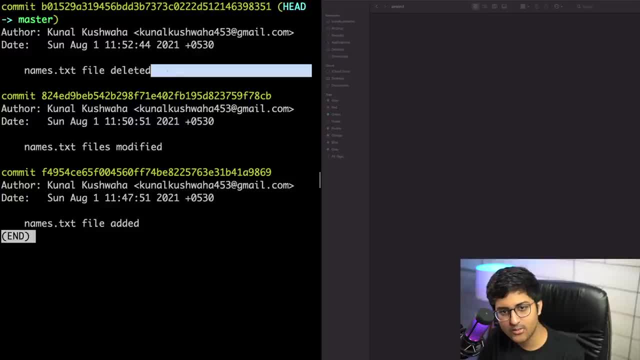 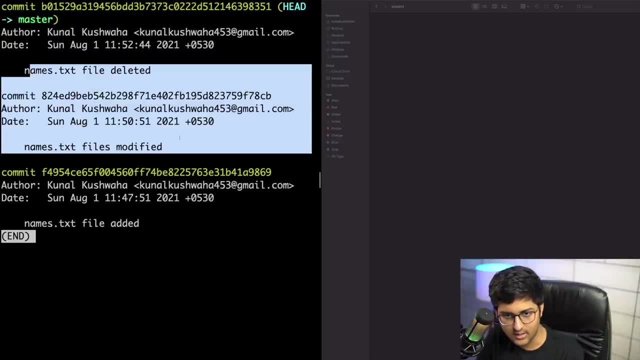 by mistake. i did not want to do it. all i need is i basically want to remove this commit from my history of the project. so if you want to remove this commit or all the you know this commit or like these commits, you cannot like remove just this particular one commit from middle, because 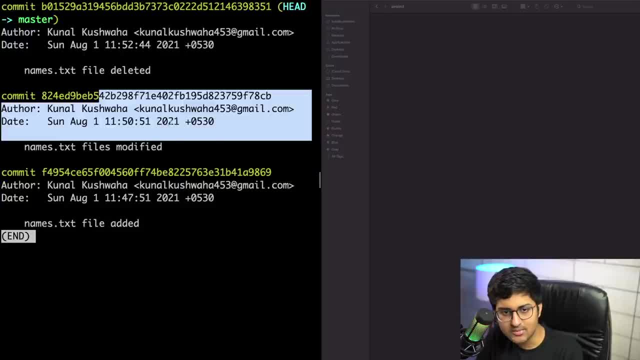 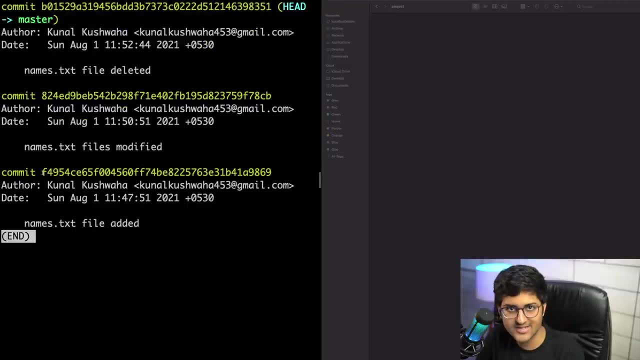 as you can see, each commit has a hash id, so each commit is built on top of each other. you can unstage these commits. let's say you want to go back to, you know the previous example that we were giving. let's say you want to go back to any particular history of the project. let's say you want your. 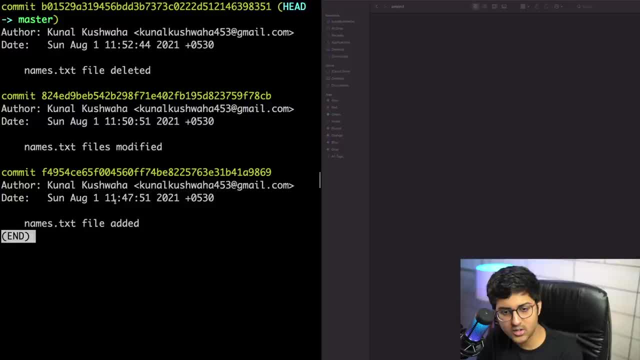 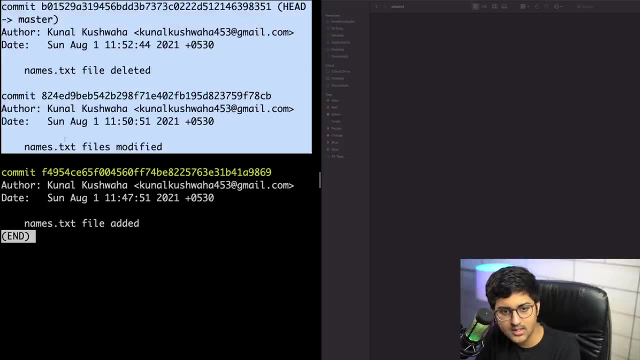 project to be what it was like on sunday, 1st august 11: 47 am. means this: this particular commit. i will just copy this thing, okay, if you want to remove these commits, just copy the commit just below it. so if i want to remove these commits, i will copy this thing. okay, i hope that makes sense. 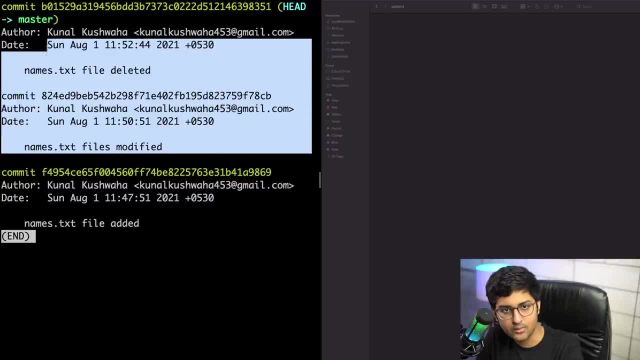 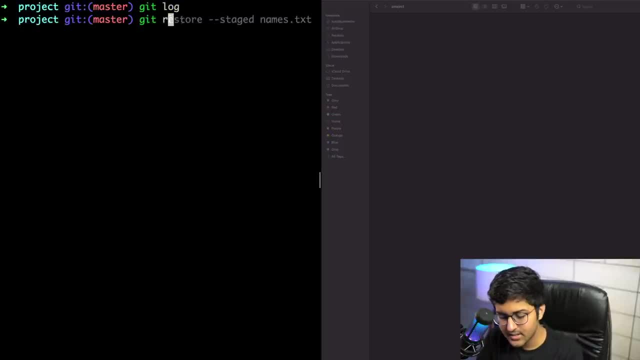 i copy this now. whatever i am about to do, it will remove these commits. whatever commit, i copy all the commits above- it will be removed. let's see how git reset paste. if i do git log, i will only be able to see one commit. only one commit is here, the first one. that is what we wanted. 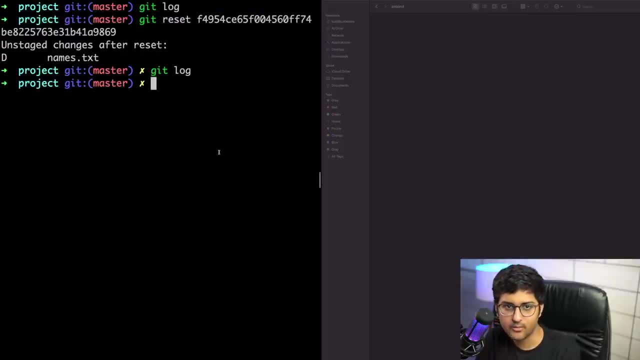 now you might be like: hey, what happened to all the files that were modified or changed or whatever in the previous commits? they are now in the unstaged area. this basically means that the people whose photograph was taken, their photograph has been, like you know, deleted and now they are again in the section of people. 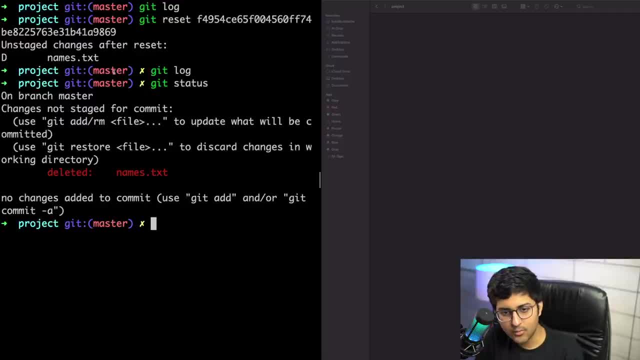 whose photograph has not yet been taken. now, what we, what we can do is: let's say, we deleted this thing by mistake, or whatever changes we made in these commits were by mistake. then what we can do, we can just restore this, or we can, um, we can also put it in the staging area, in the stash area for 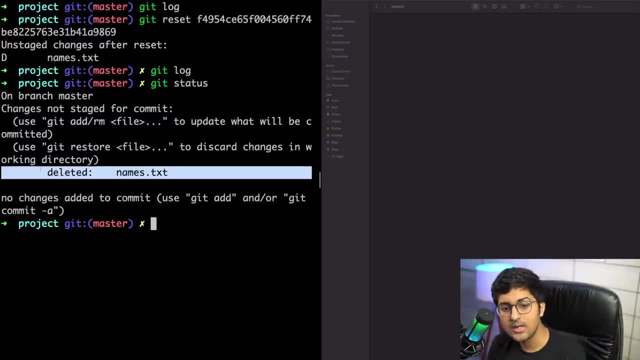 example. imagine you don't want to, you don't want to delete these changes right now. imagine you just want to say that, hey, you are a few people whose photo has not yet been taken. go to the backstage, and whenever we want you to come back, we will get you back. how can i explain this more simply? let's. 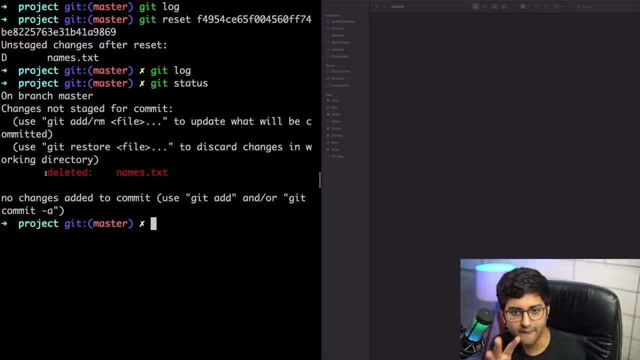 say, you are working on a project and you are working on a particular feature and you have a few, few lines of code that you are working on. now you want to try out something new with a clean code base. okay, all the changes that you have been made that are work in progress files you have. 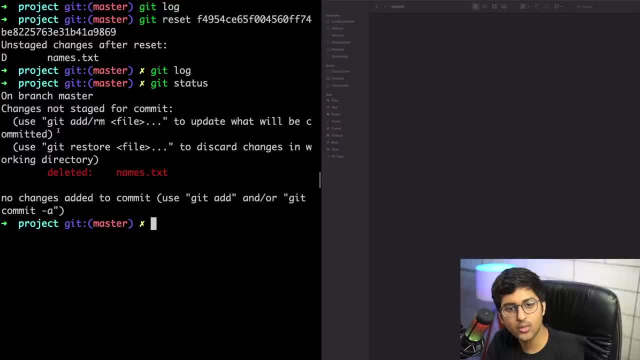 been modified. you want to remove those, but you also don't want to save your progress as a separate commit. you basically want: hey, i wish there was a way where i could just put all my work somewhere else without making a commit, without making a history in the project, and whenever i want that. 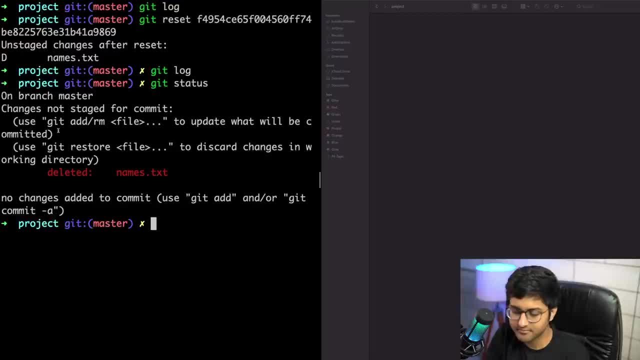 thing back, can get that back whenever i want. command for that is called get stash. so basically get the people you want to be on the backstage first on the stage. so it says this file was deleted. this is a change. now i'm going to get stashed this. i'm going to say, hey, go back to the staging, like one. 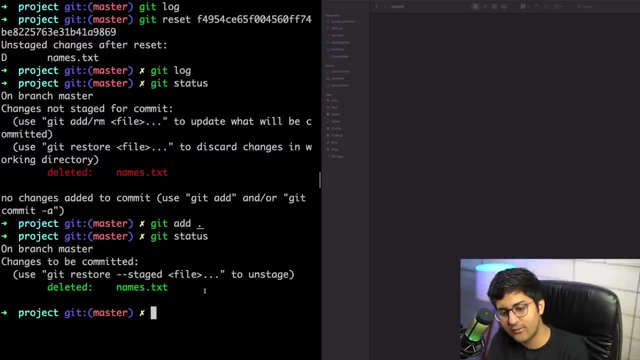 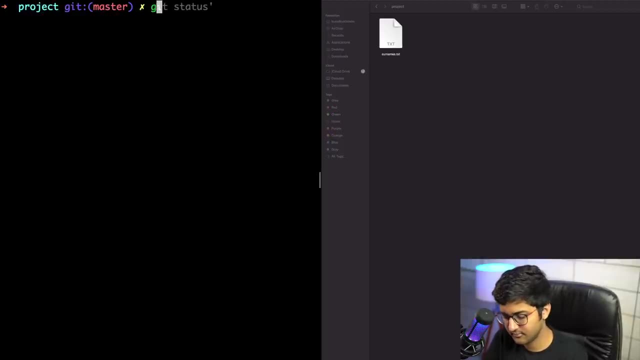 go into the backstage whenever i want you all the changes, whenever i want all these changes being made, i will bring you back. for example, i can make another change. let's say touch surnamestxt. i can say git add dot git status. i can say: you know um surnames dot uh namestxt. this one is saying that uh, namestxt has been. 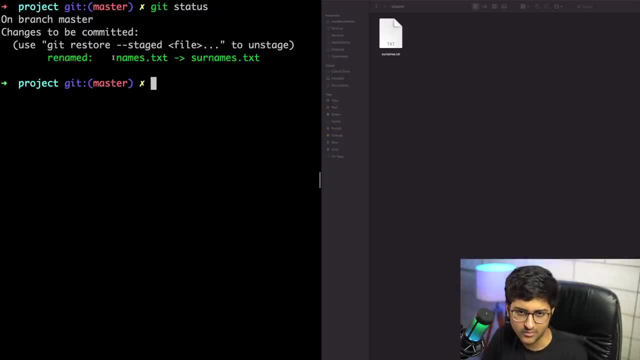 modified to surnamestxt like renamed, so it's a, you know, pretty smart in that way. but uh, what we can do is let's say, let's say let's try to make a few changes now. so vim, surnamestxt, i can say insert kushwaha. okay, let's create another file, let's create houses dot txt. 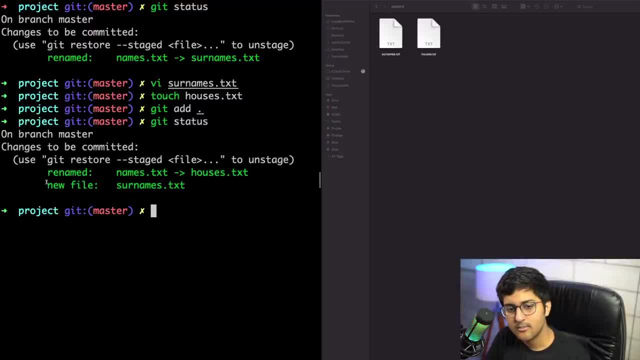 git. add dot. git status. bunch of things i have done. bunch of things i have done. now what i want is like, hey, all these changes i have made, i don't want to commit it. i also don't want to lose these changes. i basically want you to go backstage and whenever i want you, i will bring you back. 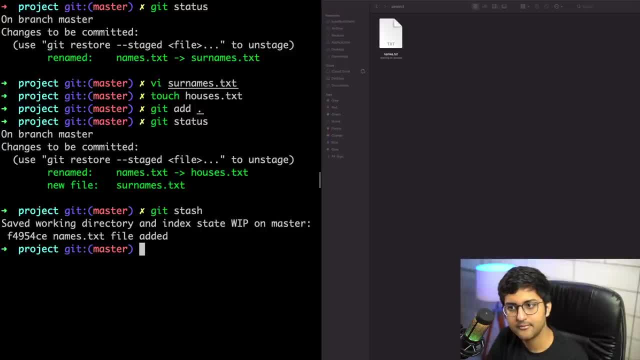 you can do git stash for that git status clean. now my project folder is exactly like it was on august 1st 11, 47 am. exactly like it was. that was my first commit, and my first commit only consisted of what the namestxt empty file empty make sense. that's how you can go back in the project. now let's say: 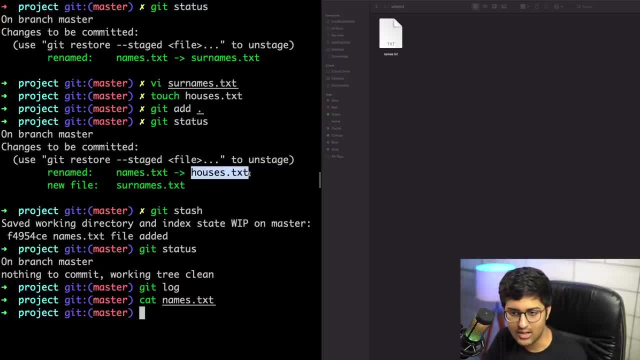 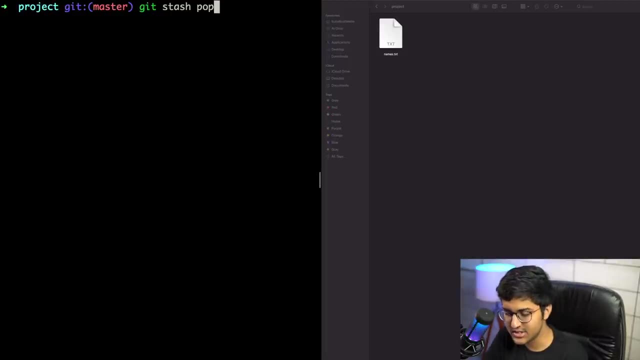 all of these changes that you made, like rename the namestxt file to housestxt or whatever, created a new file like surnamestxt or whatever. you know how can we do that? git stash pop. hey, all the people who are in the backstage come back to the staging area. 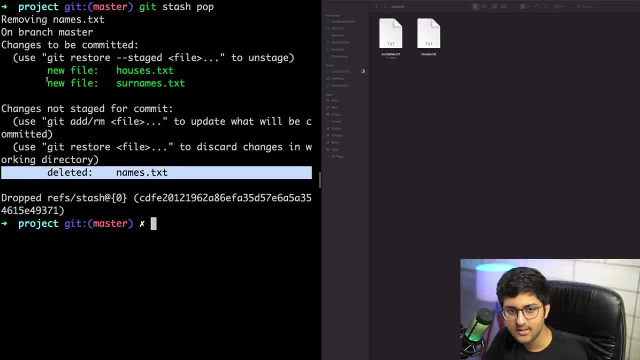 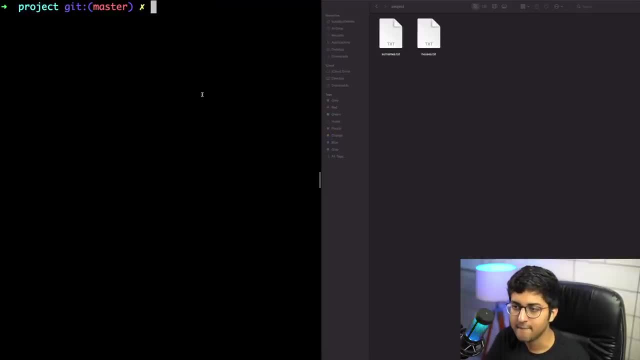 in the unstaged area. so you can see, here we have all the changes that were made previously. cool, all right. so i don't want these changes. let's say i can just say get add and get stash again. now let's say they are in this, you know that backstage and we can just say, hey. 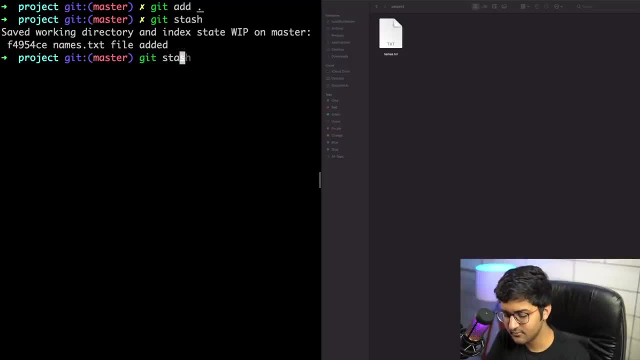 your photo is not being taken. go go away. git stash clean. sorry, not clean clear. so those changes that we made here would be were doing versionИ. i thought you wanted them out, but actually I didn't want to create that. but if I want toOLLe then i'm gonna interrupt that at this point. 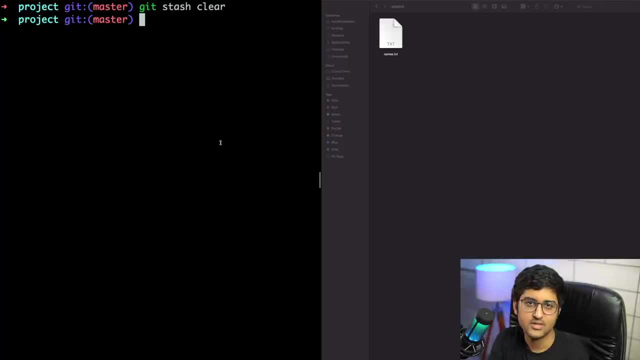 pullingagen, then doing Rayaji. so I'll include these changes andJam captured these changes all the time. so were made that were like not committed and in the you know separate structure. they are now gone. you cannot get those back. they're gone now. okay, cool. so that was about how you can go back to your 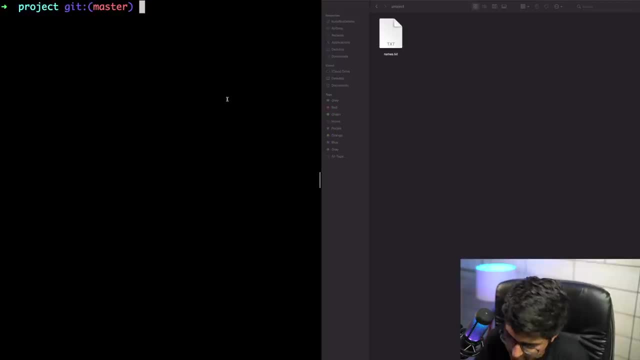 comments. let's move forward to learning about github now. so what we are going to do now is there are two ways, like two things we are going to do. first, hosting our own project on github. let's say you have your personal projects or local projects or whatever, and you want to push those. 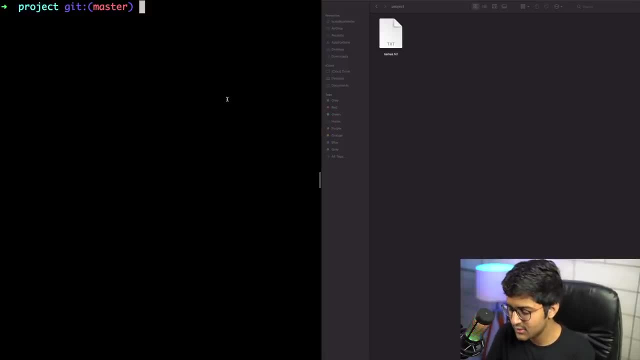 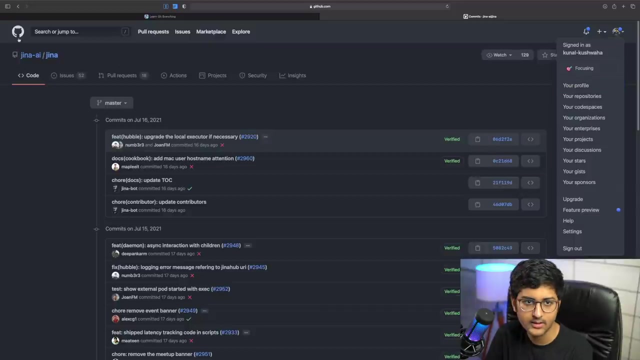 on github. you want to share it with other people, so how do we do that? let's see. so let me go to githubcom. let me open up my. let's go to github. we are here at github. let me go to my personal profile or like the dashboard or whatever. we can create a new repository. i can just click, say create. 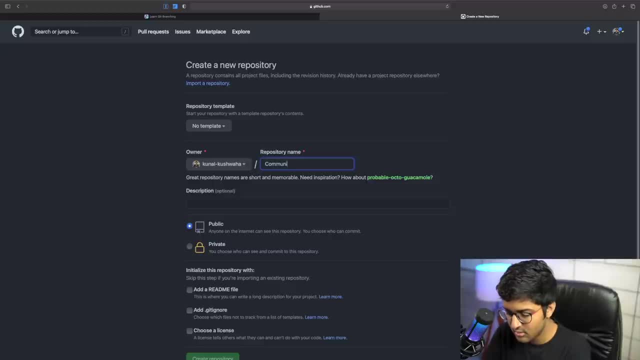 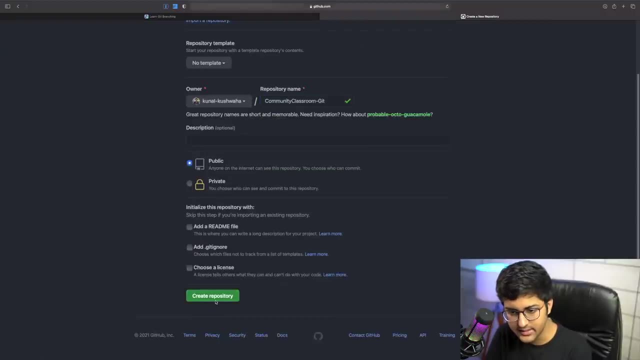 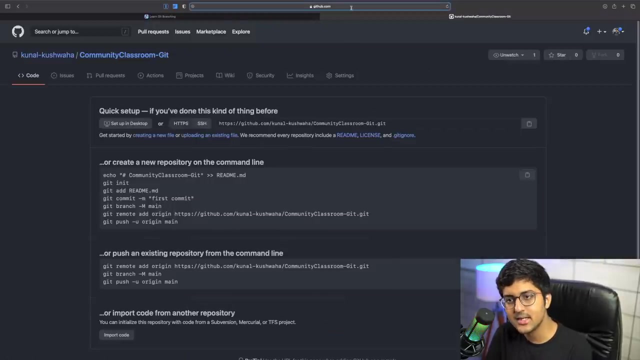 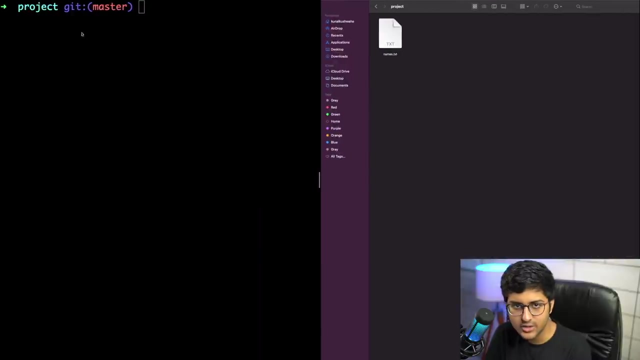 a new project. i can say community classroom git or whatever. i can create this repository. i can set it as public and create the repository now. basically, this is the url for my repository, kunal kushwaha- community classroom git, and we want this url to be attached to my project, the local project. a command for that is git remote. 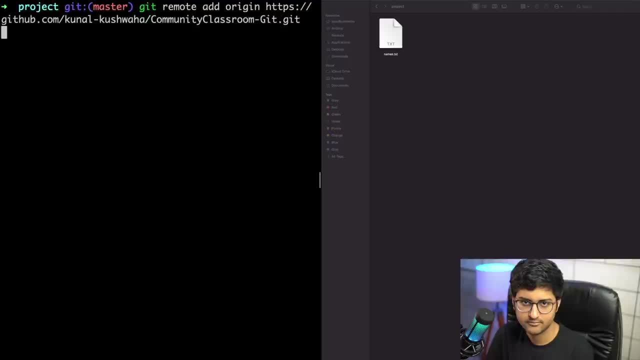 app: add origin url. i did a lot of things over here, so git is just the git command. remote basically means you are working with urls. add basically means you are adding a new url. origin basically means what is the name of the url going to be that you are going to add. it's like phone numbers. you. 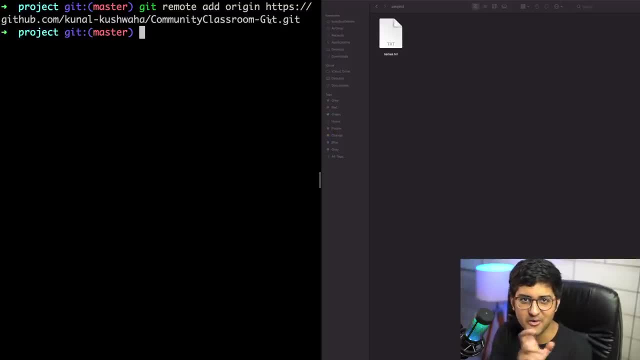 don't remember all the phone numbers. in your contact list you save a phone number with the name of the person. similarly, the name of this url is origin. by convention, this can be anything you can do, but by convention, all the repositories and folders that start that basically are in your 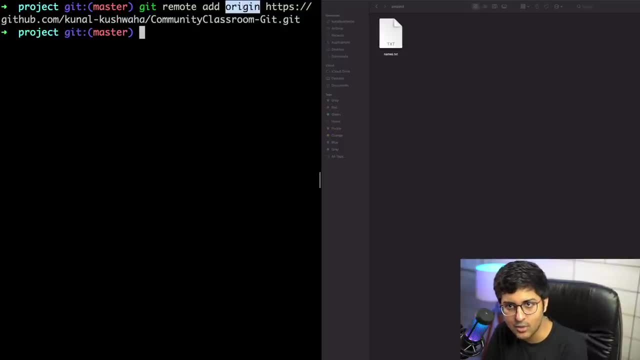 personal account. on your own account, they have a name called origin. if i say git remote minus v, this will basically show me all the urls that are attached to this folder. this is attached. these are the same one: fetch and push. we'll look more into what fresh is. what fresh is what fetch is. 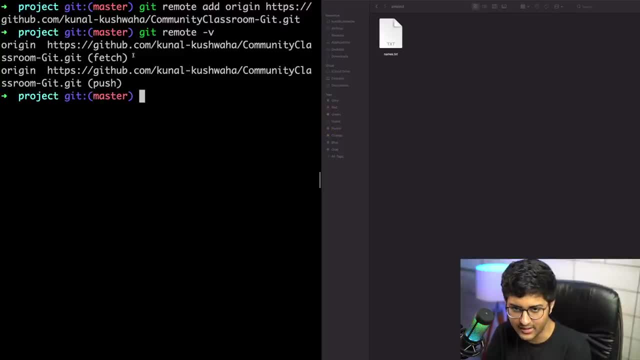 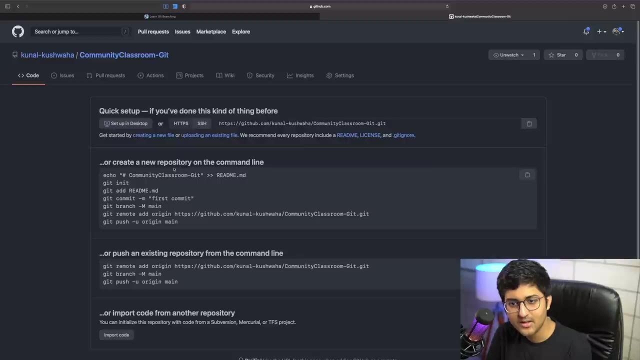 push is and we'll look more into like what is master and head and everything. don't worry about that. so now our thing is connected. this url is connected with this particular folder. now, if i refresh this, can i actually see the namestxt file here? let me refresh this. no, we can't, because i have 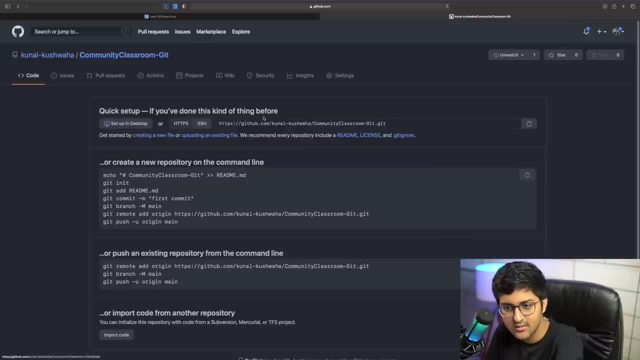 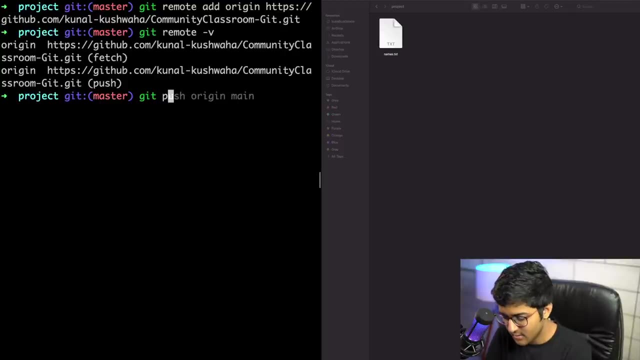 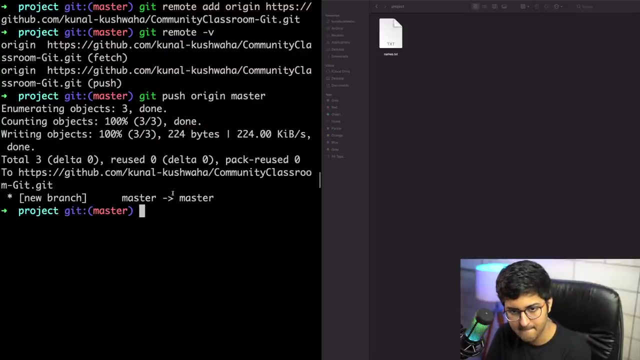 not shared the changes on this url. a command for that is git push. here you can see push. push means changes to which url do you want to push origin and which branch do you want to push? we'll look more into what branches are master, but now imagine it's master now, if i refresh this. 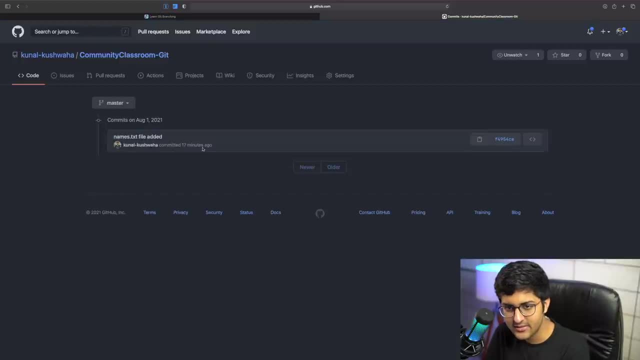 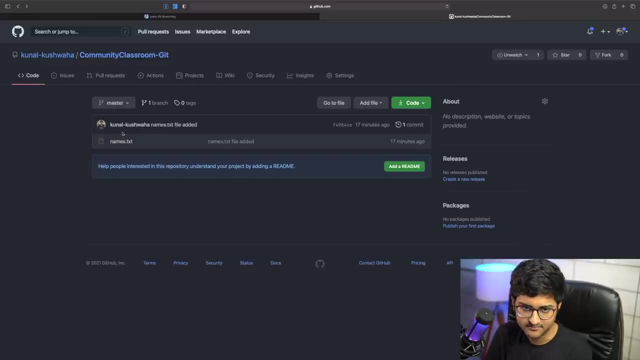 namestxt file is here. commit is also here. 17 minutes ago, namestxt file was added. this is the commit message that i sent. what do we mean by branches? you can see master is here. currently. it's known as main because of the naming convention, inclusive naming convention. 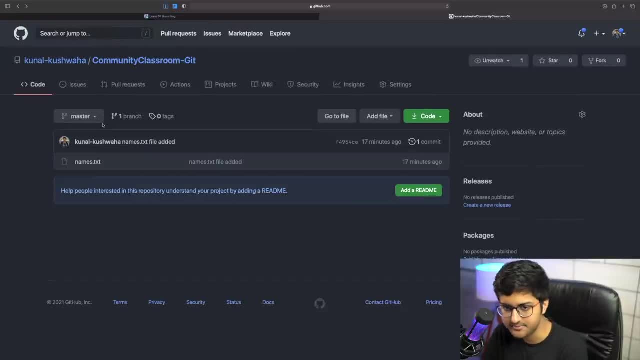 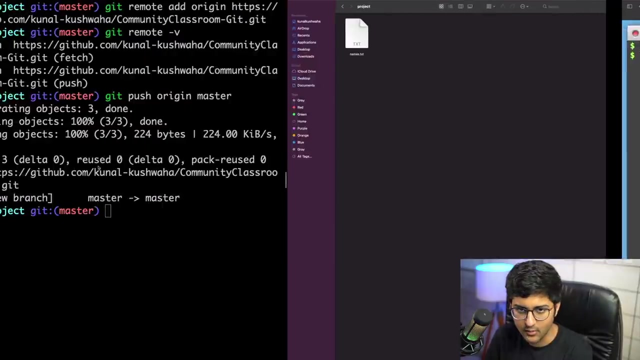 so it's most probably going to say main whenever you get started. my client is like a little old so i don't think it was updated, but uh, previously it was known as master. what is this master? what is branching? let's look into it. so what are branches? imagine you are making commits, like we. 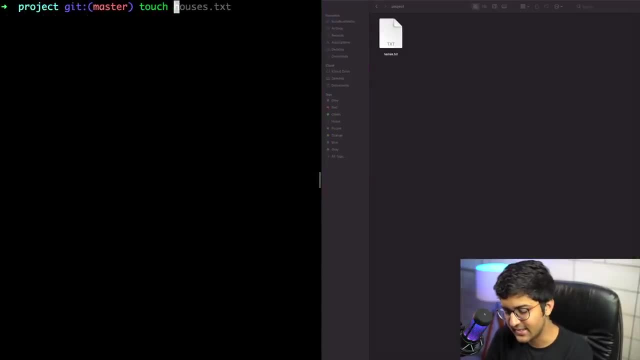 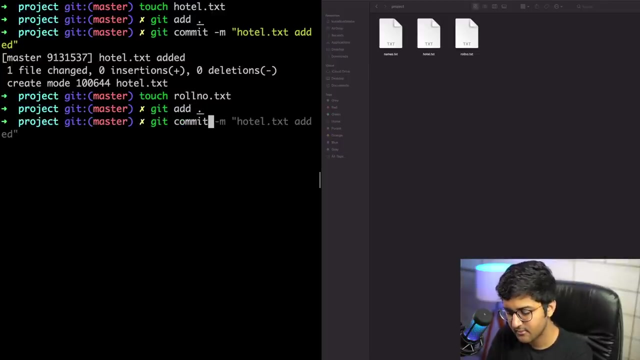 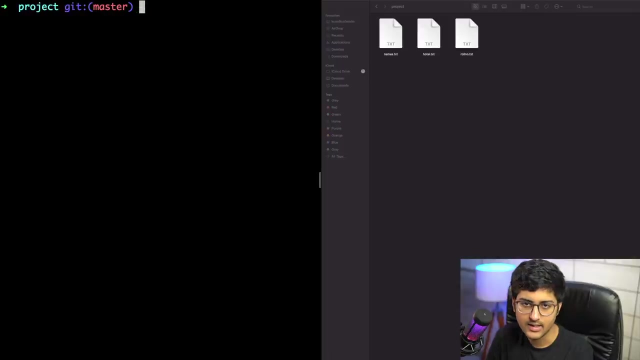 were doing so let's make a few more. you know random commits. let's say i create a new file- hoteltxt. i can create a commit like this: git commit- hoteltxt added. roll number, dot txt. roll number added. let's create one more. i can say i can create another file, or i can 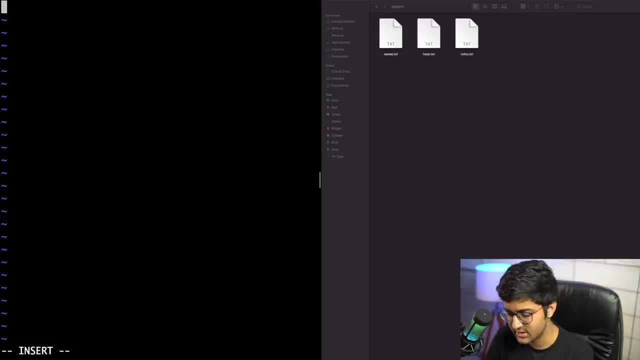 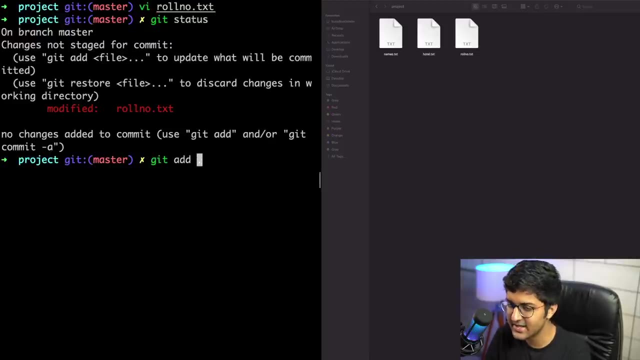 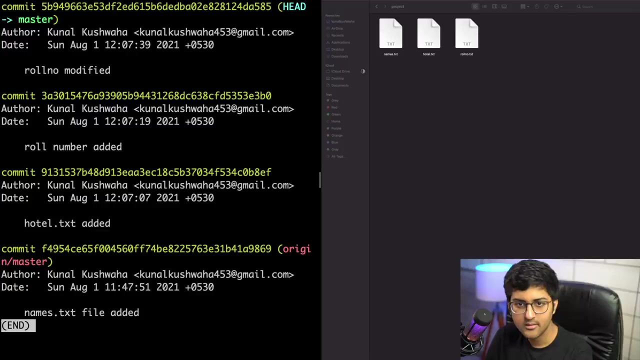 just make some changes in some file. i can say: add some changes here. some like this get status. so don't worry if i'm doing it so fast, because i'm just adding random commits. nothing is to be explained over here. role number modified, so many commits being made. 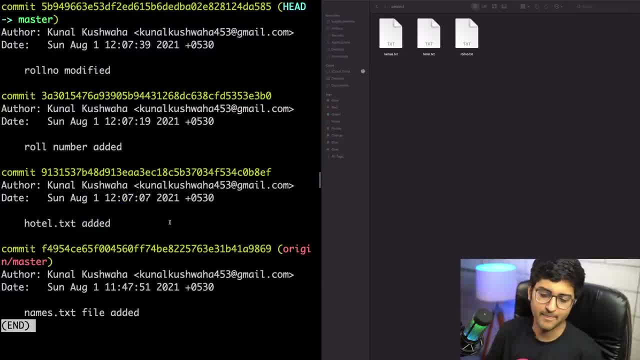 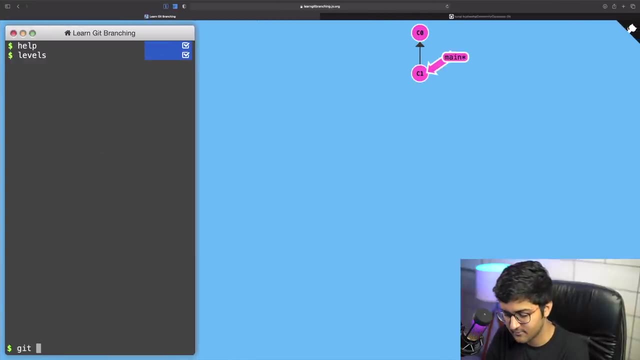 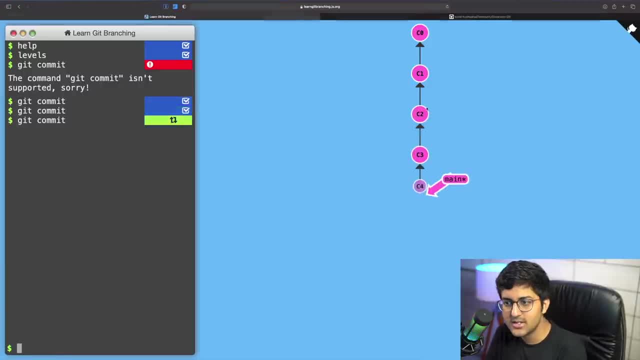 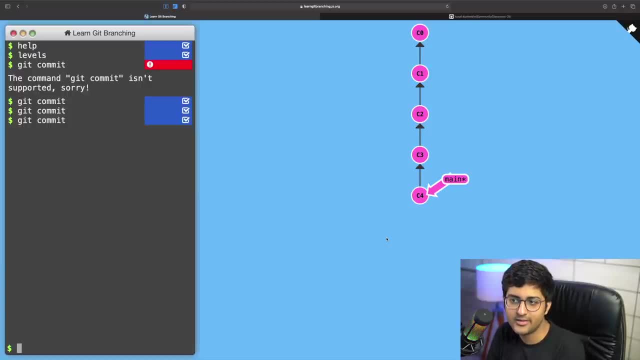 now internally. if you have heard about it, this is a directed acyclic graph. don't worry, we will cover that in detail in the dsa boot camp. but uh, as you can see, as simple as it gets, this does look like a branch and by default the name of this branch is called main. previously it was known as master. 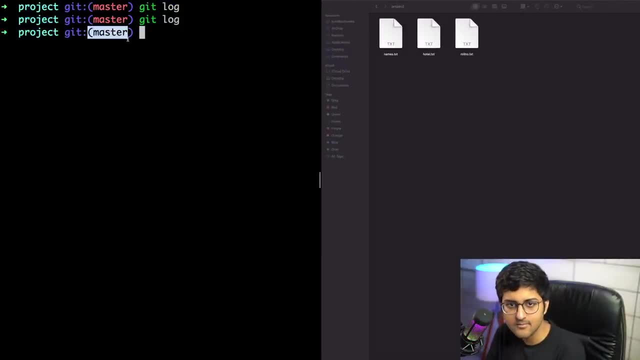 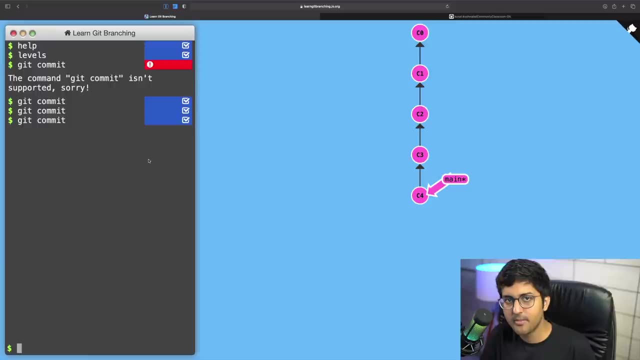 that is what this master thing represents. okay, so these are what are known as branches. now your question might be: hey, kunal, what is the use of a branch? why are we having branches? the use of it is that, in short, whenever you're working on some other feature or new feature, or resolving a bug or whatever, always create a separate branch. 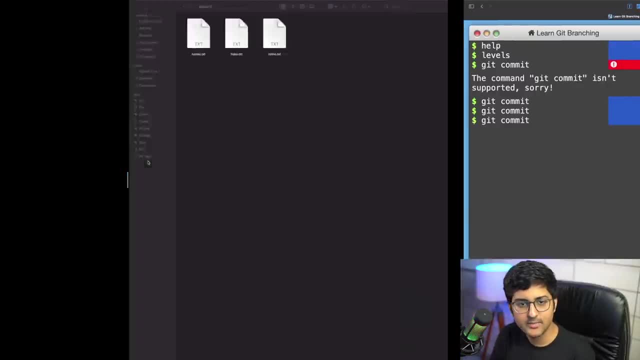 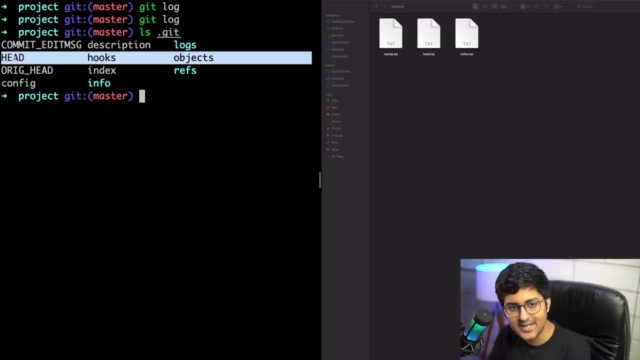 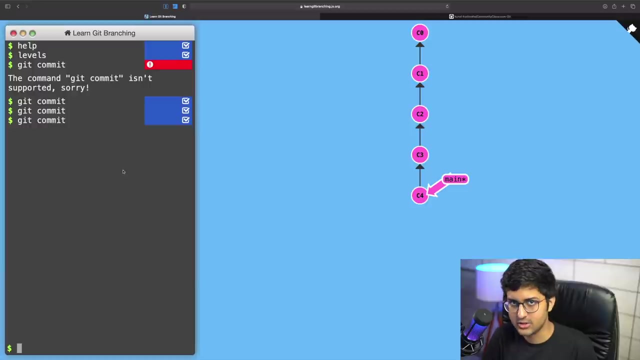 reason for that will be shared later in this video. what all things are remaining that i did not cover. what is this head, this head thing? so in branches what happens is that, uh, you should never comment on the main branch or the master branch. your your main branch, because in open source project, let's say, if i say react. 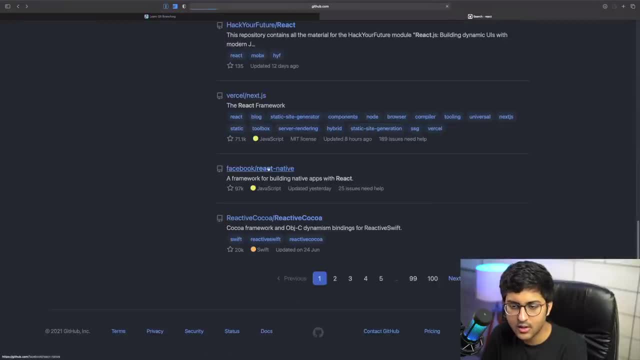 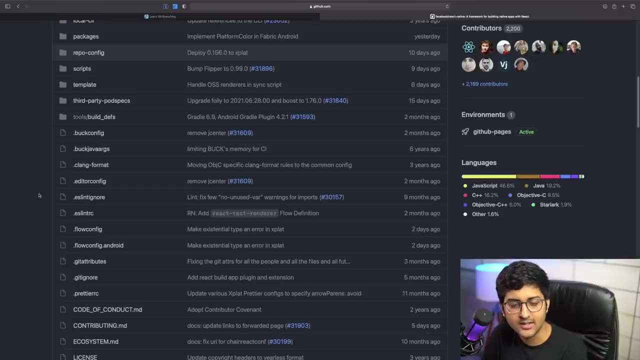 there is the react folder, facebook react or react native, whatever. so you can see this is the main branch. this is the code that is actually being used in the project by hand right now. delicious a used by people like the, like the users and developers. imagine that you know there might. 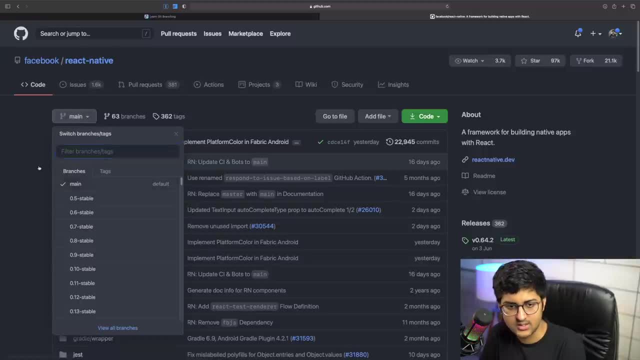 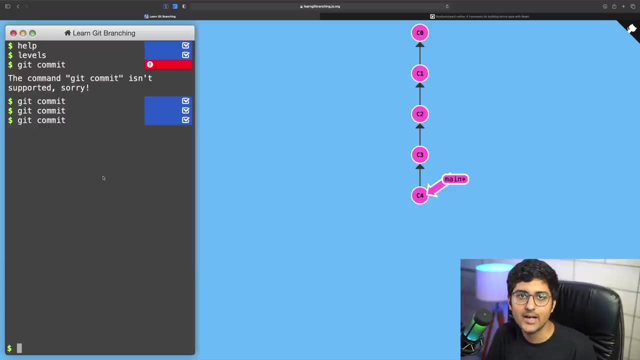 be so many other branches, but the main branch is the default branch. this is the one that is being used by people. so that is the reason we never commit directly on this, because our code that is not finalized yet might contain some errors. that is why all the code that is not finalized 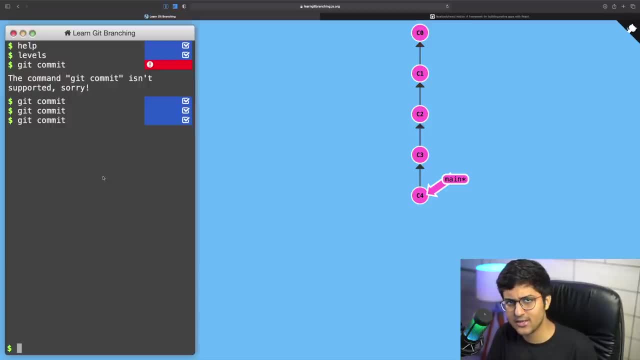 that you are working on should go on a separate branch that the users are not affected. now for that, you can create a new branch like you can. the command is git branch, let's say feature. so I'm working on a feature. you can see a new branch is created called feature. what do I mean by head? 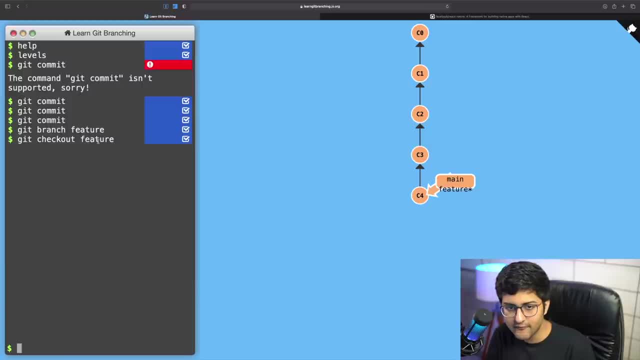 a command was executed called git checkout feature and the star thing that was on main is now on feature. this basically means that my head is now pointing to the feature branch. what is this head? head is just a pointer that says all the new commits that you will be made. 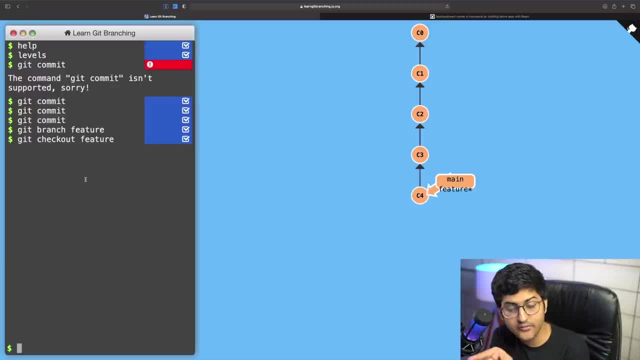 will be added on the head. currently the head is on the feature branch. hence all the new commits I'm making will be added on the feature branch. you can see color being changed and only the feature branch is moving forward. main branches as it is. that is what we want to do. another thing is: 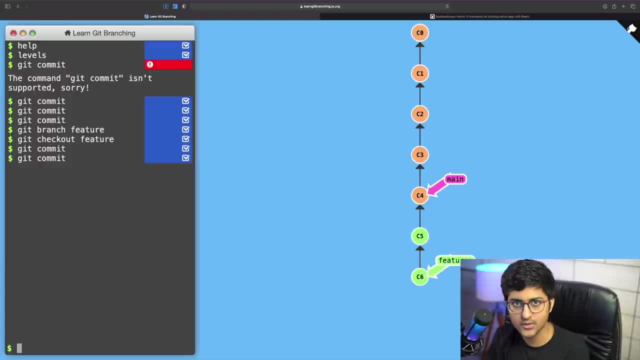 you are not the only one who is going to be contributing to this code base. you can see so many people contribute right to twin- more than two thousand people. so let's say that we want to create a new branch. let's say that while you are working on a project, you're on your separate. 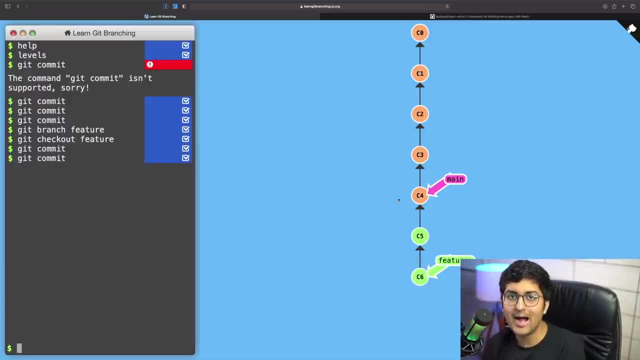 branch. while you are working on your issues, someone else gets their code added in the main branch. we'll talk more about how that happens. that can also happen. so let's say, git checkout, main, git commit. so I can see now the main branch is going on like this and your work is going on side by side. 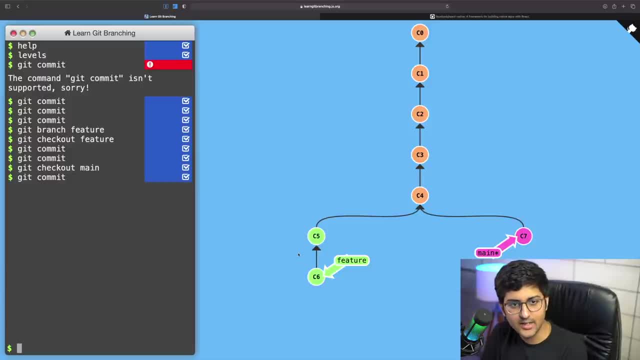 okay, this is the use of branches again, do not worry how this is happening. we'll cover that in detail in a completely hands-on tutorial. but that is basically what branches are. that is what basically what head is. so my currently head is on the main branch. whenever I make a new commit, it will be now. 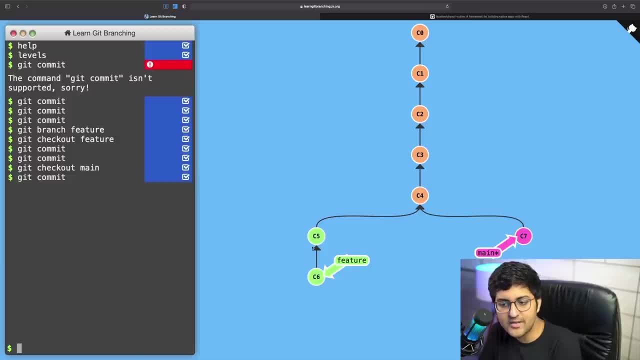 on the main branch now. let's say your features that you are adding in your branch, in your code sample, that are not current, not currently part of the main branch means users cannot see it. let's say these changes are now finalized. you're like, hey, people who maintain this project. you're 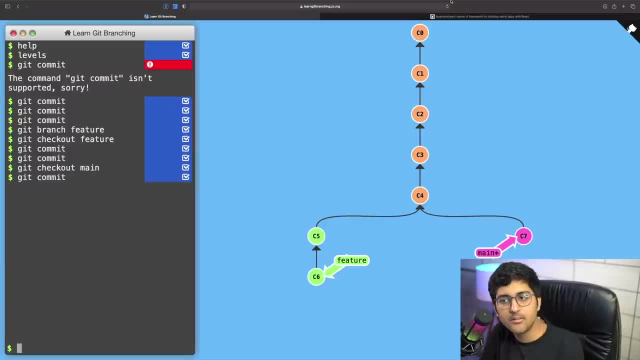 telling them: hey, my code is now finalized. can you please maybe merge this code into into the main code so that the users can also use it? they're gonna be like, yeah sure, git merge feature. now your branch is a part of the main branch. people can actually see this code now. that was in commit c5 and c6. 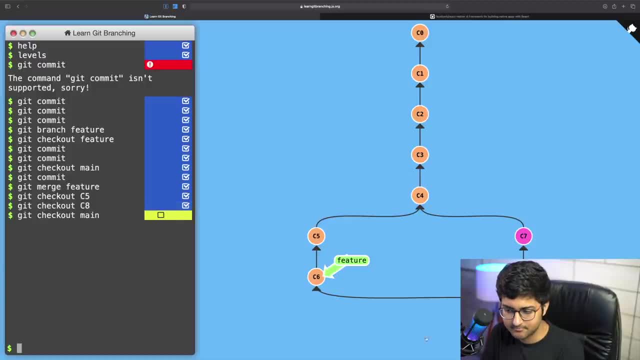 okay, make sense, sound good. I'm. I'm doing it in such a way that, uh, that you all can live. but anyway, how this merging happens, it happens via a pull request. we'll look more into later on. now I know I know there are a few questions you may having. how do we create new? 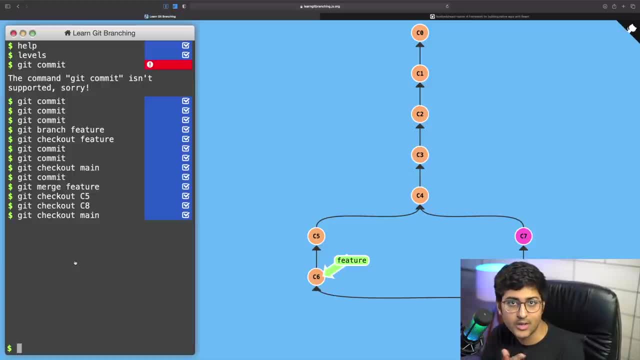 branches. why do we work with new branches? why can't we just- you know every. why can't everyone just work with the main branch? how do we get a new branch merged? what is a pull request? five to six questions you may be having. we'll cover these shortly. if you look at our code sample right now, 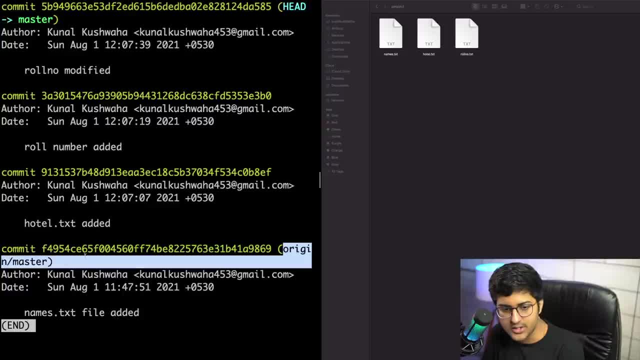 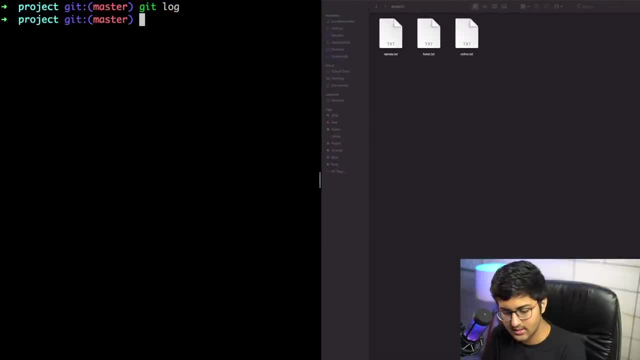 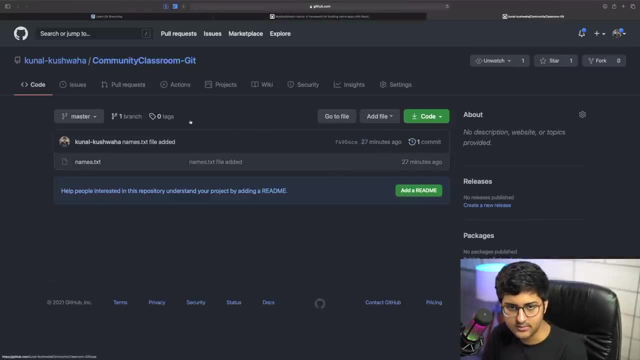 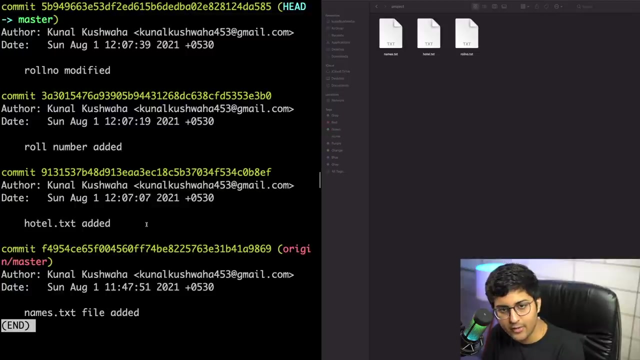 you can see that this is the one on my origins, master branch. okay, that is true. on my own repository I can just open it like this. you can say git remote dash v open it up. only one commit is here. that is true. only one commit is here, because that is the only thing I pushed. this is the only thing I pushed. if I want to push, 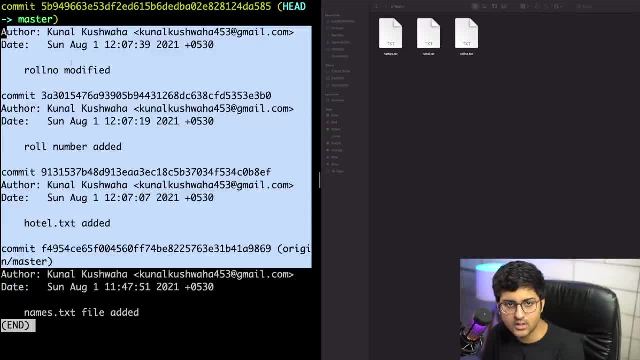 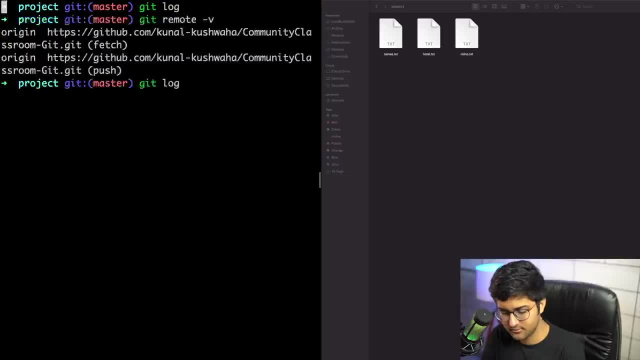 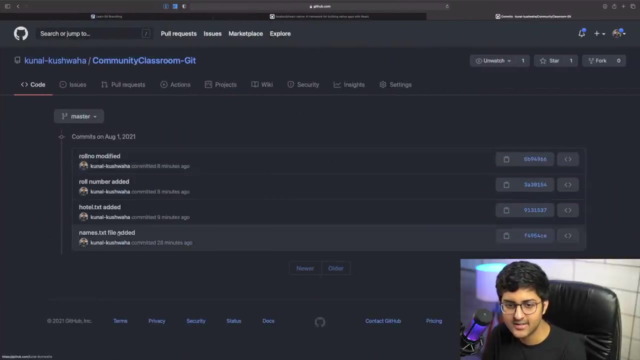 these changes on the new new like and the the new commits. on the master branch I want to push that git push. to which URL do I want to push origin? which branch do I want to push? master branch refresh- ta-da. let's look at the code sample: ta-da. 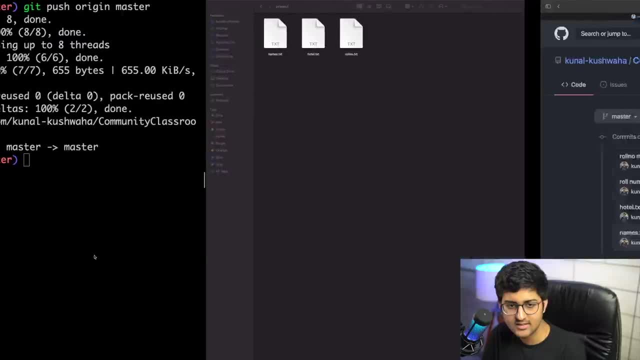 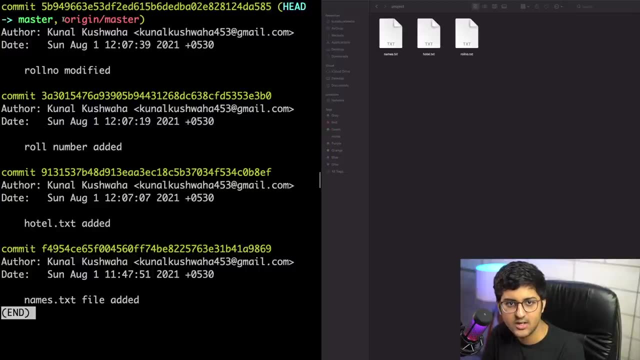 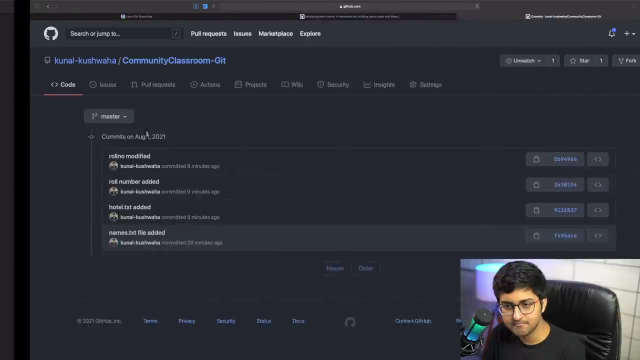 awesome. four commits here, four commits here. head is on the master branch and origin is like the origin the. the URL that I added that is also over here, means there are no commits above it that are extra which are not already on the URL. all right, you can see this is my. you can see this is my master branch. 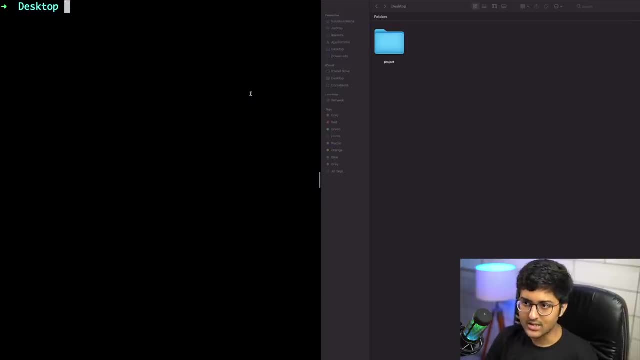 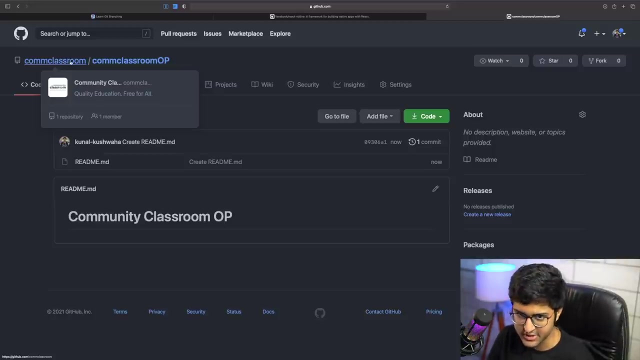 all right now, most of the questions that we need to answer right now. they will be much more clearer when we are doing this next thing, which is known as working with existing projects on GitHub. so let's say that this is the organization, com, classroom, Community Classroom organization, and this is the 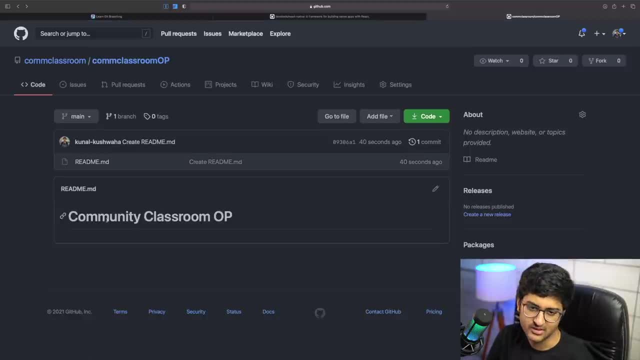 project of that organization, known as a com classroom OP, for example. now, what do we need to do in order to make changes to this project and make some- you know uh- contributions to this project? this is the project on the account of Community Classroom. should anyone who does not have access to it? 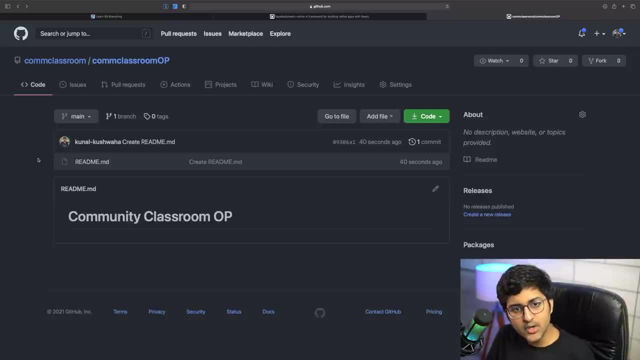 directly like any random person in the world. should they be allowed to make changes to com classroom project directly? how dangerous would that be? so if you try it right now, you will not be able to directly change any file in this folder. currently it only has a readme file. 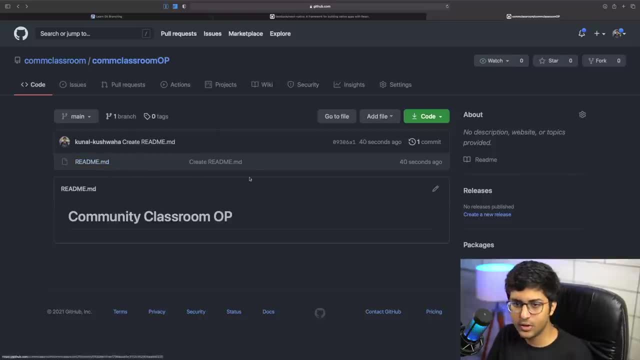 but if you try to change it, you will not be able to do that. why? because you don't have access to this account, this organization. this is a problem that we, you know, face. how do we resolve it? what is a way to contribute to this code sample without you know? 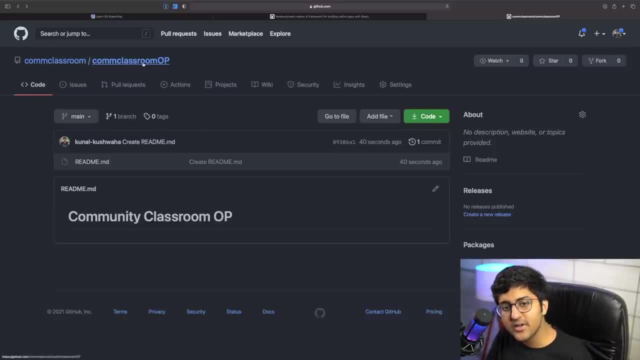 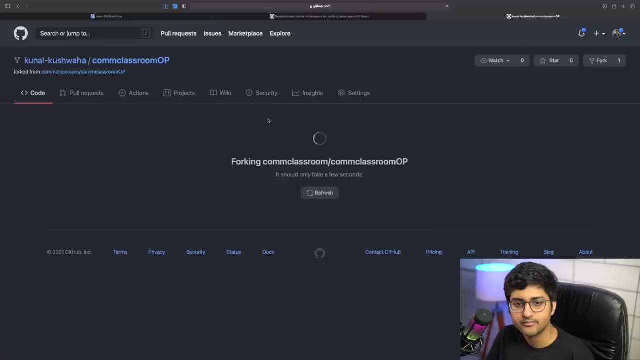 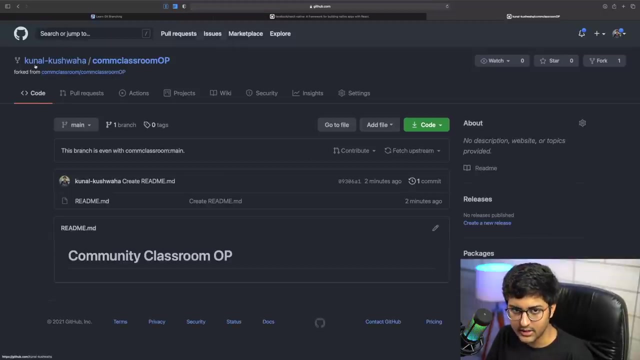 because if we don't have the permission for this, you create a copy of this project in your own account so I can say fork in my own account. so now you can see, instead of com classroom- community classroom op project, it is now kunal kushwaha com classroom op project. 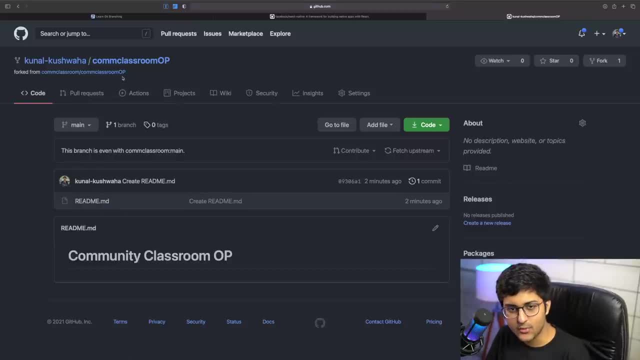 so this thing, you can see this folder, this is a main one and this is yours main one, forked one. now, since this folder, com, classroom op- is in your own account, you can do anything you want with it. let's copy this clone and remember I said: any folder that starts with your own account, the name of that. 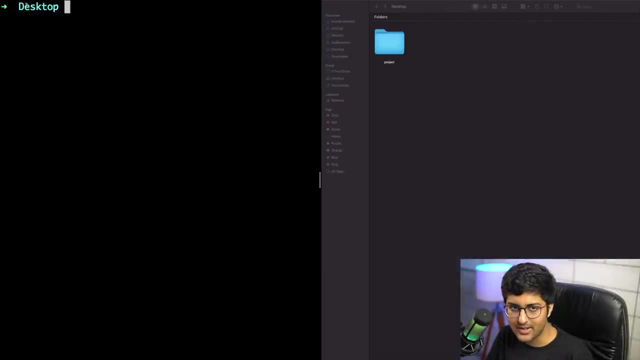 is going to be origin. so whenever I clone this in my desktop, I can say git clone, and then this is going to change it all in my computer. the way I choose to do is I can say using one, or you can even say use another one if you want to. so, for example, 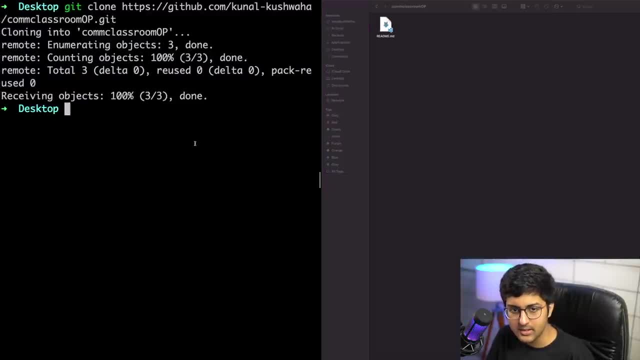 if I want to make this into my booklet, then I can say: git, clone and do that. now what I have to do is I have to create a folder, and I have to create a project, and I have to create a folder, and then the next thing you will see is: 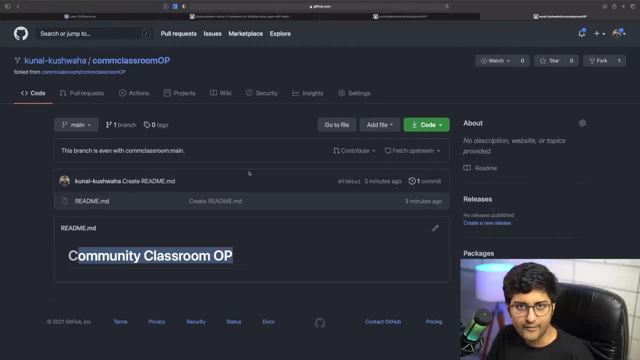 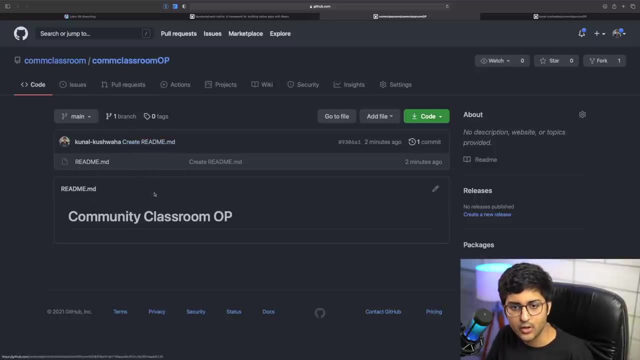 that I have made this as a folder. I can say git clone app and this is the navigation. someone was changing the code sample in your project. you know, without your permission, without anything just like that, that would be very dangerous. but since this is a copy of that, 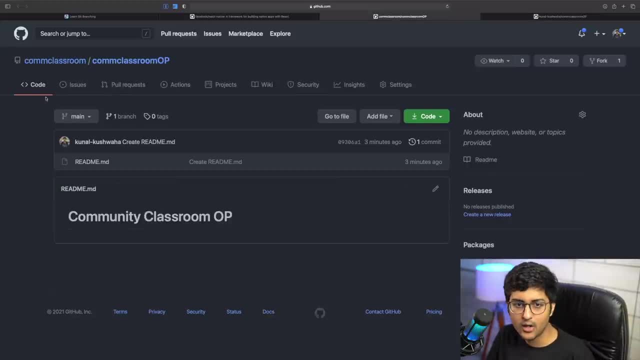 folder in your own account. you can do whatever you want with it. it will not reflect in the main project until and unless the people who have the approval for this project can merge. your code can approve your changes via a pull request, which we'll look into next. so this is what we're doing. 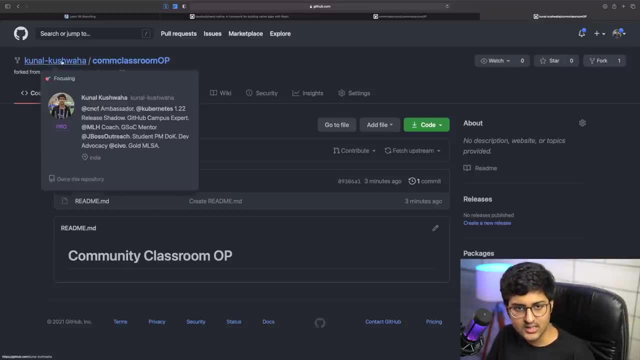 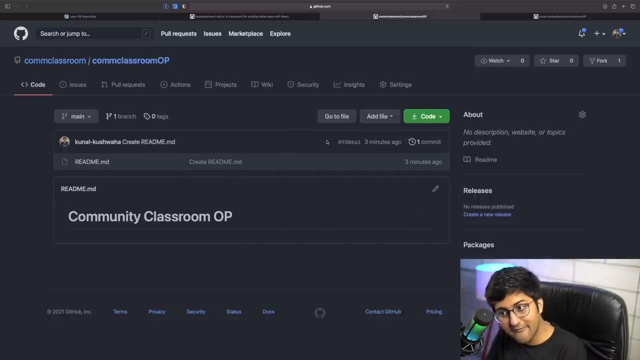 over here and you can see. now, one more thing i want to share is: you know that the origin url is basically your own account. from where you have forked this project means this url. i repeat it again: from where you have forked this project. that is known as upstream url by convention. 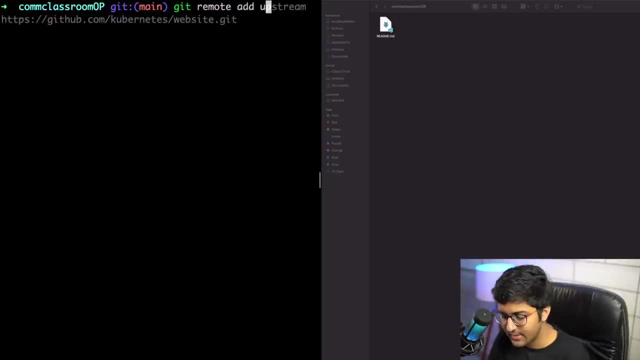 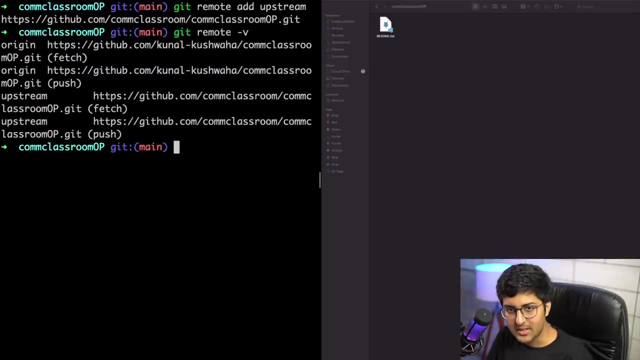 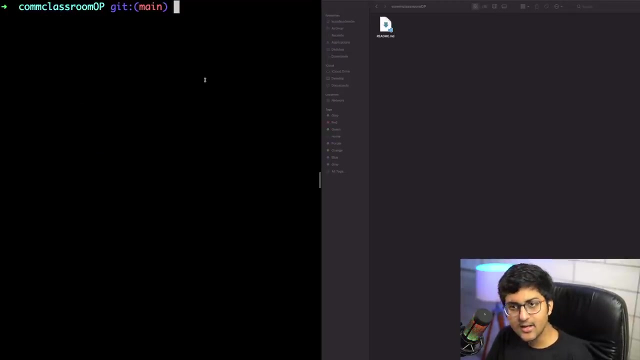 so i can add another url over here. git remote add. upstream url. origin is my personal, upstream is the from where i have forked it. okay, let's say you can do this as well. you can open a pull request after this or via via watching this video as well, so you. 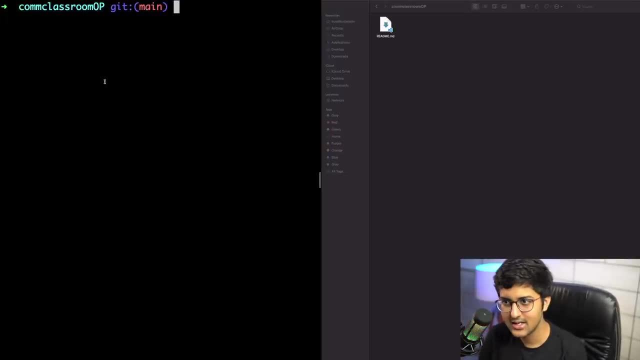 can definitely do this, what i'm doing right now- to get some more hands-on practice. so after you have cloned this, you can create. well, let's do that afterwards. let me first explain what a pull request is. let's say i make a few commits, say we make a few commits, i can say 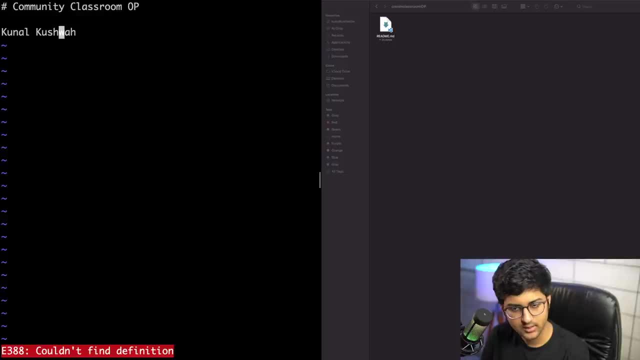 kunal kushwaha, or i can just i can say kunal kushwaha says that this community is amazing. so when you open a pull request you can add, like a dash here, a new point and say your name says that and whatever you feel about the community, okay, so 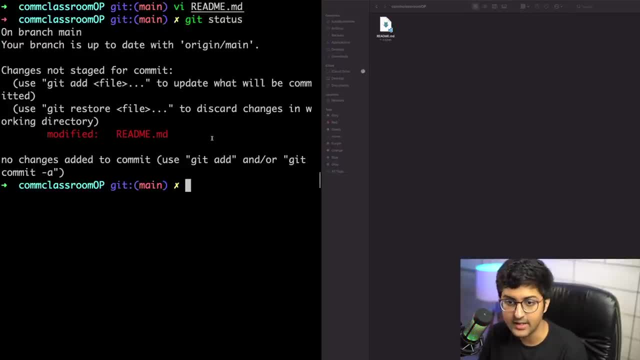 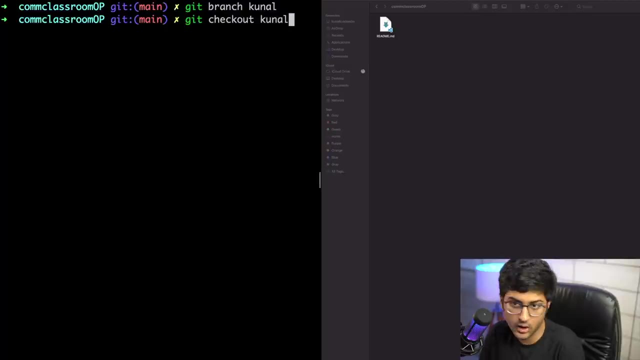 when i do git status, it will obviously show me that readme has been modified. in the beginning i mentioned something to you that never commit on the main branch. always create a new branch for whatever work you are doing. let's create a new branch called kunal. let's check out to that branch. you all know what checkout is now. checkout basically means the head. 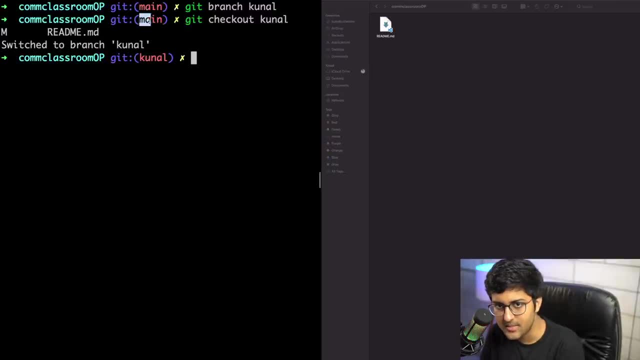 will now come on the kunal branch. that is true. main is now changed to kunal. all the commits i will make now will go on to the kunal branch: git add dot. git. commit minus m. kunal added a message: git log. this is the main branch, not changed only till. here we have the commits and 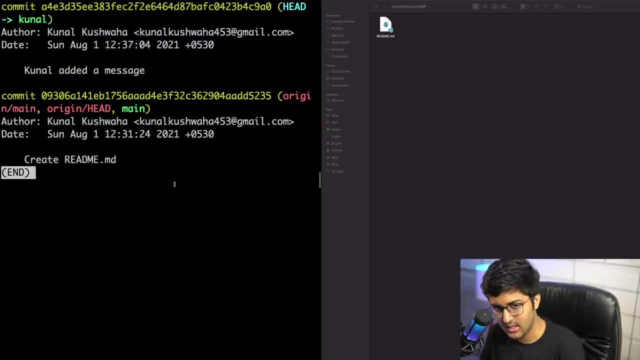 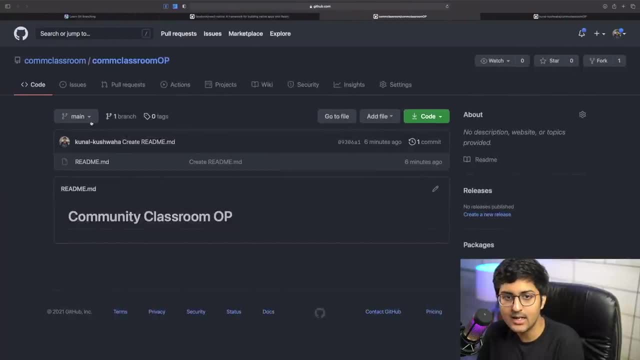 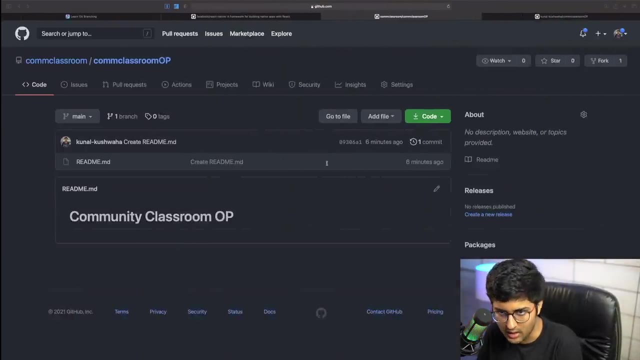 the kunal branch has an extra commit. now, basically, what i want to do is i want to push this branch. i want to say the idea is that, hey, whatever code that i have in this branch, the kunal branch of my own account, please merge that into the main project's main branch. that is, you will do what you. 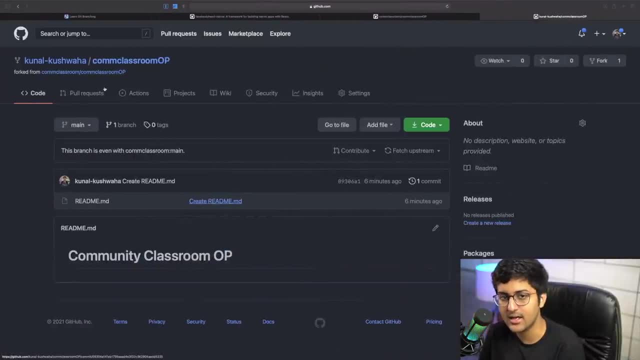 will do. let's say rahul wants to add something. so rahul will say, hey, rahul's account has a com classroom project. so rahul will say, hey, rahul's account has a com classroom project and he will have a branch called rahul branch or rahul temp or whatever name he wants to give. 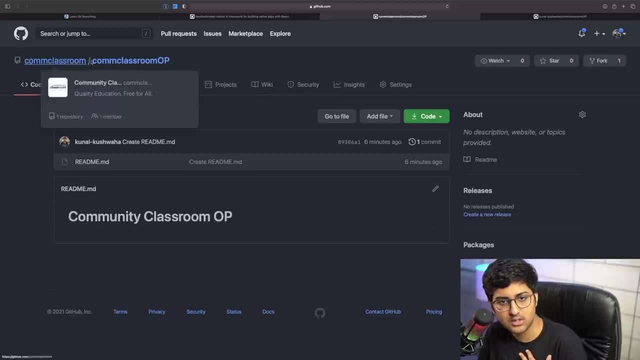 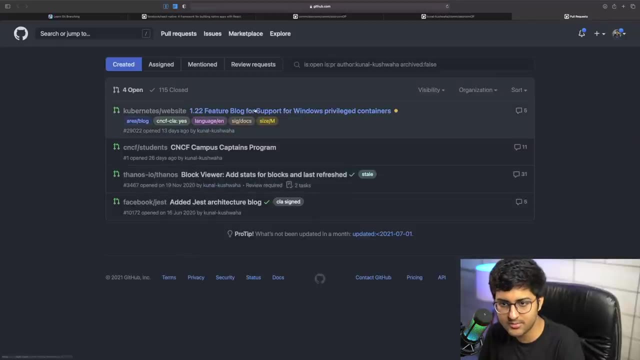 and then he will request me- the person who is responsible for the main project, like, hey, i have something. let's open up some pull request. let's say some pull request that i got merged previously. this is an open one. let's see the one that was merged. so this one was merged. 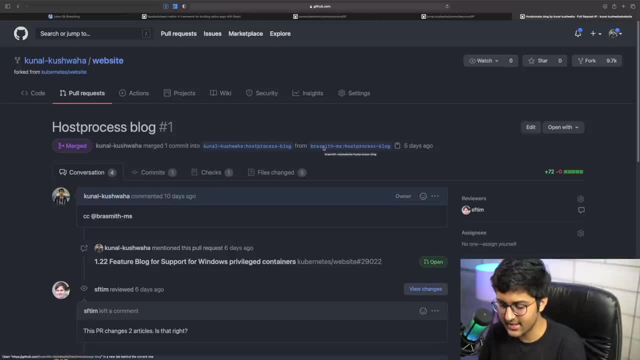 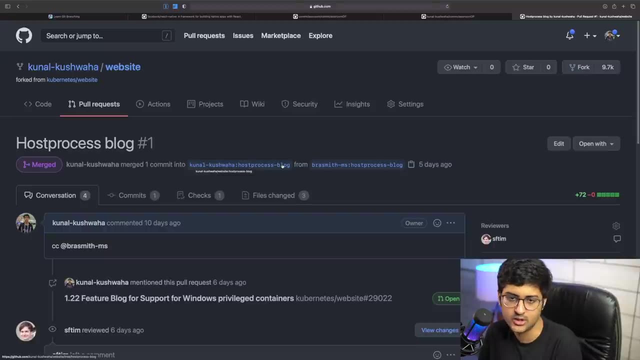 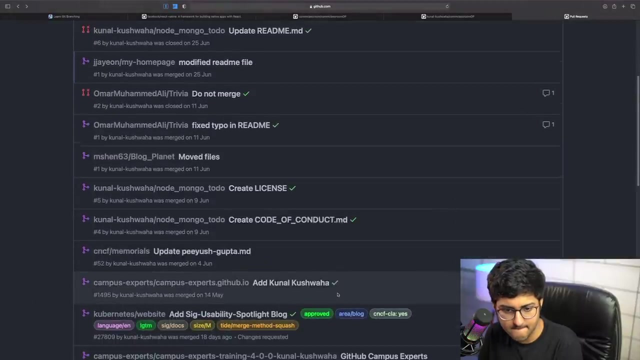 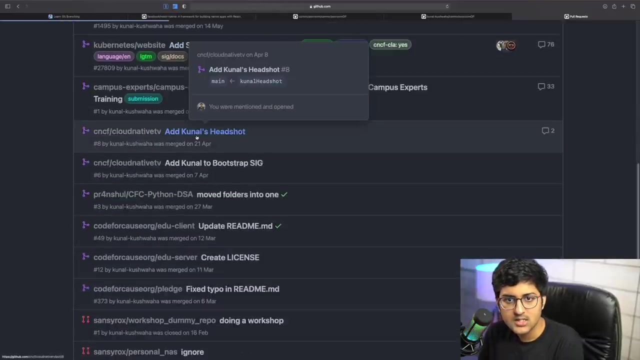 so brad was saying like: hey, i have a branch known as host process kunal. can you please merge that branch into your host process branch? or let's look into the more simple example, this one. so i, let's say, wanted to contribute to the kubernetes website. this is a really nice example. 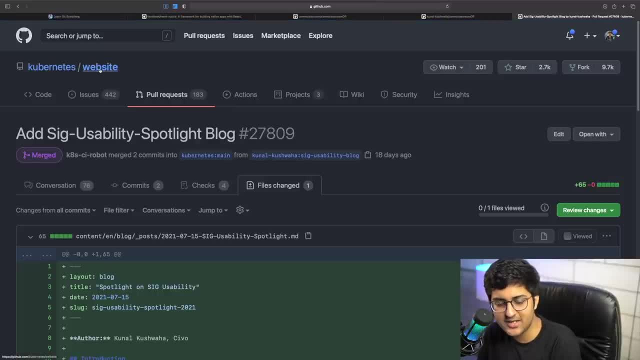 i said that, hey, obviously i cannot change your website directly, so i created a fork of it. you can see kunal kushwaha. the kunal kushwaha fork has a branch called sig usability blog which contains these changes. and then i am requesting the people who maintain this project: 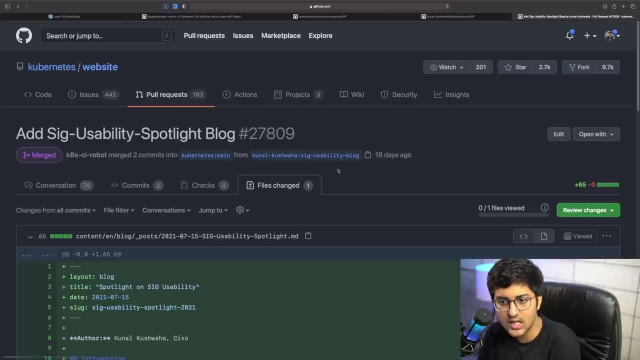 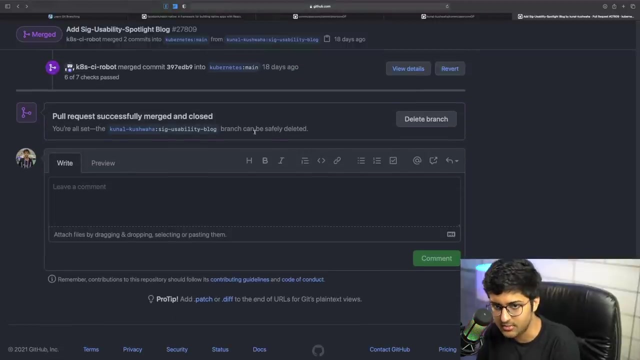 like: hey, whatever changes i have in this branch, can you please merge it into the kubernetes main projects main branch so that the other people will be able to see that? and after that they were like: they gave some suggestions, they ran some tests, i made some changes. in the end, my pr was merged. 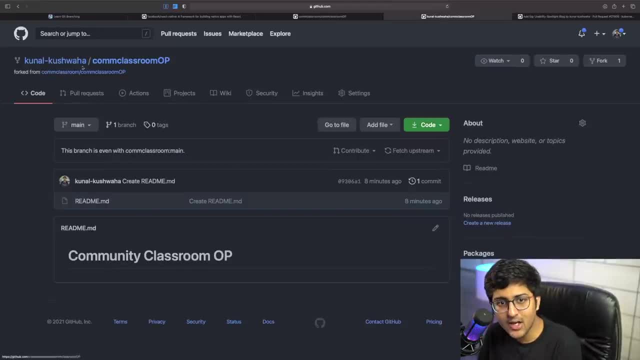 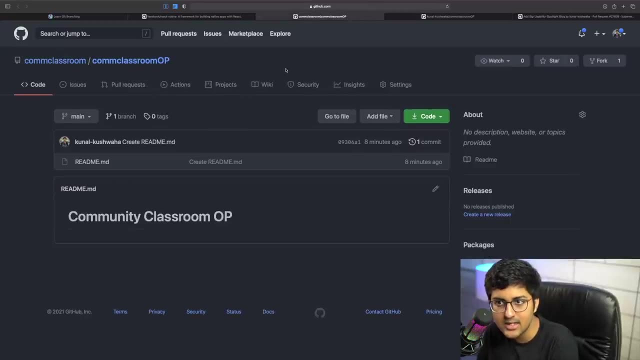 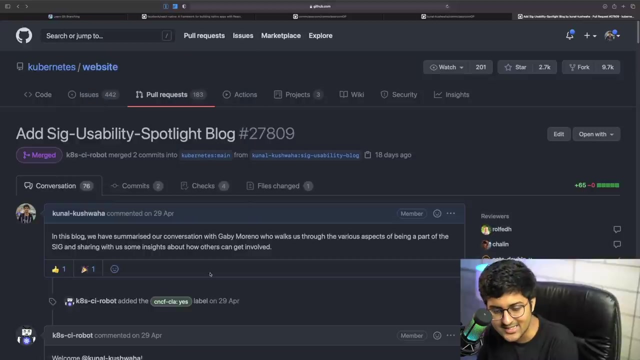 this is what is known as a pull request. so when you create your own copy and you create any change in your copy, how do you make sure that this change, whatever you create in your copy, is visible in the main project? you request it via a pull request. then people will review your code. suggest some. 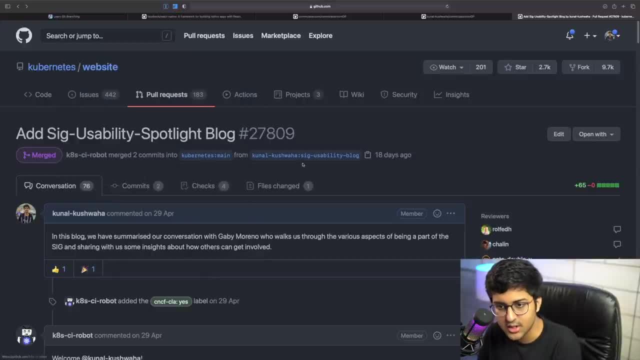 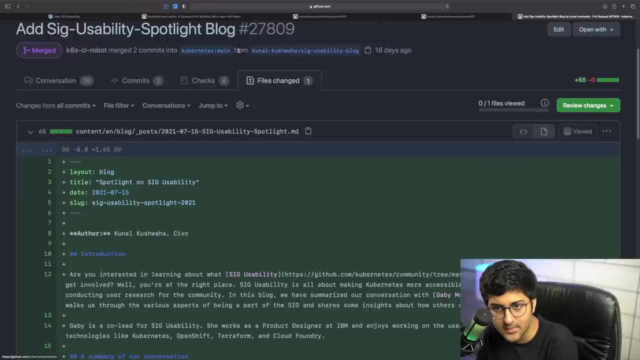 changes, you will make those changes and when this is merged, your code sample changes that you made in your own accounts fork in any branch. that will be visible in the main projects main branch. so once this is merged, this is merged now. so basically, this code sample is now in the main. 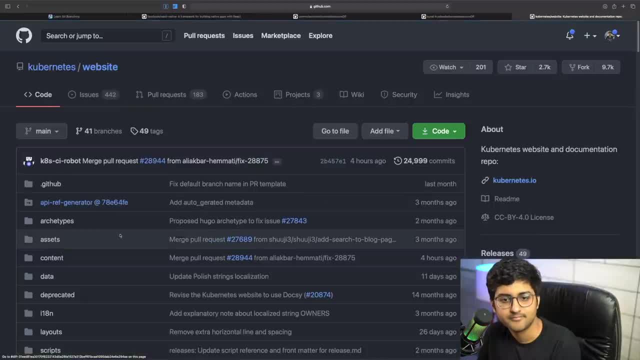 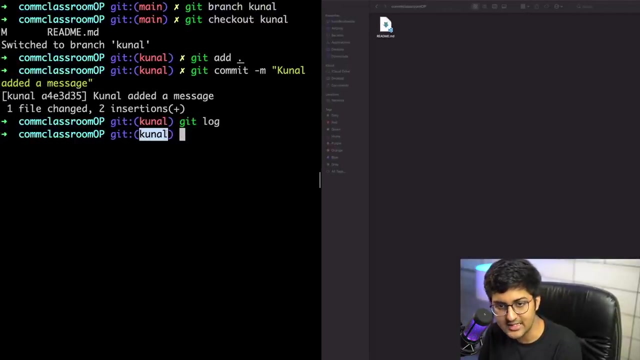 kubernetes website in the commits. it is main website over here. somewhere over here my blog is available. okay, that is what we are doing over here. now i will give you another example on why you should never commit on master branch and always create such branches. to sum up, if you have any new feature you are working on, on any new bug you are working on, or 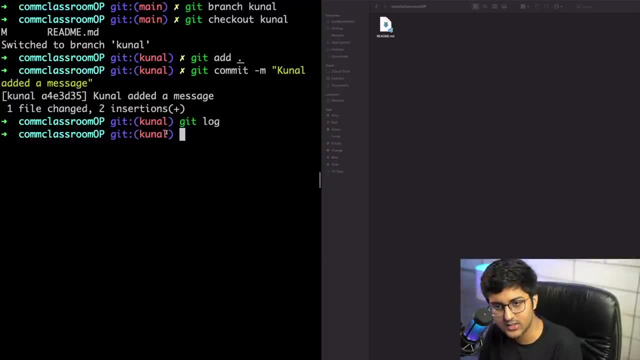 any new thing you're working on. make sure you open a new branch for that and a new pull request for that. it will be much more evident when we give this example. let me push this branch on github. i want to push on origin, if you, would you all be able to push on upstream? no, because you don't have. 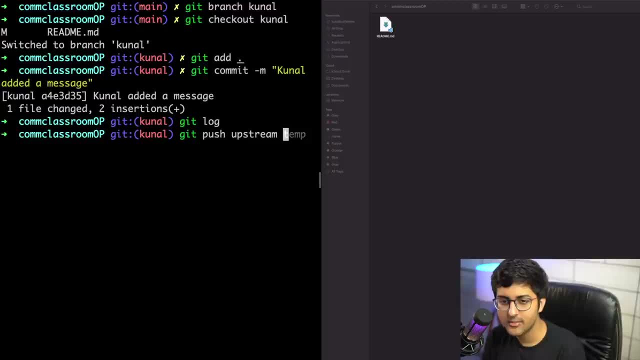 access to community classroom organization. if you say git, push upstream your own branch name, it will. you will not be able to push it. how can you push to upstream url? you don't have access to it, but you have access to the origin url because origin is your own account. let's go to it. as you can see, 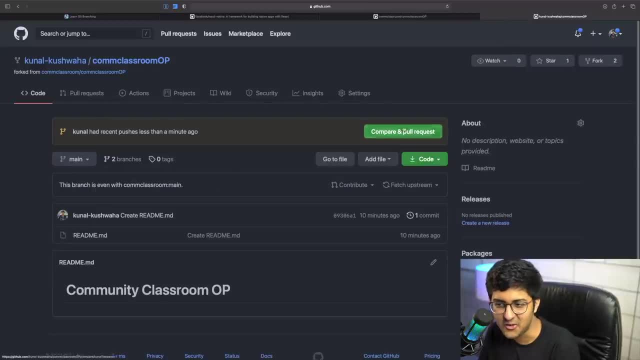 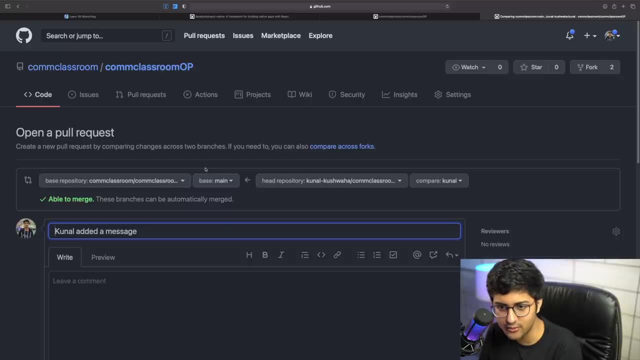 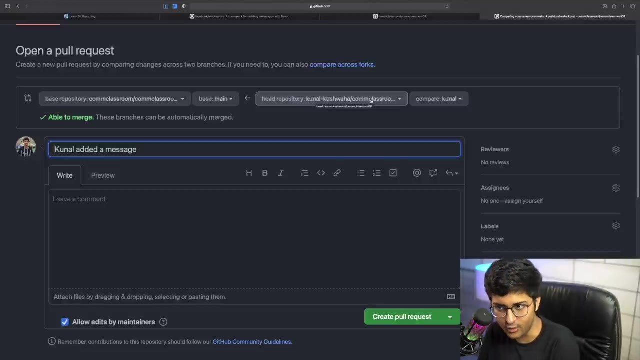 there's an info, there's a this thing, this thing, like all, automatically it's saying us click on this. this is what you need to do whenever you add yours like this, you, you have to make sure that hey, let's say rahul is doing it. so rahul's kunal, rahul's com classroom copy, or the fork has a branch. 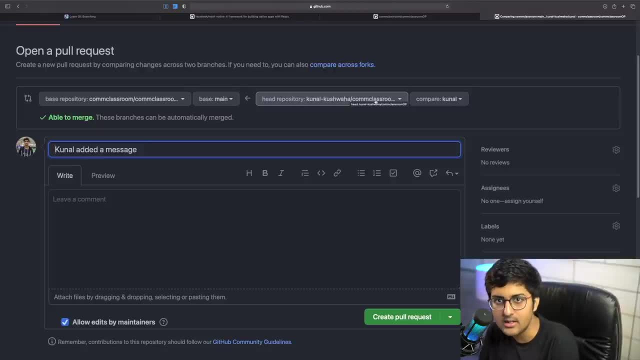 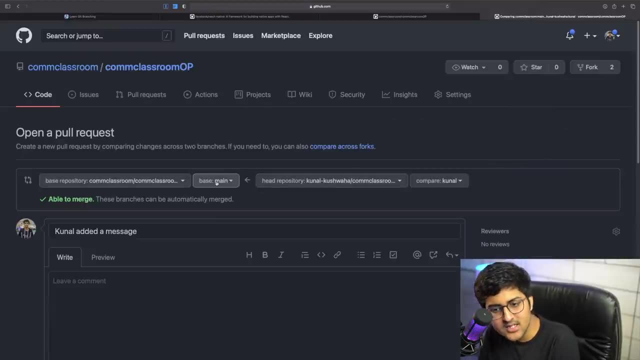 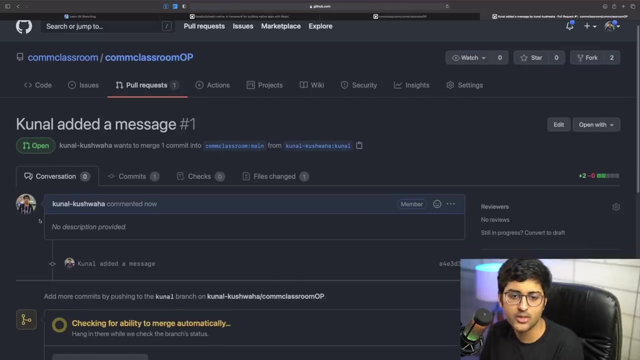 called rahul, let's say, or kunal's com classroom copy has a branch called kunal and that branch contains these changes. i am requesting, hey, please merge these changes into the main branch of the project. create a new pull request. when you create a new pull request, i will get this notification. 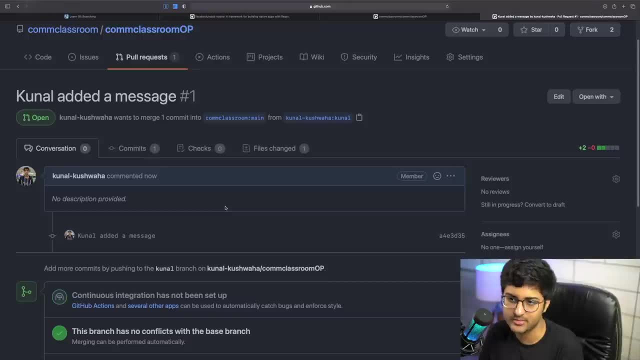 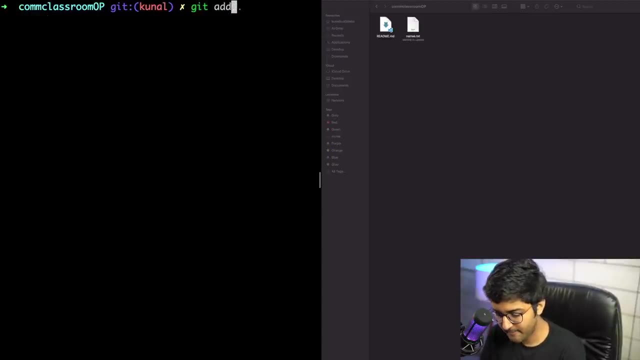 and then i can merge this code. before merging, i need to show you something else. let's say i want to make some other changes. let's say i say: touch namestxt you. you can see this git commit that i am doing. it's going into the main. 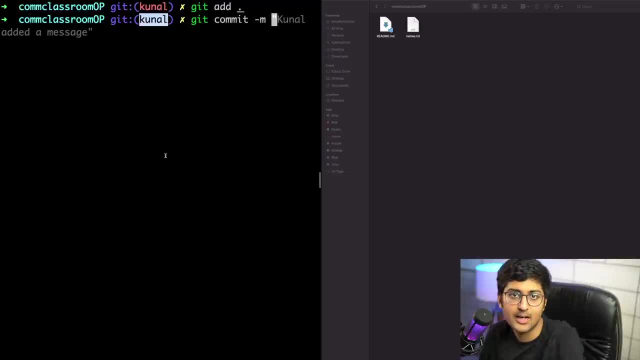 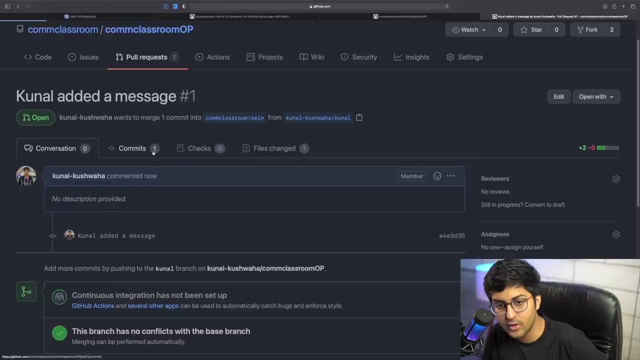 not the main branch but the kunal branch, because head is at the kunal branch right now. i did git checkout kunal. this is something i'm just doing to show you git push origin: kunal. you will notice that now it will allow me to create a new pull request. it will add these commits here. only this will now become from. 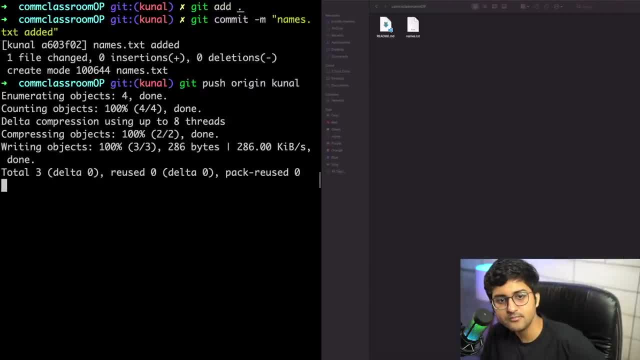 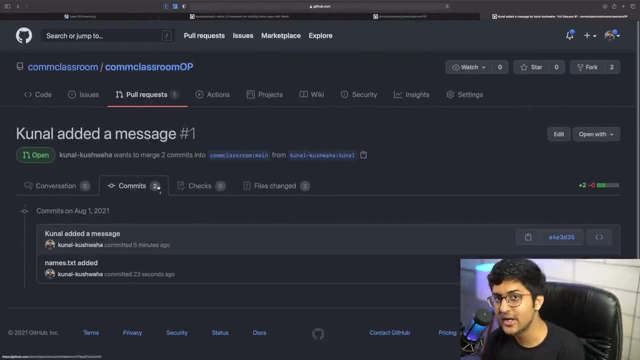 one to two, let's see. let's see refresh two. this is the reason you should never commit on main branch. why imagine you're working on 10 projects and let's say you're working on 10 features and for every feature you want, you create just one pull request. 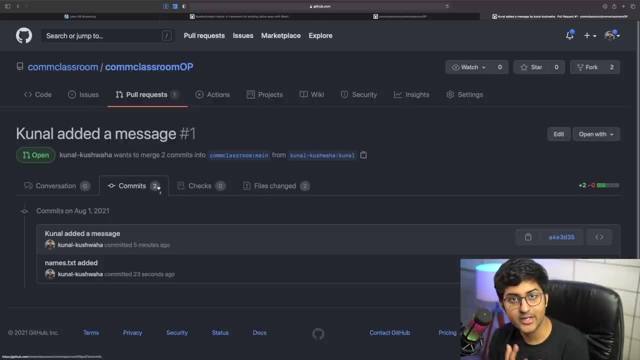 how difficult would it be to review your code, to have the discussion? it would be very difficult. all the 10 different things on on just one pull request. that is why, for every new feature, every new bug or anything you are working on, create a new pull request. and from this example you can see: 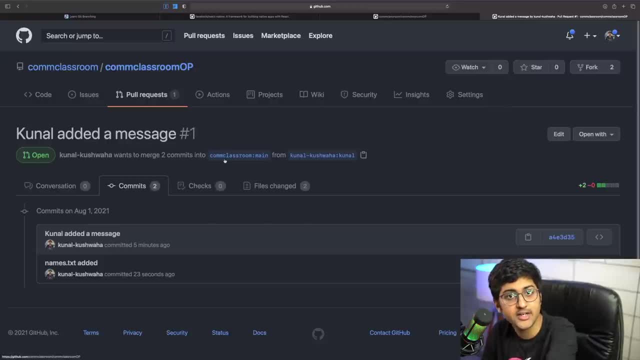 that if a branch already has a pull request associated with it, it will not allow you to create a new pull request. all the commits will be added to that full request. only in simple language, one pull request means one branch. one branch can only open one pull request. if 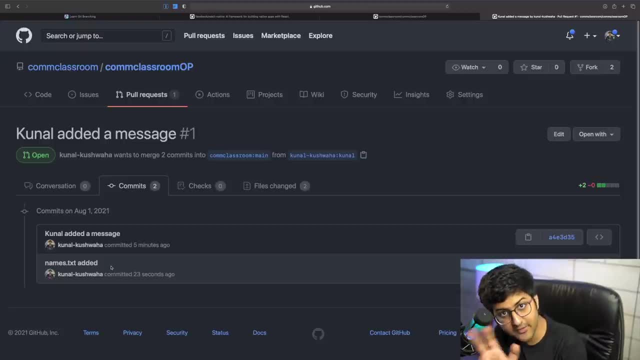 you want to open different pull requests for different features that you are working on in the project, which is also recommended, that for that you want to open different pull requests, and since only one branch can be associated to one pull request, so hence you will be able to need to create different branches, so 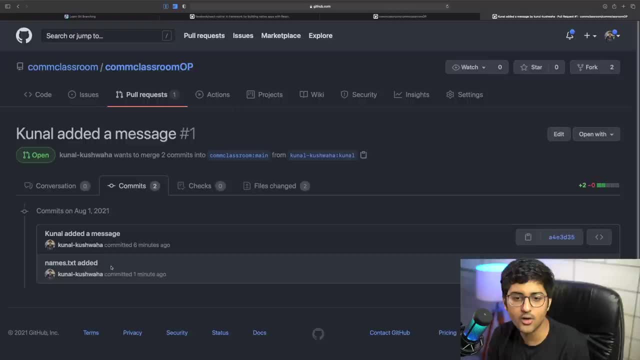 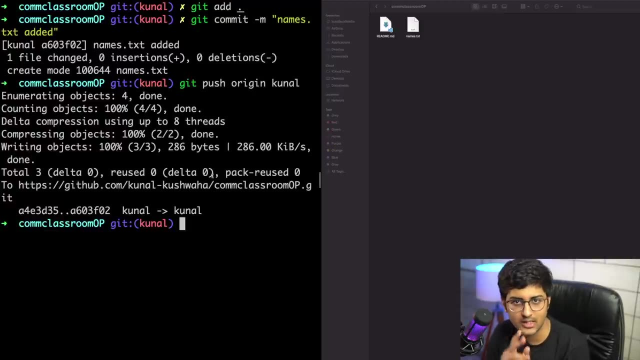 I hope that makes sense. any particular new thing you are working on, create a new branch in your local folder. make a pull request from that. you can have 10 branches, 20 branches, 100 branches, whatever you like. make sure your work is distributed like this so that it does not get mixed up. okay, imagine one. feature has 10,000 changes, 10,000 lines of changes, and you're working on 10 such features. how difficult would it be to manage such a thing? very difficult if you just created just one pull request for all the 10 features. don't do that. 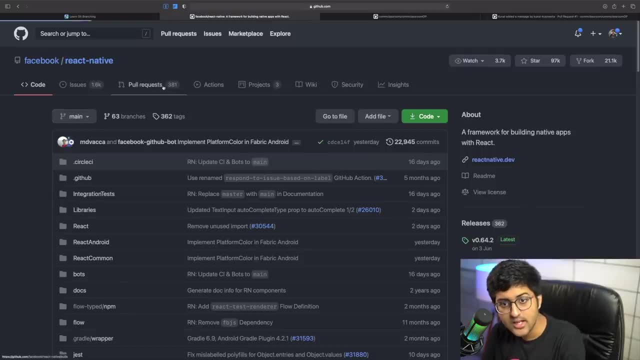 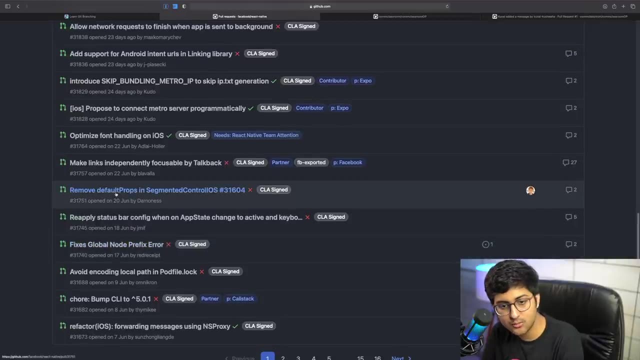 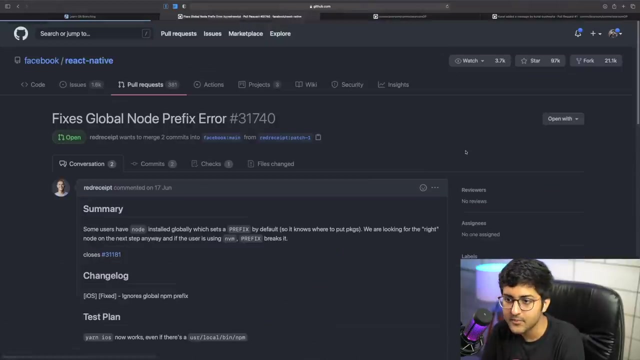 okay, don't do that. react next: 380 one pull requests are currently open. this is doing something with pod log file. this is fixing some global node. this is removing some default property. this is doing something with, like iOS. imagine all of these changes that were being made. let's say, you know 4 lines of changes being made and here something. 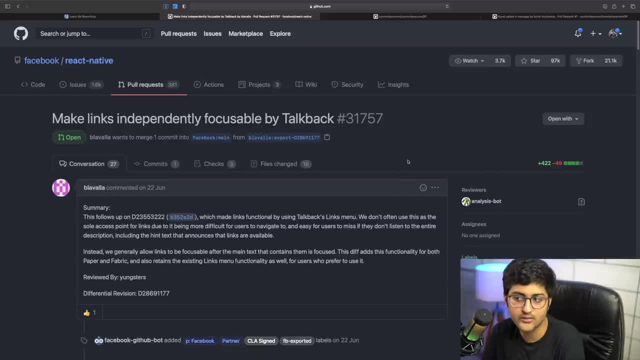 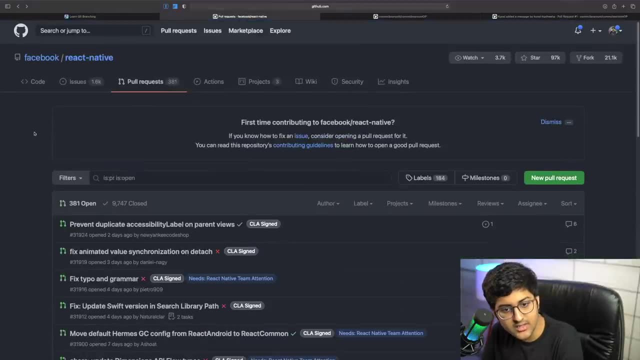 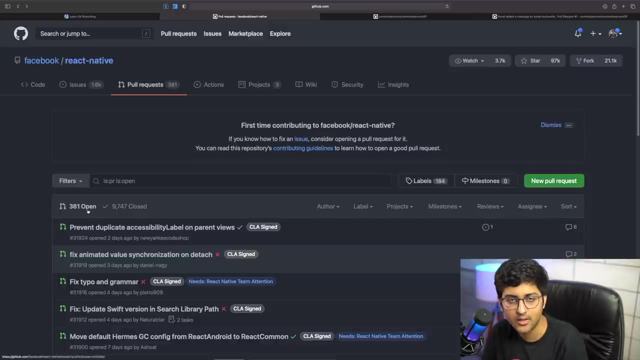 like some other line 422 lines of changes being made. we know that these 16 files that have been changed relate to this particular issue. now imagine all of these other pull requests were only on one single branch and one single PR. these 381 features or issues or bugs they are working on, let's say there was just one. 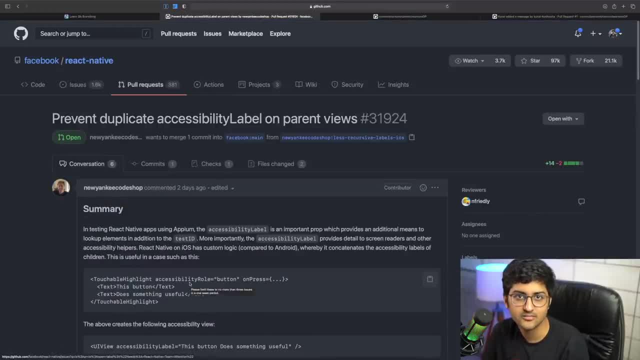 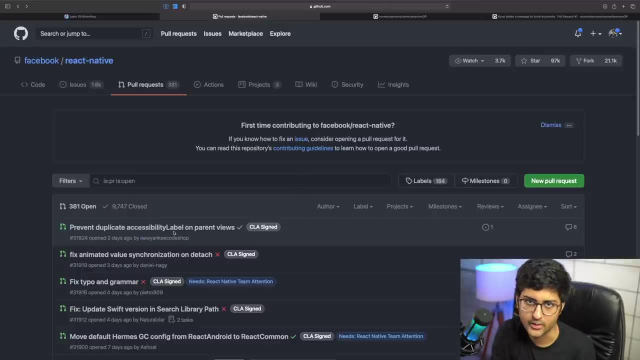 PR for this. how difficult would it be to manage and also many people would have to collaborate then on the single PR. that does not make sense. everyone is working on their own pull requests. okay, that is in short, and now you also know why you should never commit on main branch, because if you do all the commits, 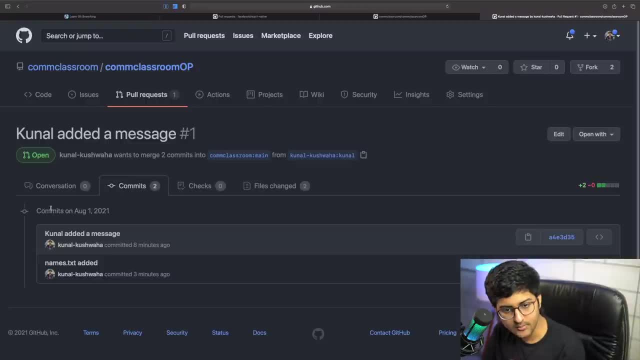 on main branch and not create another new branches, all the commits will go on the main branch only. Similarly, if you make all the commits on the Kunal branch, all the commits will come over here. If I want to add some new feature to this project, if I 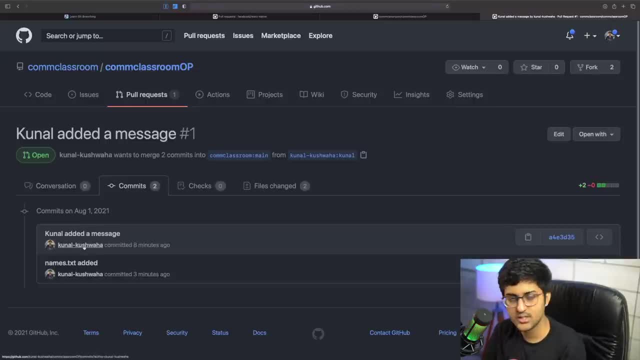 add it over in this branch only, it will come in this branch only, which is something I don't want to do, because I've already explained it multiple times. Make sure for every new feature bug you create new branch so that you can open a new pull request. So if someone 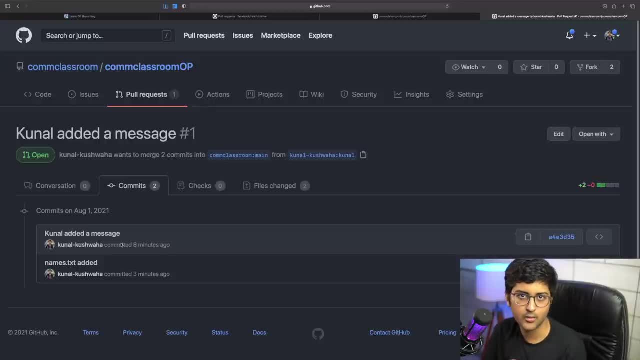 asks you why we create new branches? because we want to open a new pull request. and we can only open new pull requests with new branches. If a branch already has a pull request open, then we don't want to. We can't do that. All the commits will be added here, only Another. 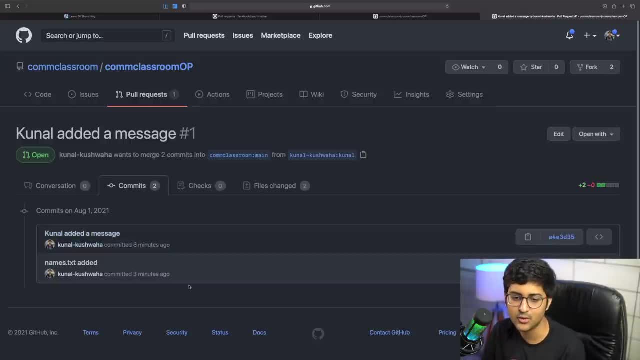 thing you may encounter is: now, this is an extra commit. Let's say you don't want this commit, this particular commit, namestxt file added. If I look at the code sample, I look at the code sample for this, So you can see two files have been changed. Readme file was: 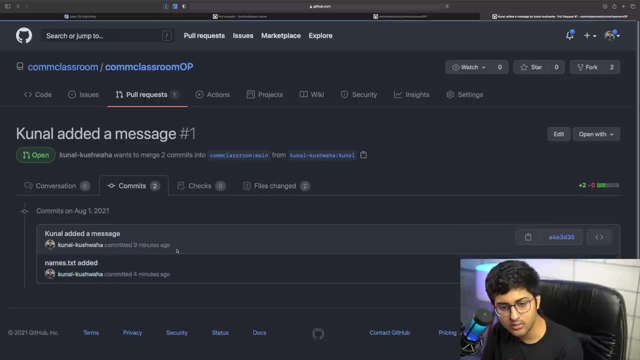 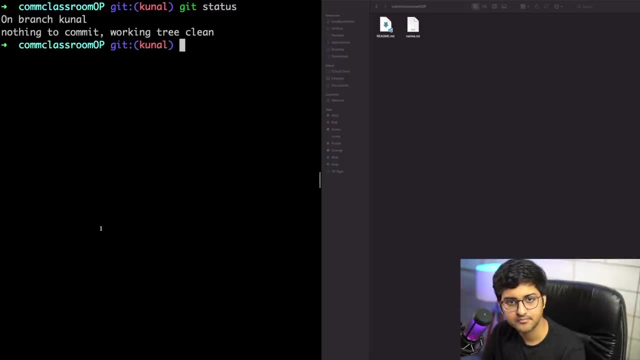 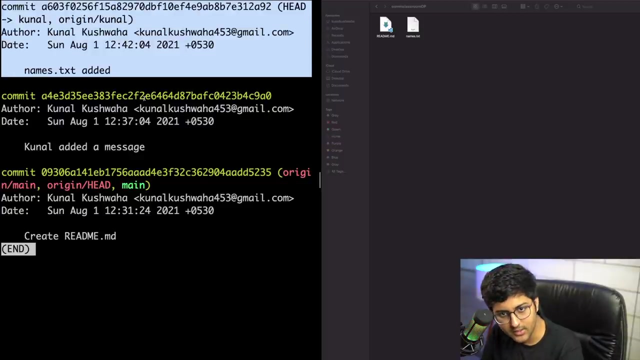 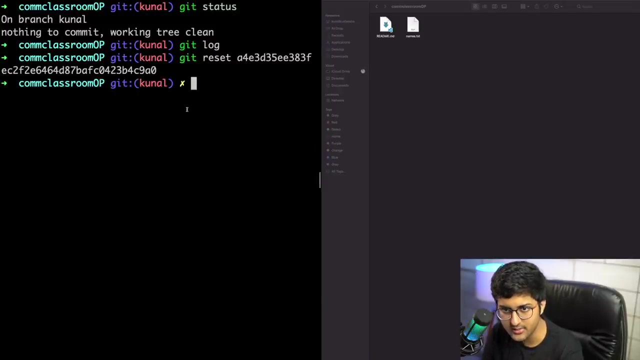 changed and namestxt was added. Let's say, I want to remove this commit, the namestxt commit Reset thing. I did reset previously git status, git log, sorry, So I will just copy this thing. I want to remove this, so I will copy the one below it: Git reset. Now this namestxt will be unstaged. 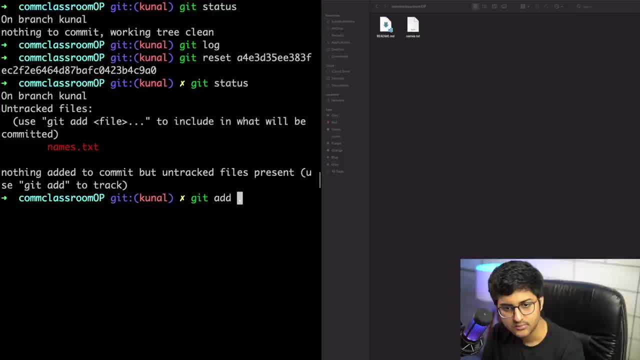 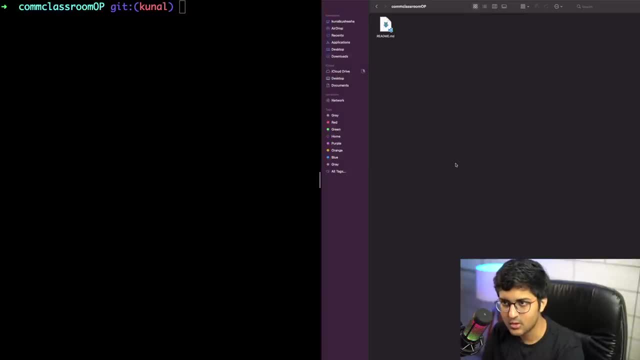 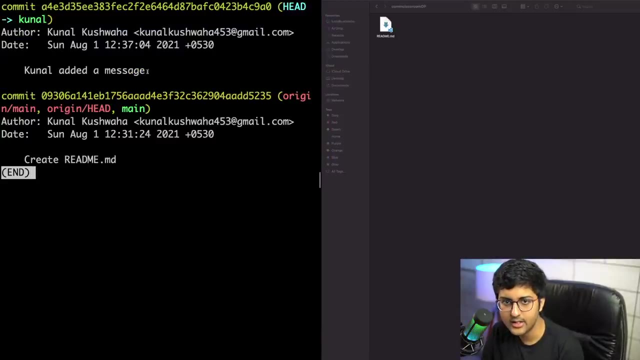 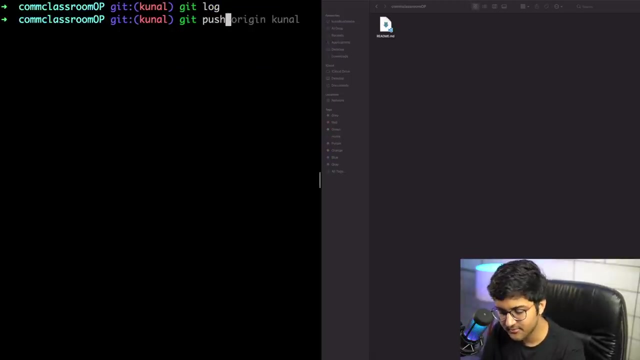 I can say git addtxt. I can do git stash. It will go back to some stash area Gone. My structure is now exactly like I wanted: Namestxt file deleted and the commit is also deleted. It is also removed from the commit history. When I push this, I would have to force push this because the 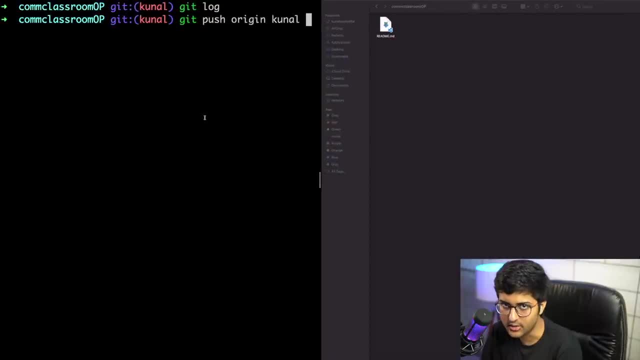 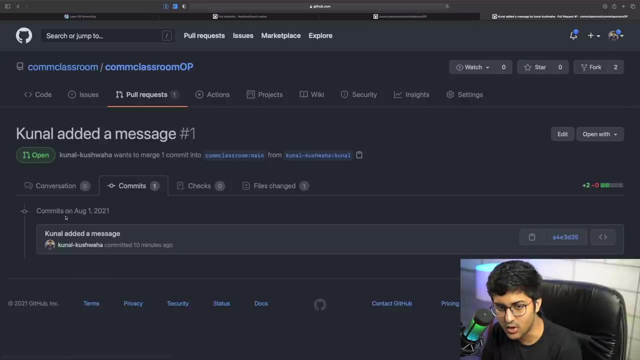 online repository contains a commit that my repository does not, And I told you commits are interlinked, So I will have to force push this Dash f Let's refresh That. commit is gone. File change also to one only Namestxt file is gone. Commit is also one only Main commit that. 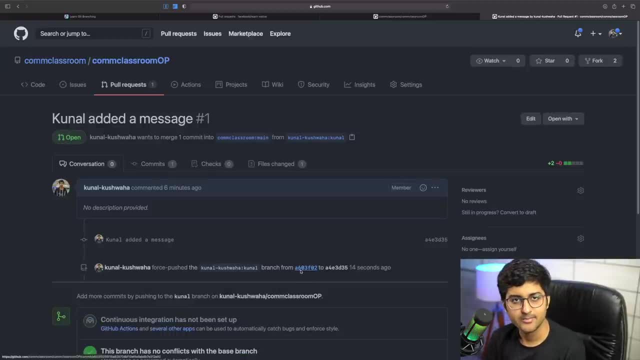 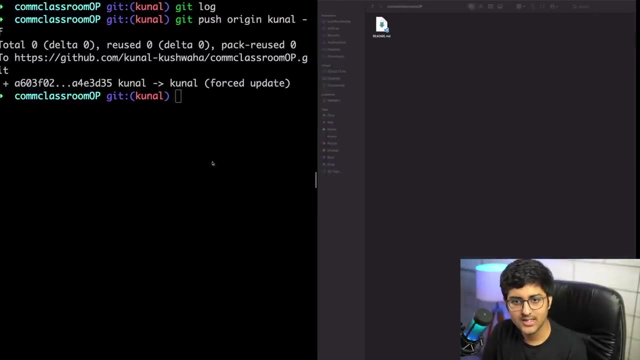 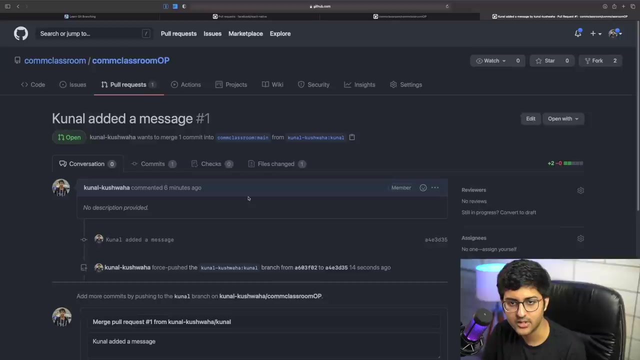 I wanted. That's it, As simple as it gets. That is how you work with pull requests. Alright, Cool. So the next thing may be related to merging your pull request. So let's say, we merge this pull request. I can merge this. Confirm. merge Now the changes I made in Kunal Kuswaha's. 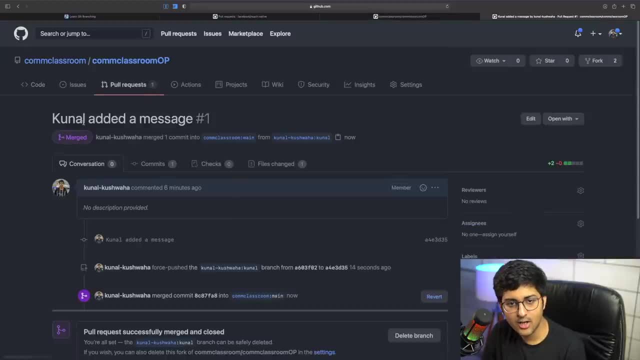 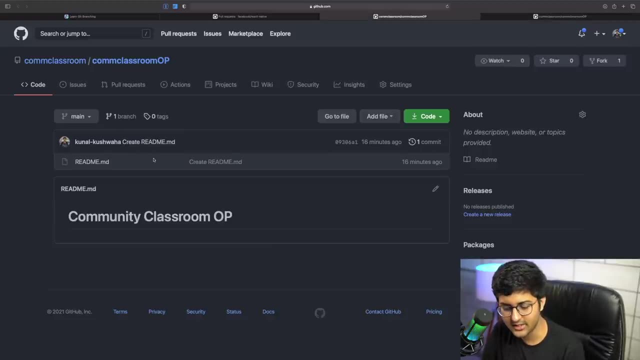 Kunal branch Here. They will now be represented in the main project. Let's see Ta da Changes I made in my own project. They are now merged into the main project. I hope that makes sense. Okay, Cool. One more thing we can notice is that the fork is not updated. That is true If you. 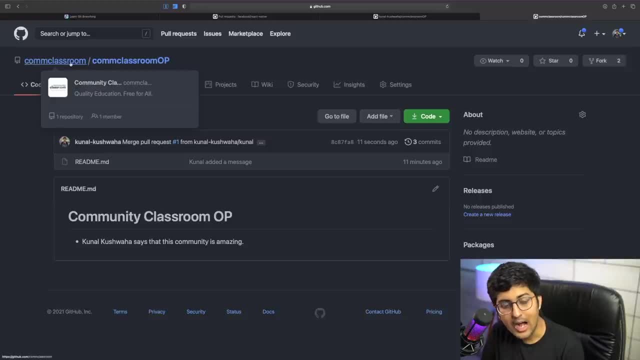 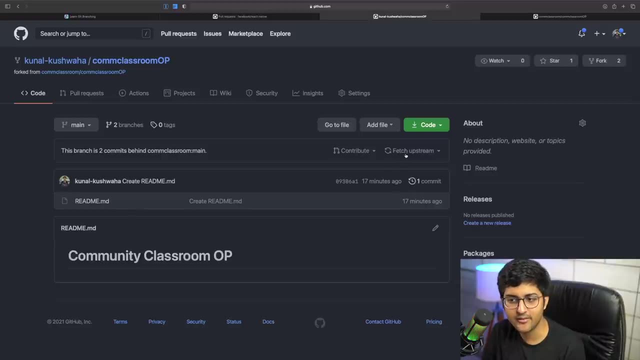 cannot directly change the account of com classroom. how can com classroom directly change your account? They can't do it. There are two ways to do this. You can click on this button: Fetch upstream. It basically means this branch is two commits behind the. 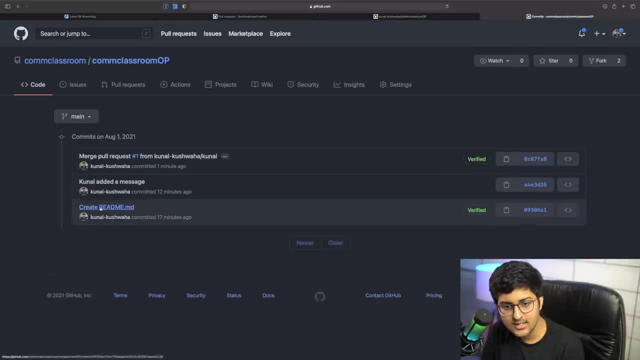 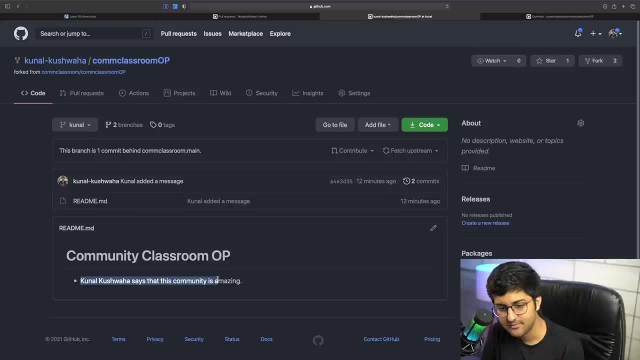 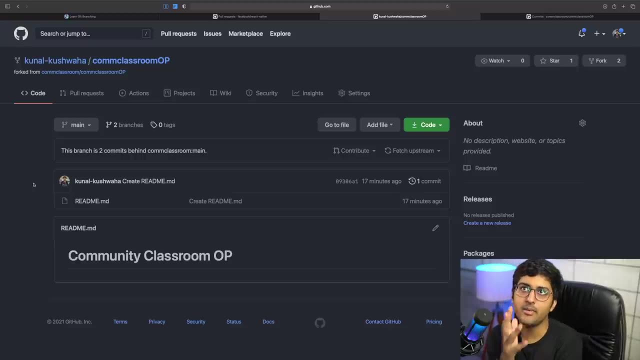 the extra commit that I had was in the Kunal branch. It was not in the main branch. So this is the reason you might encounter something like: hey, some other person merged their code in the main branch. I want to look at that code sample as well in my own fork. How do I make sure that the 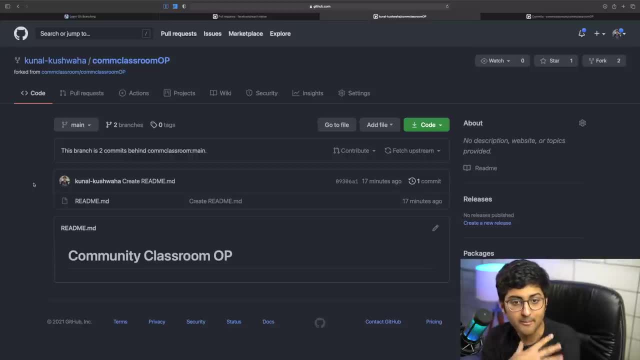 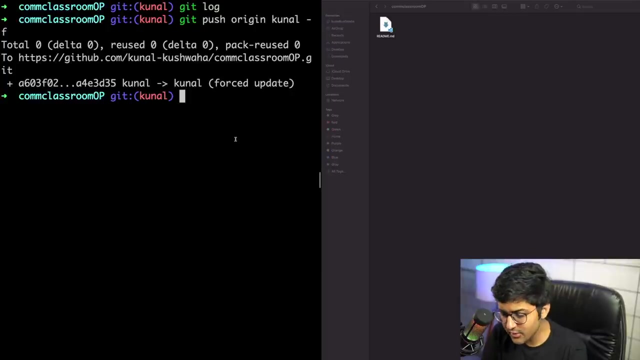 main branch of the upstream- Okay, own forks- main branch is always maintained. there are a few commands that you can use for that. you can also use this button called fetch upstream, but I will actually teach you how to do it manually. first thing you need to do is: 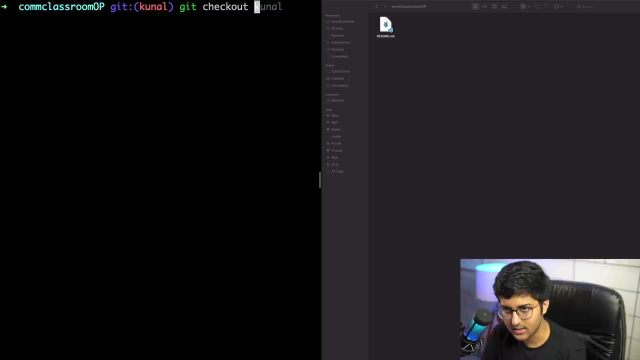 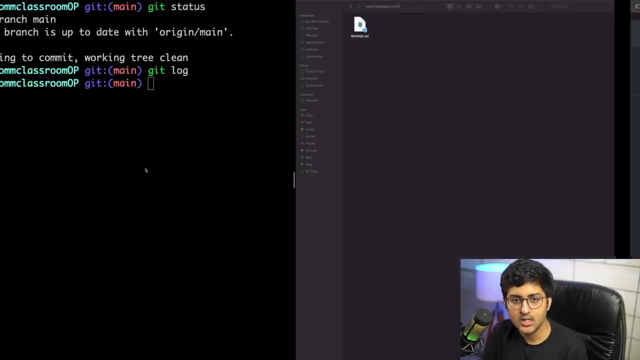 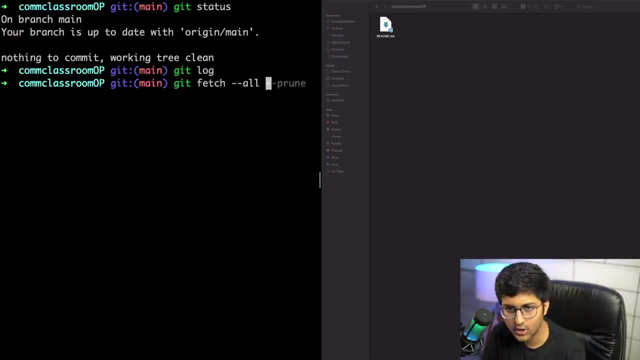 git checkout your main branch so you can see, here in the main branch of my fork I only have one commit, but in reality in upstream it has three commits. first thing we need to do is we need to fetch all these commits and changes. git fetch, dash, dash, all, all the branches. the prune means the ones that are deleted. they. 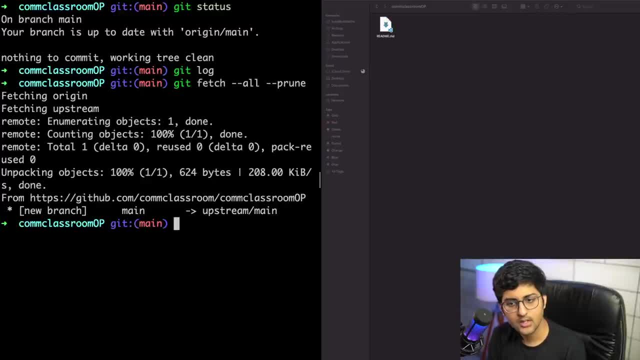 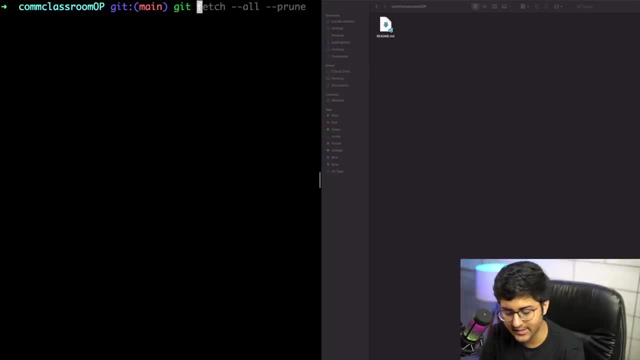 will also be fetched. okay, now I've fetched all the changes, first step. that was the first step. second is git checkout main. but you have already done that. after that you need to do. one more thing you need to do is you need to fetch all the commands that are deleted and after that we can reset it, reset the main. 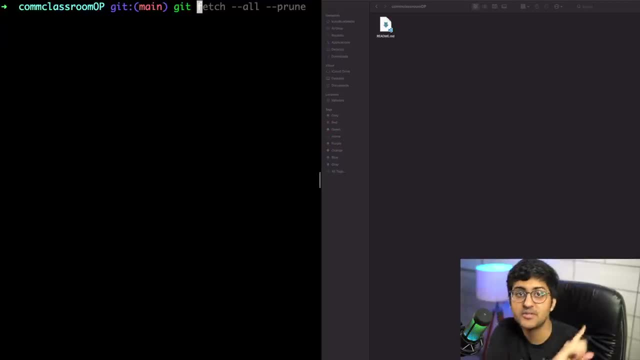 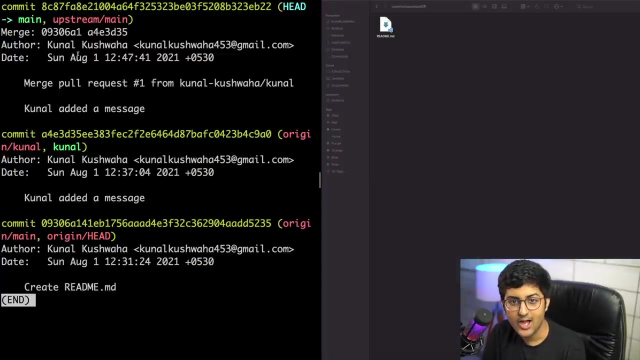 branch of my origin to the main branch of upstream git reset. dash, dash hard. upstream main branch git log. three commits, three commits here, three commits here. now my folder, the fork that I have, the folder that I have on my local system. the main branch of that is exactly same as the one that I have on. 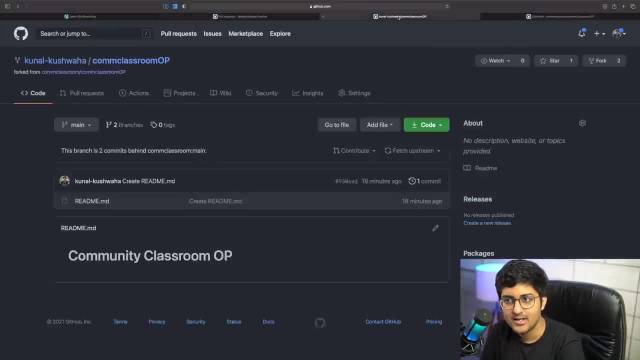 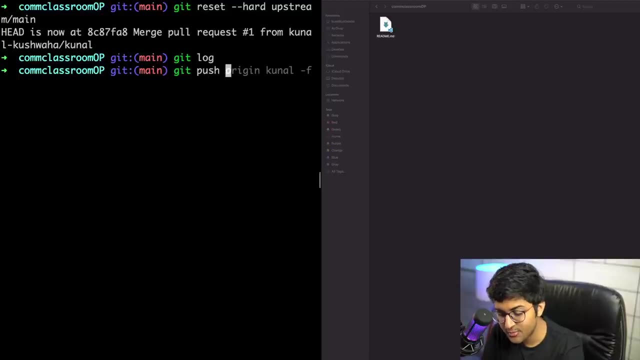 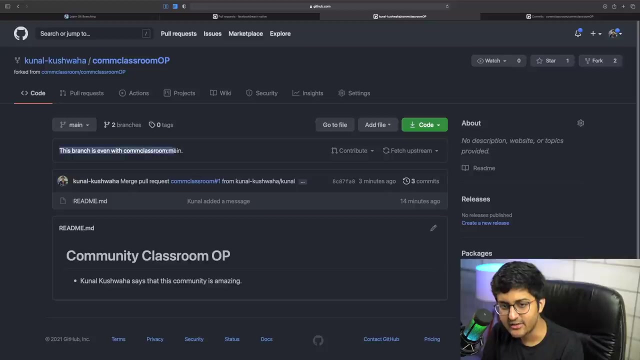 in upstream over here. let's look at my fork. it is currently also not updated because I have to push my changes. I can say git push to my origin. which branch do I want to push? the main branch in my local system. time to refresh this branch is even with the main branch commits. three same commits in my fork. same commits over here. 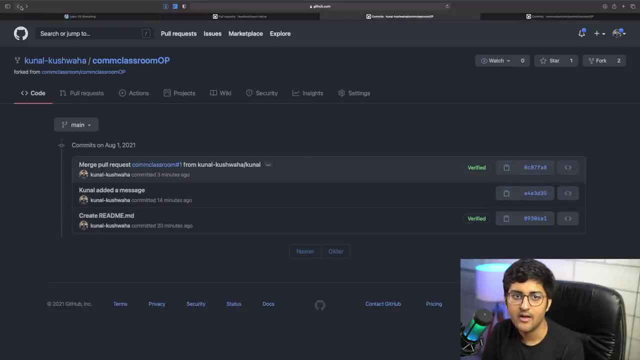 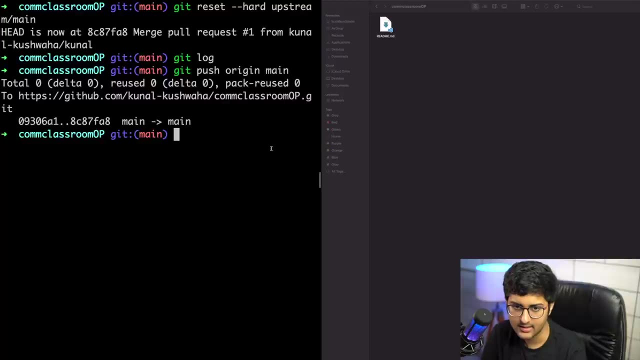 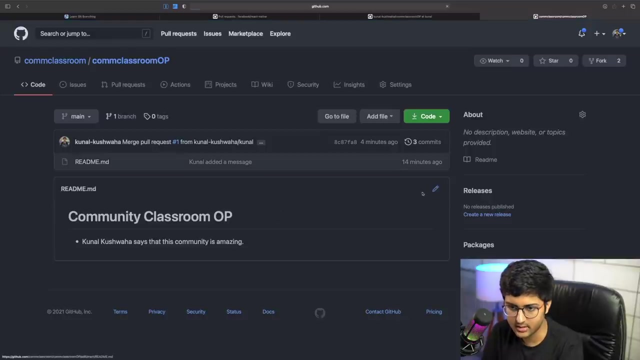 that is how you keep in sync with the main branch fetch. basically, you can also do something like this: get pull, let me just do something. let's say, let's say we create another, another commit over here. okay, let's say we create another commit in the main project, just for demo purpose, let me create another commit- they. 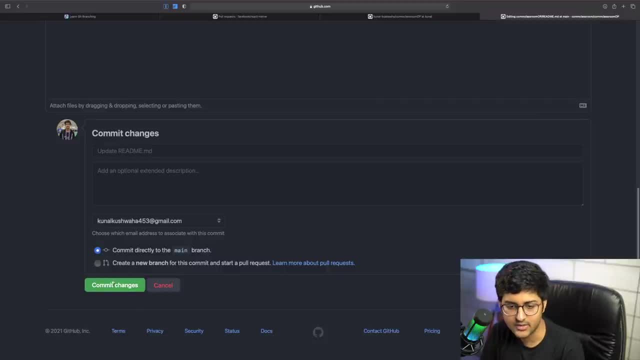 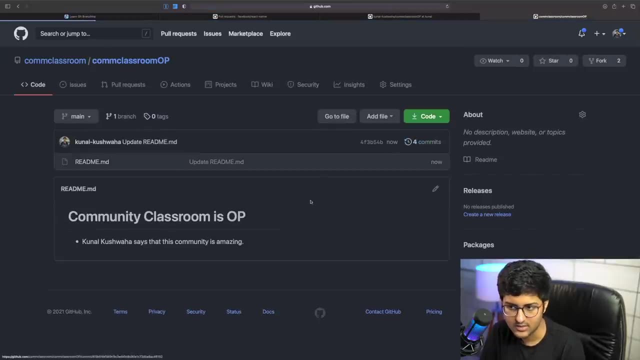 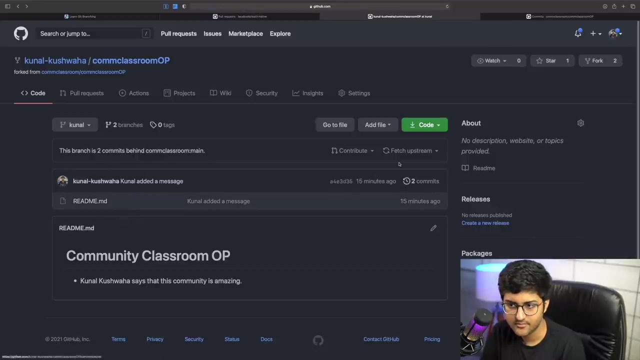 are is over here. I'm creating a directly, but don't like if for your project you can do anything you want for your personal projects. but yeah, now it contains four commits, because i just added one update readme and my only contains three commits. okay, so it's like. 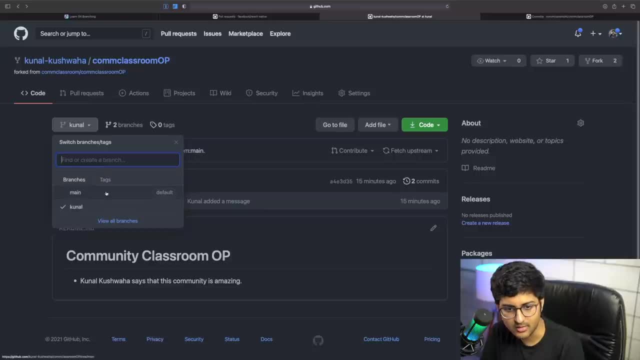 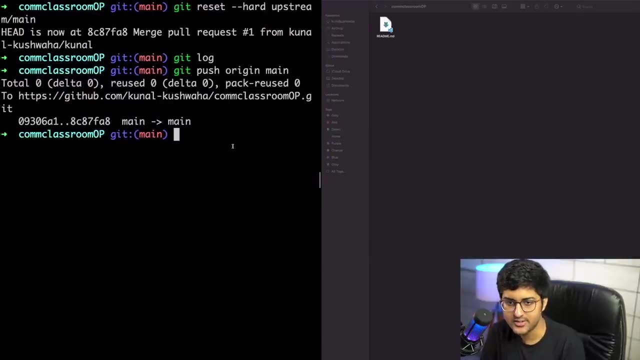 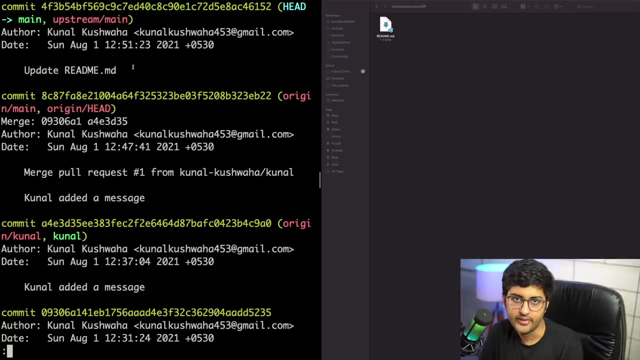 sorry, two commits. so basically it's like: oh no, not sorry, main branch, three commits, okay, four commits, three commits now. basically what i want to do is you can also do something like get pull upstream main, make sense. this is the same thing that happened. we did get fetch before get pull. 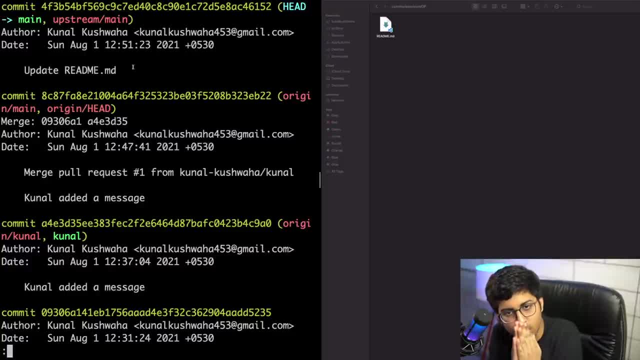 internally also does the same thing. i just showed you so that you can understand what is what is fetch, what is, you know, reset and whatever committing. so all of these things that we did previously were done in just one single command: get push- sorry, get pull upstream, upstream. 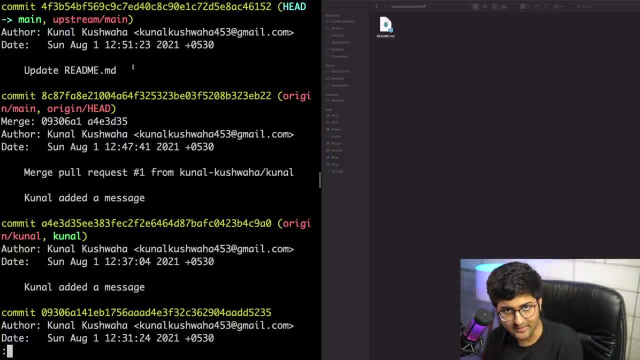 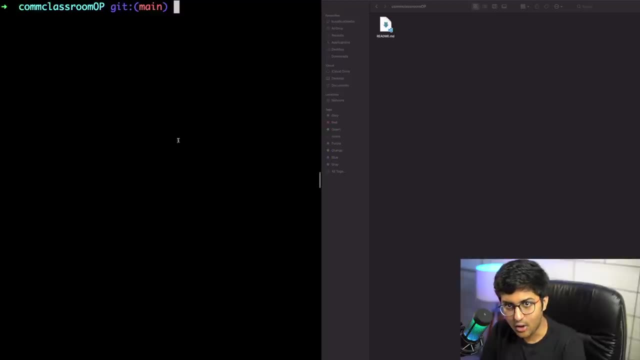 urls- main branch. so in the java code base, whenever you want to pull the code that i submit, you will just do git pull upstream main. that is what you will do. okay, now again, all the changes are in my local folder, only not in my upstream. so here only three commits are visible: git push. origin mean like: hey, my local folders main is in sync with the main branch, the upstream branch. let's also sync the origin url, then refresh requests. that is also about how you can get your prs merged. how you can create new branches is how you can make changes, how you can fetch with upstream- two ways. i already taught you one. 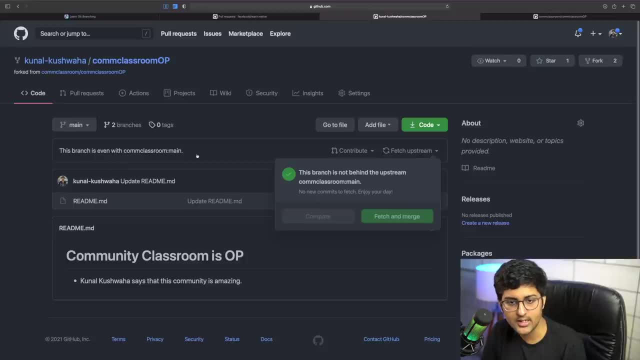 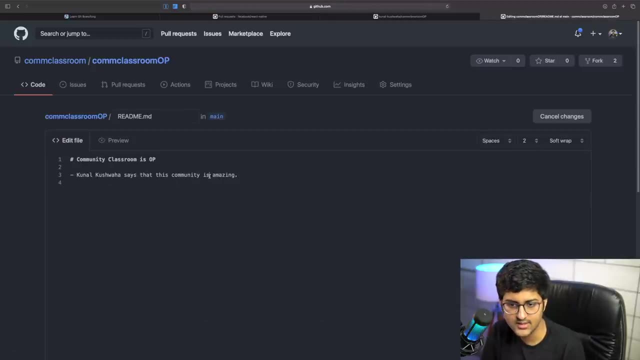 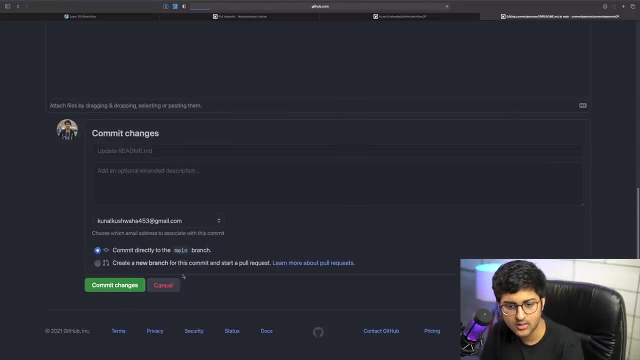 another way is you can just fetch upstream. currently it's already, you know, in sync so you can just click fetch and merge whenever you get a new, new thing added. so if i say i remove this thing, let's say, or i add some new commit, like an exclamation mark commit, i can fetch. 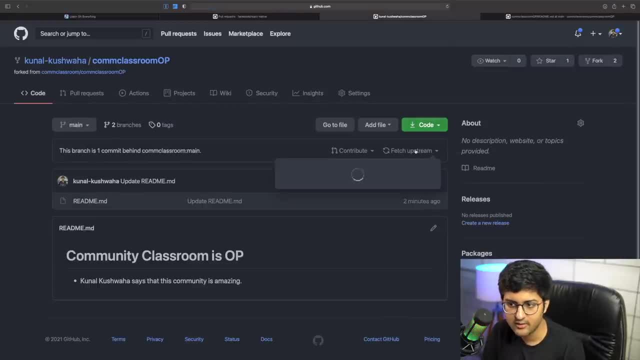 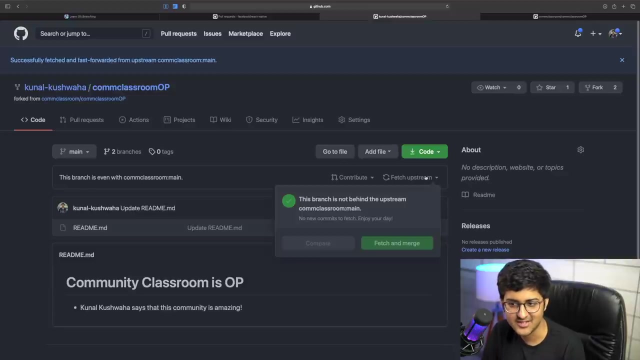 refresh. it contains five commits, but i only have four commits. fetch and merge- very simple. you don't even have to do git pull upstream main, just just click on this button. it will do it automatically for you. so i hope you are able to understand what is forking. i hope you are. 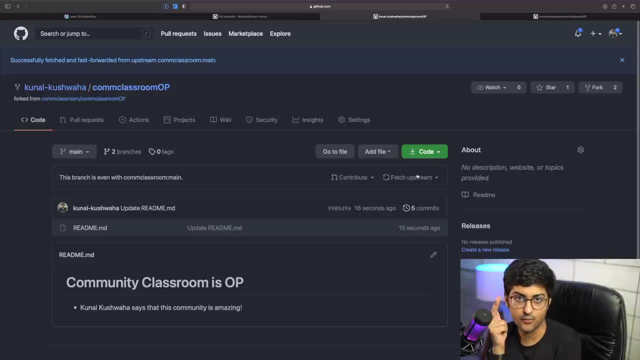 able to understand why we create new branches. i hope you are able to understand how we clone, how we get add date, commit, how we keep in sync with the main branch of the upstream. i hope you know what is upstream and what is origin. and now let's look into a few more intermediate concepts. so if you want to try it, 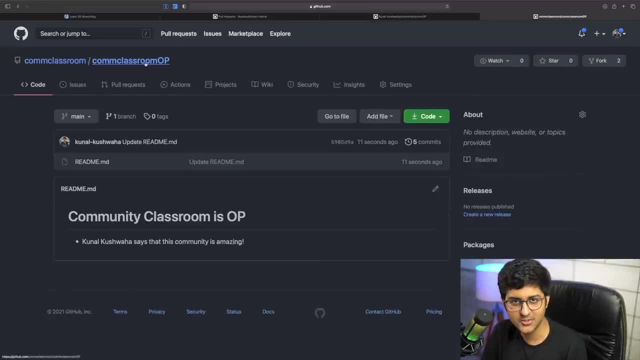 out hands-on. what i would recommend you to do is just go to this url. you know this particular one. i'll leave it in the description below. obviously, fork it on your own account, clone it, get. do do the same things that we did: get remote, add upstream url so that you can also fetch the changes. 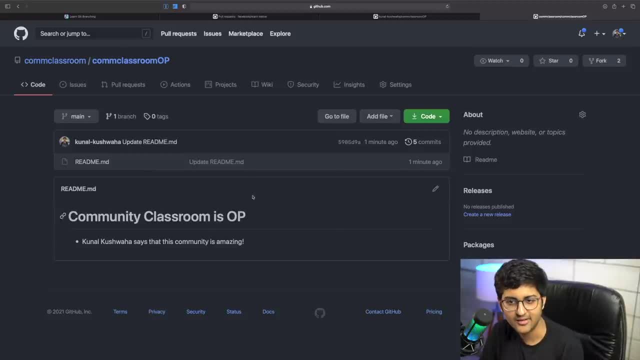 whenever changes are made, and then just write a line over here, update your branch like whatever new branch you create, and make a pull request, and then i will merge your full request and your changes will be visible in the main project. okay, cool, let's look into one more thing. so let me show you something else. there are two more things i want you to show. 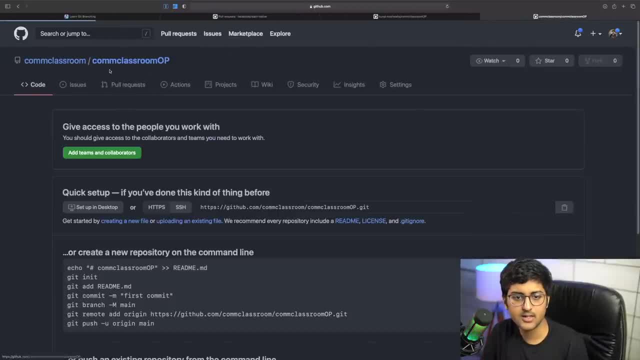 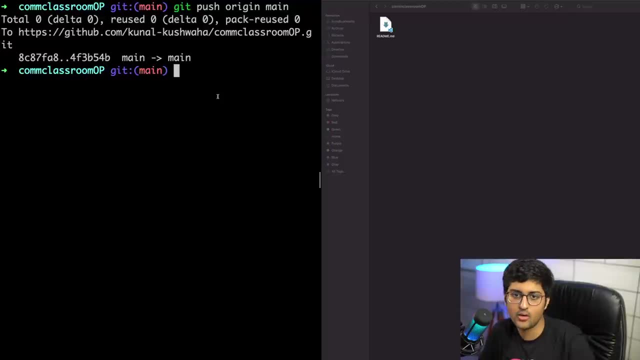 one is known as merge conflict and another thing is known as squashing your comments. okay, so if you have a lot of comments that you are working on and you want to merge that into just one commit, how do we do that? so i can say: git, check out my kunal branch, let's. 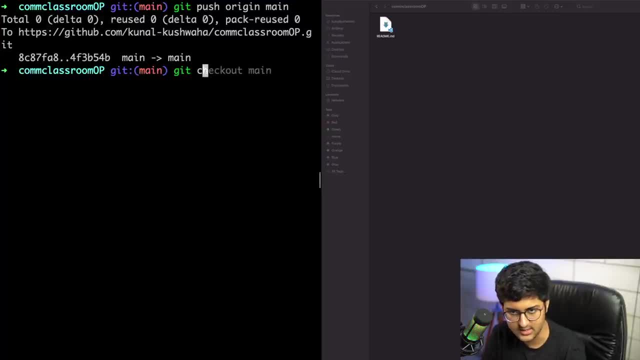 say or not, not kunal branch, some other. let's say, create another branch, let's say grid branch, temp git checkout. whenever you create a new branch, your new branch is going to be created from your head. so make sure whenever you create a new branch, your main or the master branch is up to date. 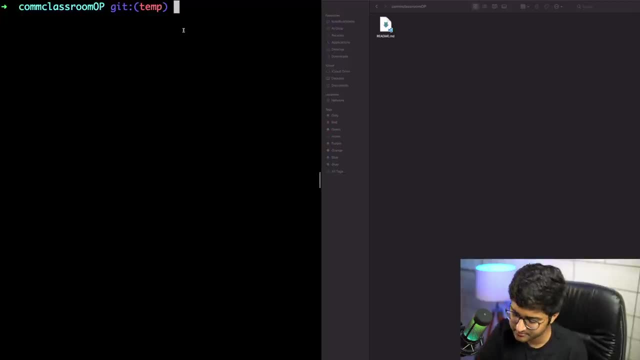 whatever things that we did, make sure you do that before creating a new branch. okay, so now let's say i want to show you how to squash commits in just one single commit. so how do i do that? touch one git, add dot git, commit minus m. i can add something like: 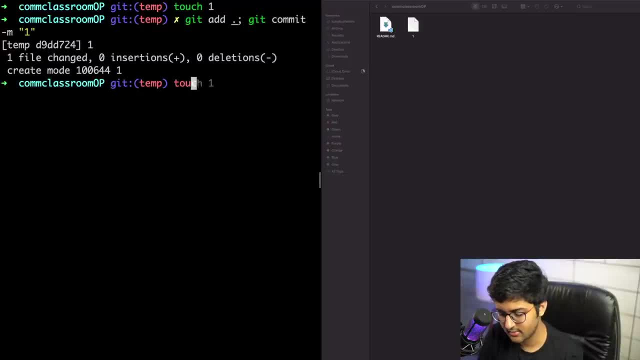 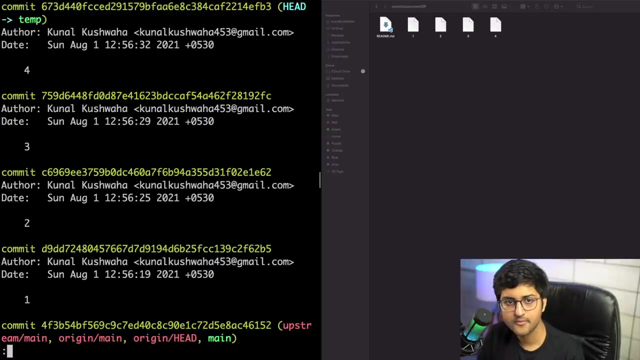 one, okay, and then i can say: touch two, just creating random files, uh, i added two. then i can say: touch three, added three. then i can say: touch four, added four. whatever git log consists of all these commits. i want to merge all these commits in one single commit. how do i do that? you? 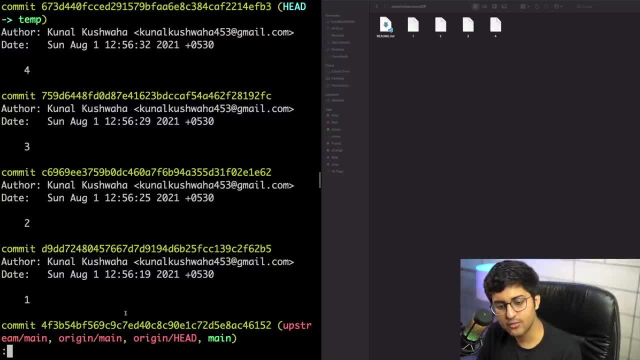 can use the rebase command for that. okay, a few a trick you can do. it is if you want to merge all these commits or if you want to merge just these two commits, for example. if you want to merge all, you can just reset. you know, if i reset this, this will be unstaged and then you can commit again. 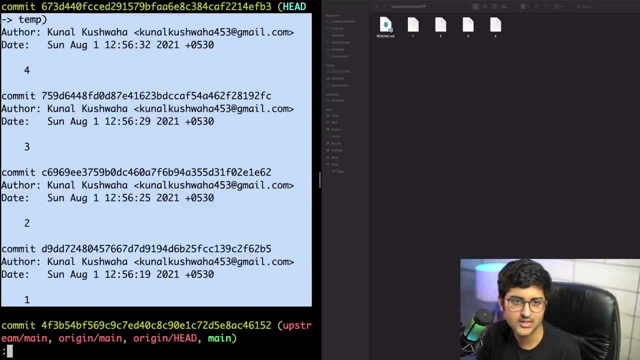 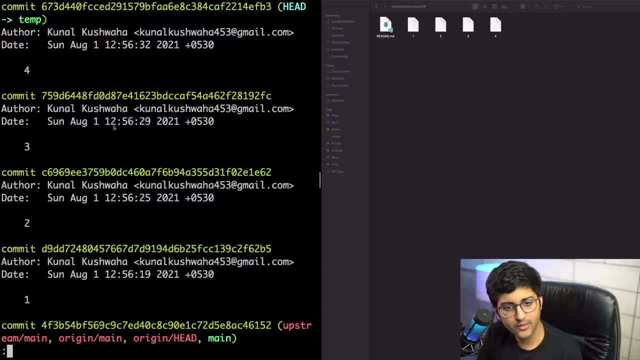 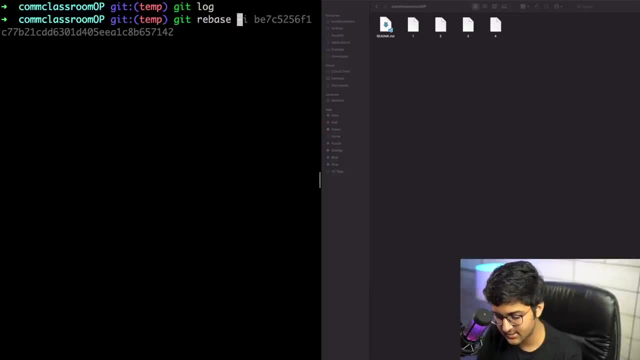 you know that right when we, when we reset this thing, all the commits above it will be on the staging, on stage area. get them on the staging area and then just one, one single commit you can make. but we are going to try something different. i copy this commit and i say git rebase minus. i means the interactive environment. copy. 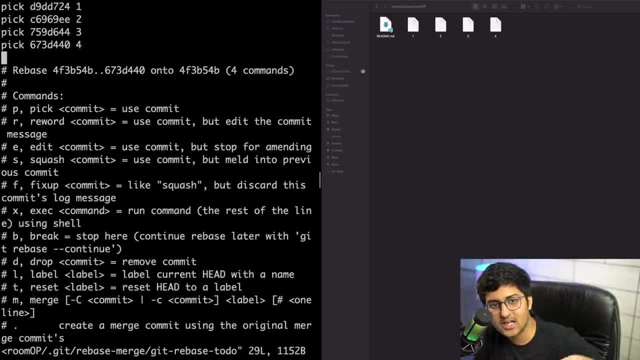 so you can see now all the commits above it. i can either pick or squash. so if i say squash, squash, these will. these will be squashed into one single commit in the pick. so this main commit that we had one, these three commits will be updated in this commit. okay, squash. 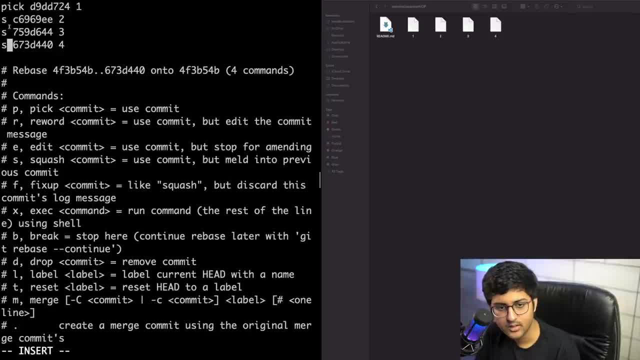 basically means whichever one is listed as pick, merge it into the previous commit, so these two will be merged here. let's say you only want to merge the middle two, then you can just do. these things will be merged in this one, so these three will be one commit. 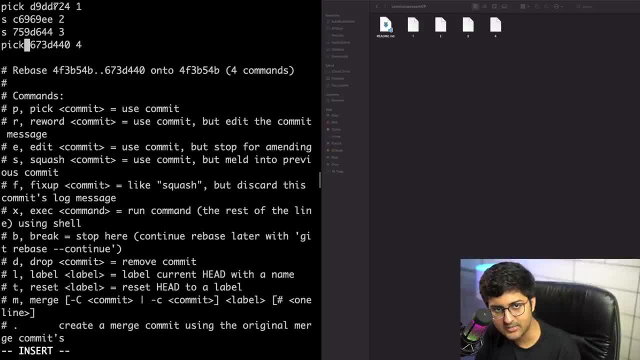 this is basically pick and squash. pick basically means you are taking this commit, i want this commit. squash basically means above, above these s, whichever pick you have, merge your commit in that. okay, let's say, i want to merge all the three commits, all the all these three commits in the 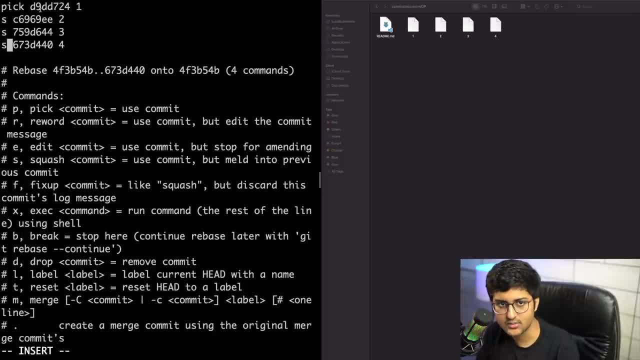 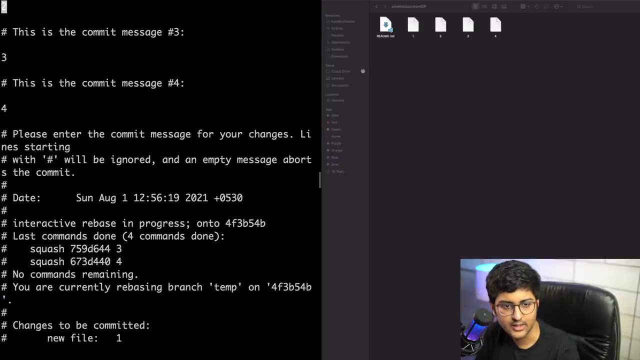 above commit. so i will make all of these as squash and this one as pick. exit out of it. escape colon x. it will now allow you to create a message for this new commit. so my message can be something like: i'll add a new message over here. i can say: 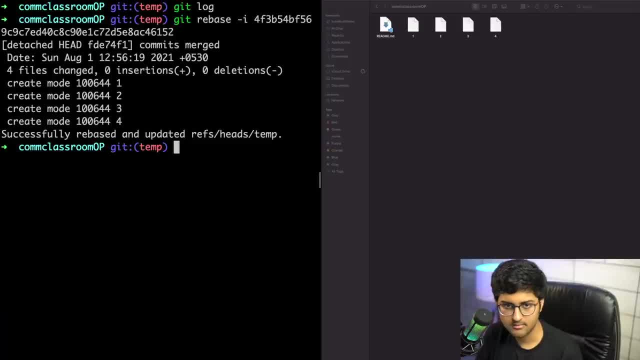 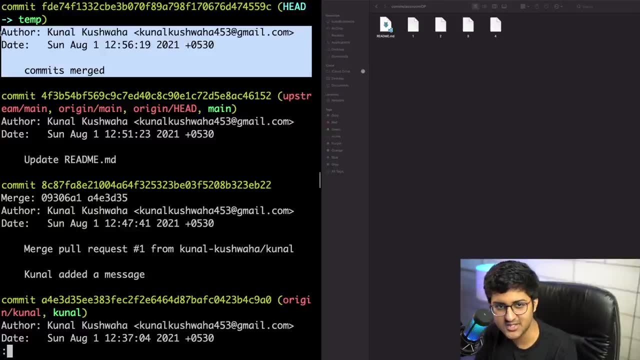 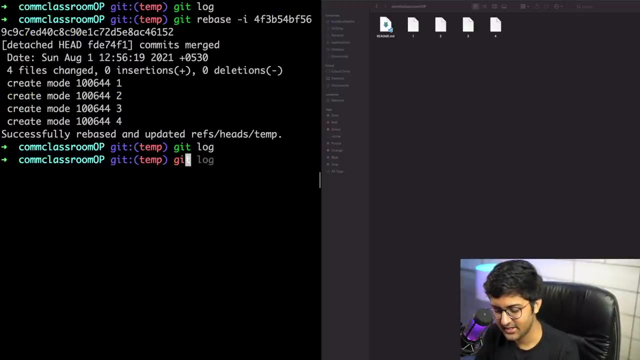 commits merged. colon x back git log. tada, one, two, three, four are gone. all of them are merged in just one single commit. awesome, that's how you merge your commits again. you can do simple git push, origin, whatever you want. uh, temp branch. so these all files will be available over there. i don't want these files. 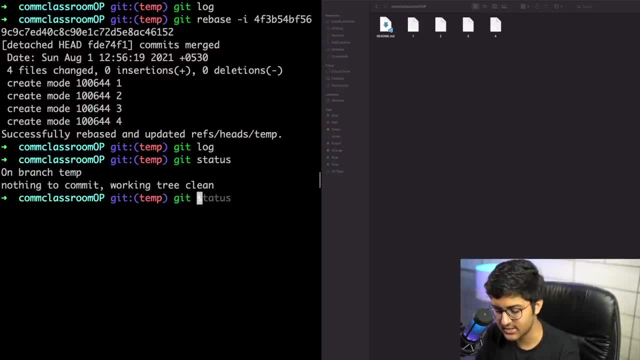 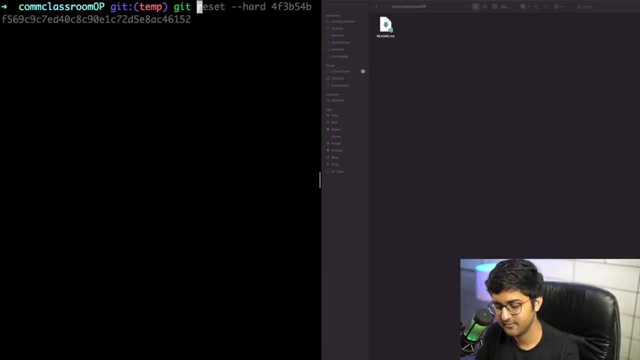 so i can remove these. get status, so not get status, get log. this is what i want to remove. this is the commit that created these four files. copy this. i can also do minus minus hard. gone hard will actually reset it with hard, so do it with caution, okay. 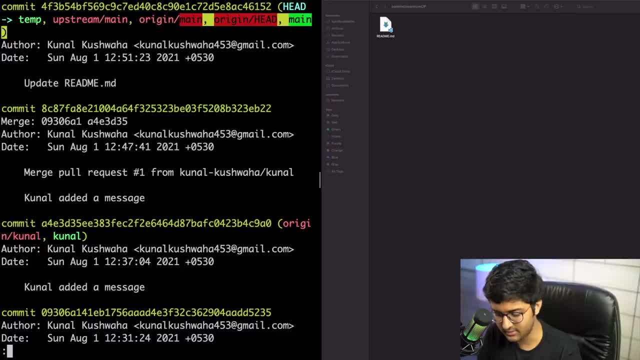 so origin? why does? why does this thing keep coming nevermind? origin is also same at the same commit. upstream is also at the same commit, my head is also at the same same commit, uh like in the origin. the head is also over there and my main branch is also here. 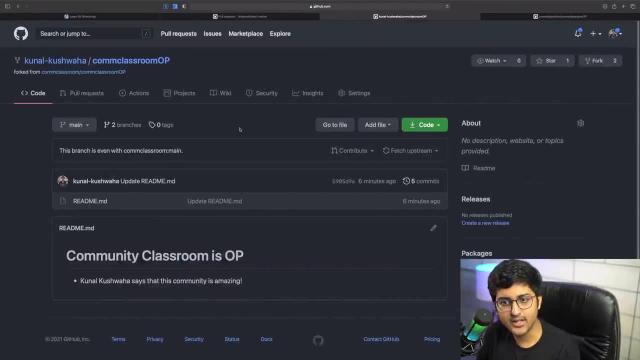 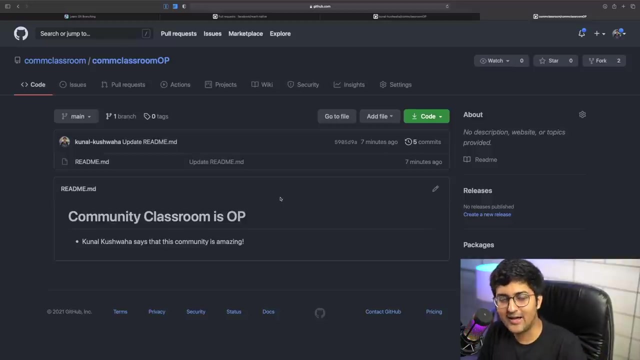 very nice. okay, last thing remaining is merge conflicts. what are merge conflicts? how we resolve those now? what are merge conflicts? let's look into that. merge config basically means that, uh, let's say you changed in a file, let's say you made a change on line number three. 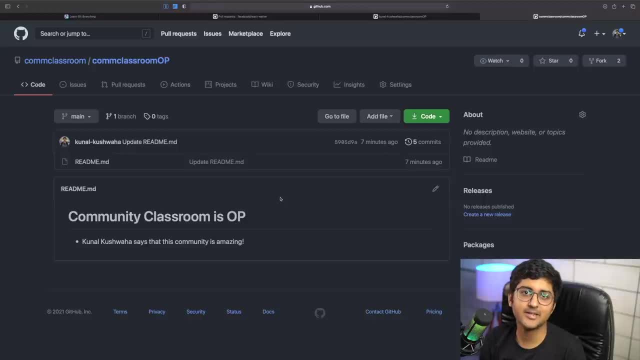 okay, and someone else also made a change in line number three and there was a change in line number 3. now git will get confused. should i take your changes or should i take that person's changes? which change do you want me to take? git will get confused, so git will ask you for help. hey, please. 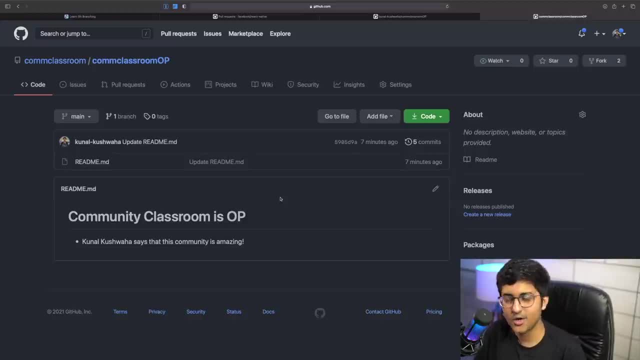 help me tell me which change you want to take. you want to take this change or you want to take that change? because both of you people have modified the same line number. let's see how we can imitate this thing. let's try to get a merge conflict first. so let's say i create a change in line number four. 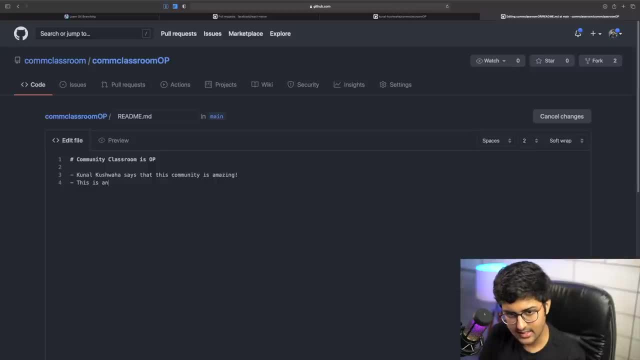 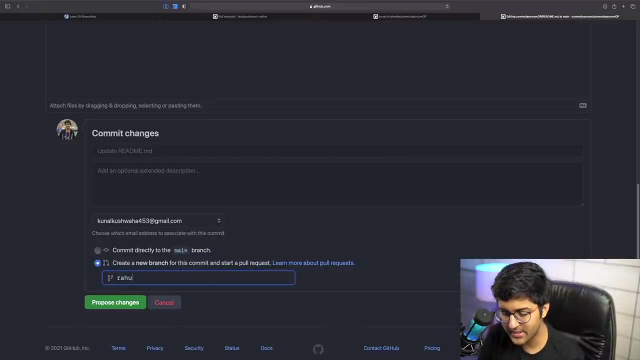 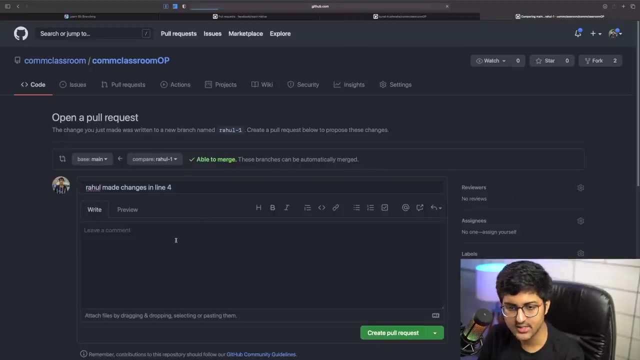 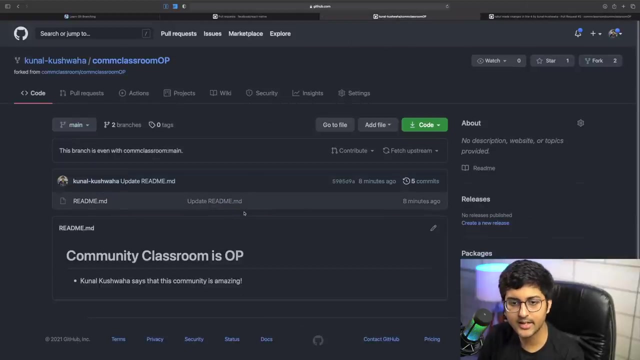 and i create a. this is an example to make a merge conflict. okay, so i create a new pull request, create a new branch and a pull request. i can say: rahul made this change. for example, okay, rahul made changes in line four. rahul made changes in line four. that is okay. and let now. let's say i create a new. 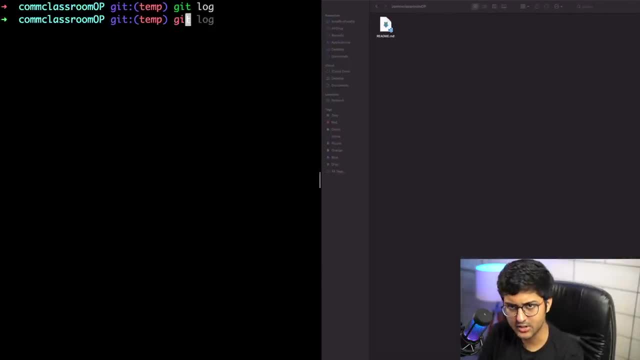 branch as well. let's take the temp branch. only make sense. let me also change line number four. so me and rahul, both are changing line number four. only git will get confused. git will be like: what are you doing? which line do you want me to? 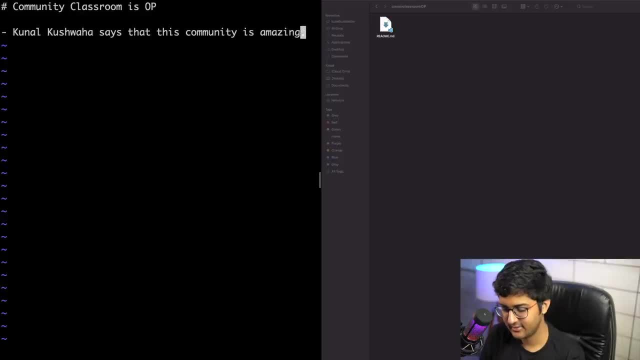 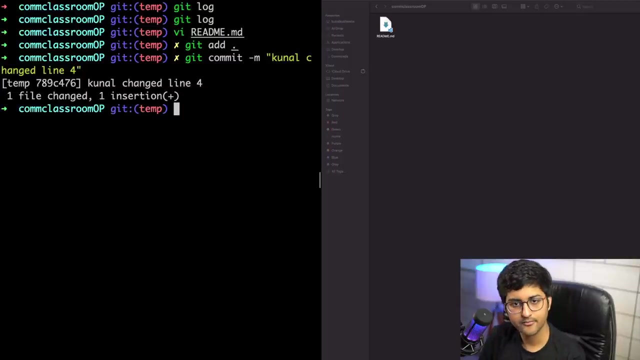 check. you want me to take rahul's line or your line so i can say kunal made this change. okay, git add dot. git commit minus m. kunal changed line four, then i'll just open a pull request. i have to push it, git push. 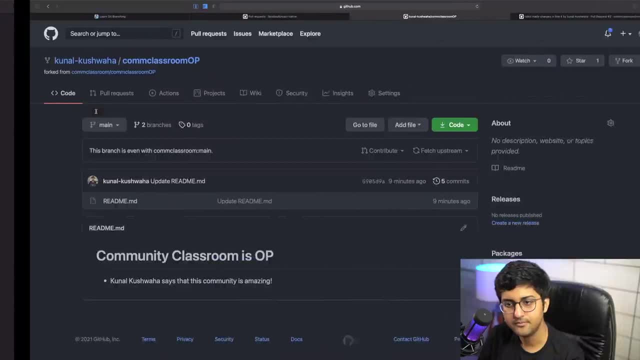 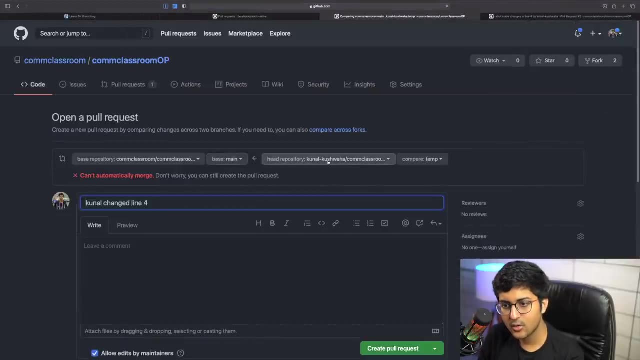 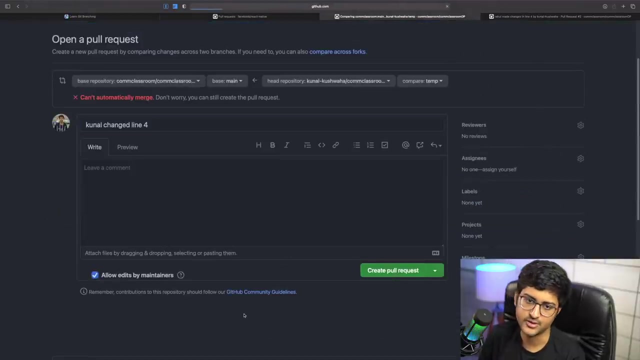 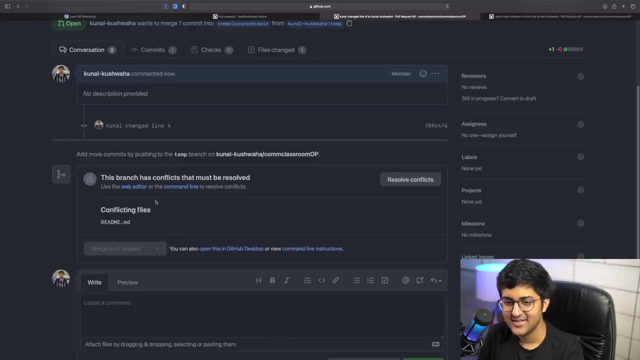 origin temp compare and pull request. hey, kunal's temp branch, please merge it into the main branch. i'll be like, okay, cool, let's merge it. create a pull request. okay, let's do merge config. it's currently checking. there you go, it's giving me merge conflict. now with the readme file. 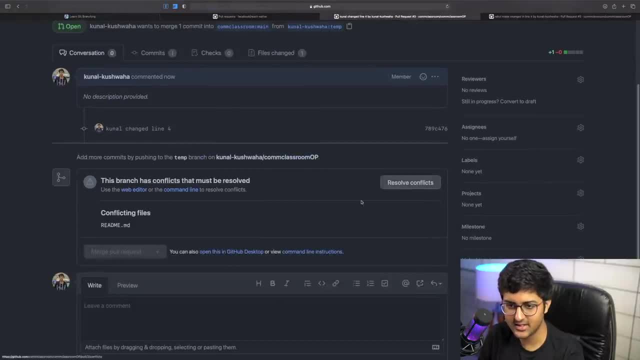 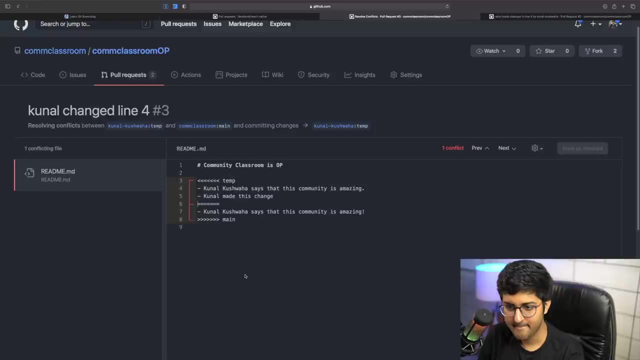 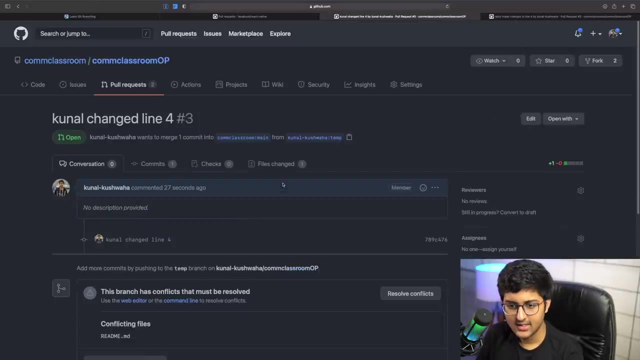 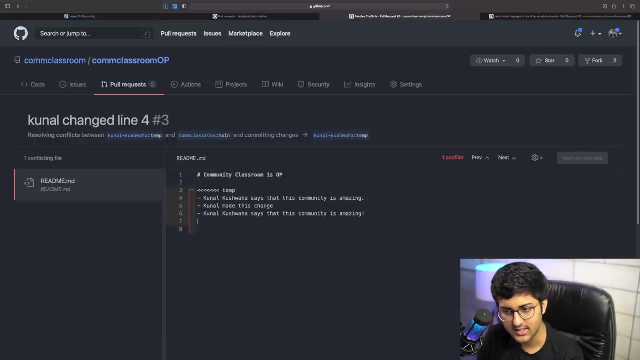 current. it's giving me with something else, but let's see what it's giving me conflict with. yeah, there are some, some conflicts over here for some reason. but uh, let's say i make, let's say i resolve these for for now. let's say i resolve it like, um, let's say i check these only, that's fine. 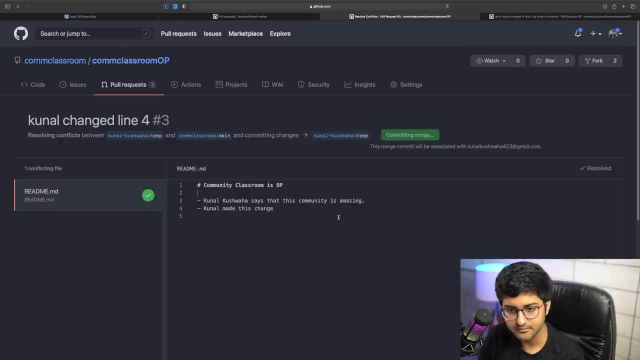 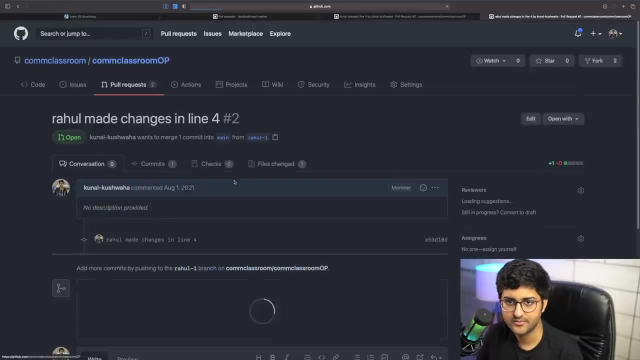 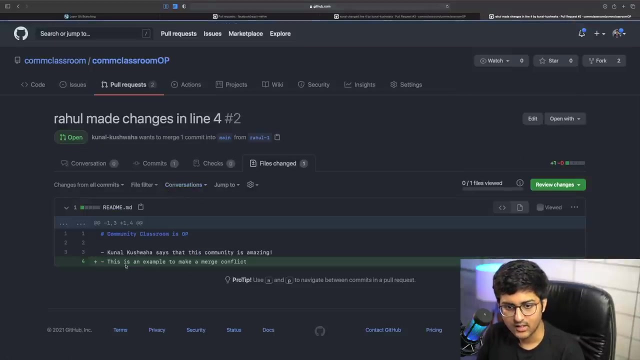 mark as resolved. confirm, okay, commit. let's say what we want to do. is that, uh, when this pr will get merged, rahul's pr? okay, let's say rahul's. this is an important point. we both have changed line number four. rahul changed line. 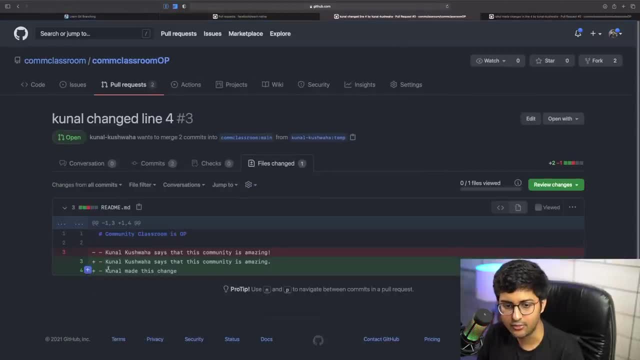 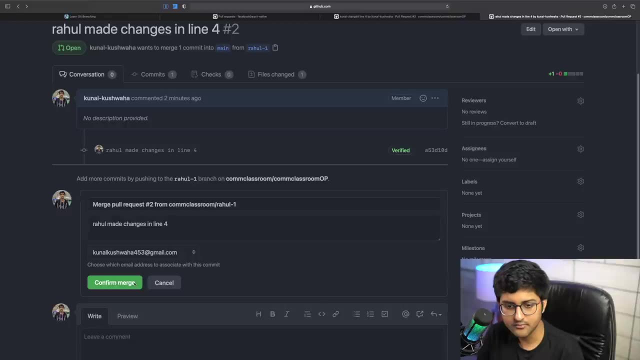 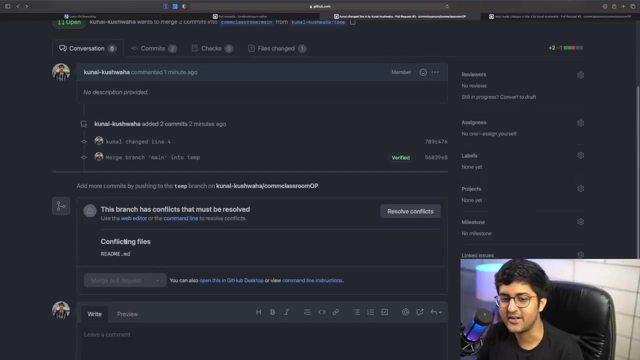 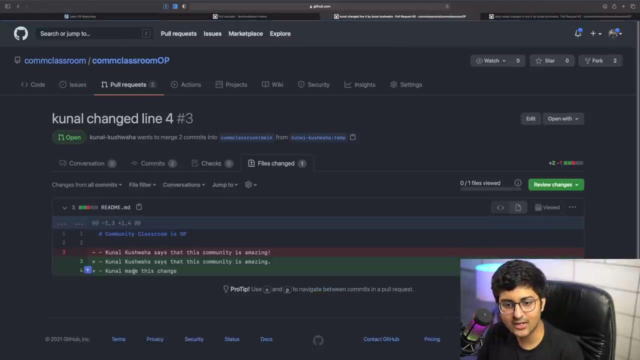 number four. i also changed line number four. okay, now what is going to happen is: let's say, we merge this pull request, this is merged, let's refresh. now it's giving me conflict. it's like: hey, rahul just got his pr merged in line number four and you are trying to change that. only which one do? 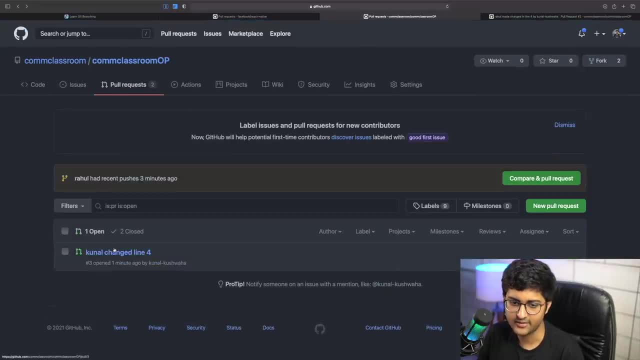 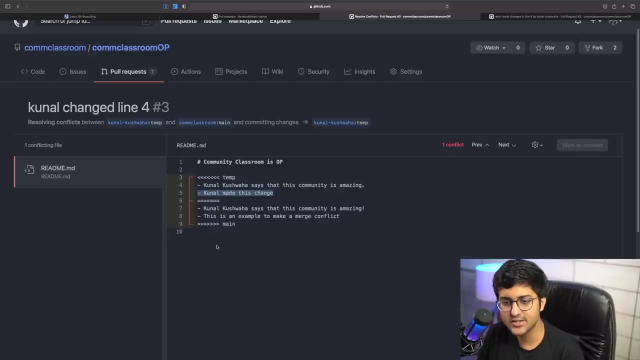 you want me to take that is a merge conflict. okay, so i would have to resolve it manually. so even here you can say that kunal made this change, and here you can say rahul made this change. this is my change. in line four, this is rahul's change. so it's saying: hey, you. 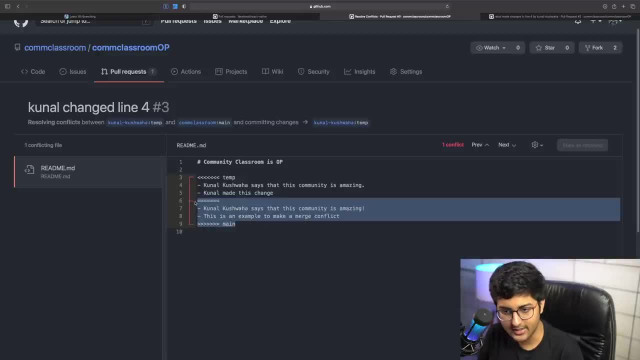 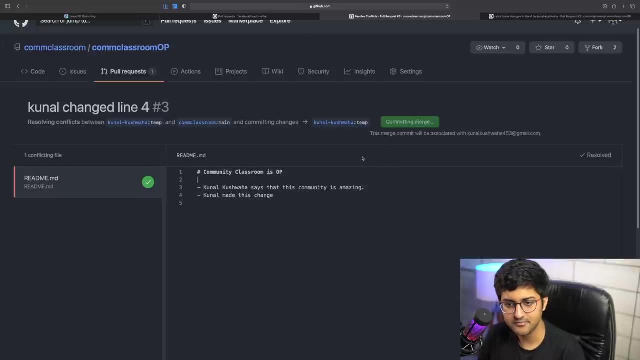 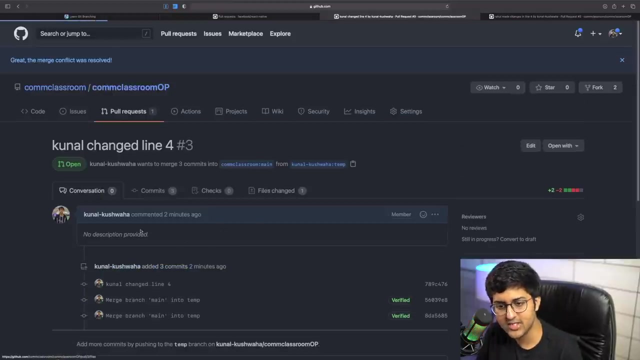 want to take this one or you want to take this one. i'm like, okay, i want to take, i want to take this one. i don't want the main one, i want my own one mark. as result, commit, merge. okay. so i overrid. i did the overriding of whatever change rahul made. so this change was made by rahul and i removed it. 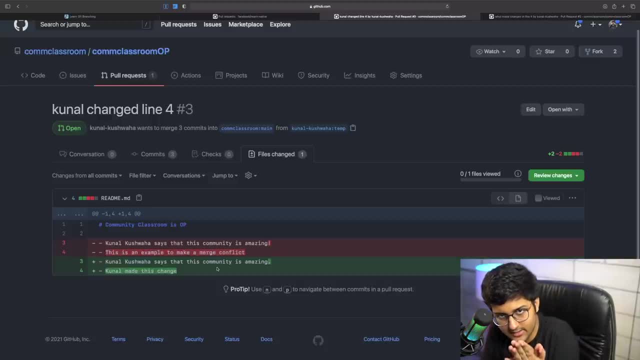 because it was a branch being created. you know, when i created it it was from the master branch, so that from the main branch. it's like: hey, rahul made a change at line five, you also made a change at line five. which change do you want me to take? it's like: okay, fine, take my change when i merge this. 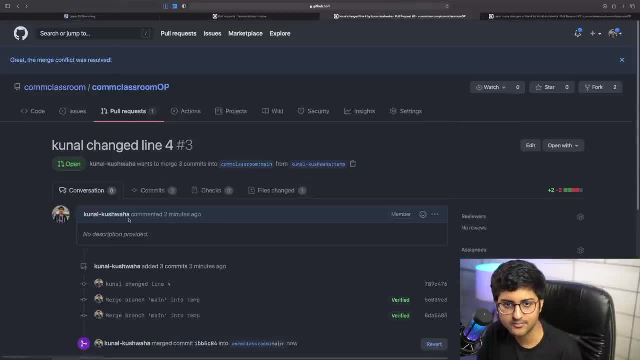 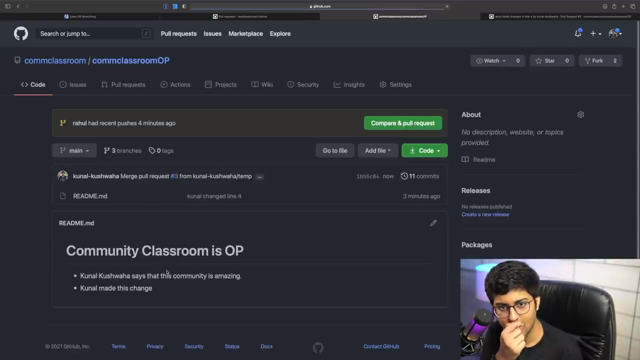 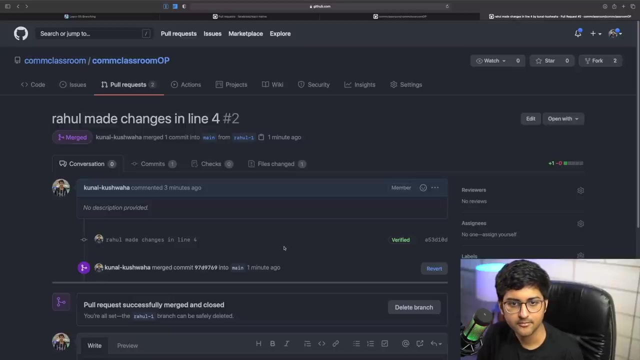 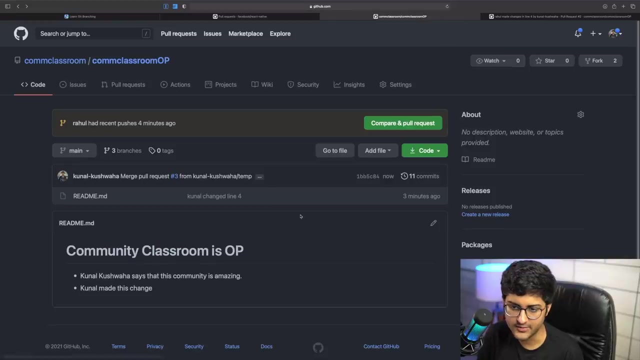 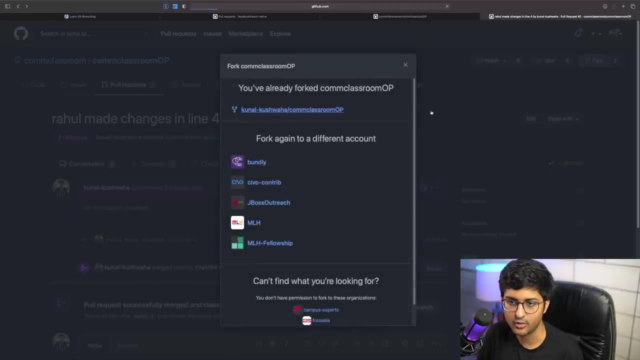 pull request in the main branch. you can see now my changes are available. rahul's are not available. hope that makes sense. cool, alrighty, so you can see rahul can open up vpr over here as well. cool, now we're going to our fork again. um, where is my fork? 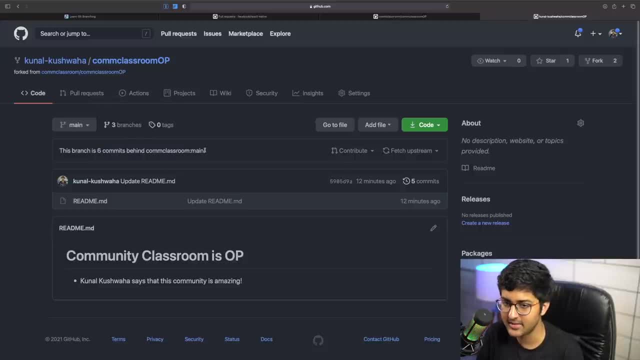 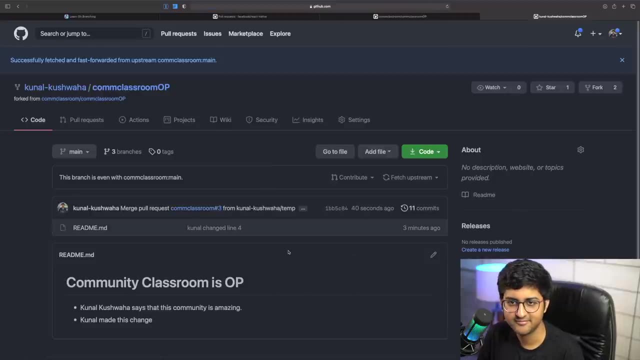 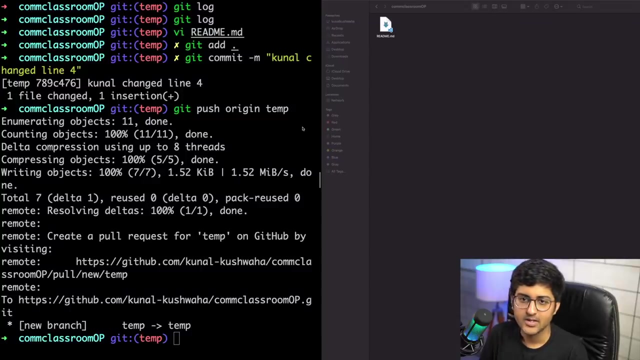 so in my fork over here i can see that this is six commits behind the main branch, fetch which and merge. now it's even pretty cool stuff, alrighty, alrighty. so that was about this session, and that is more than enough for you to get started, even with open source contributions. one last thing i would like to share is no matter. 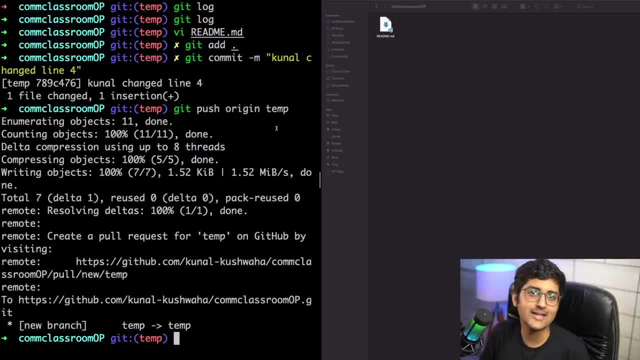 how many videos you watch. if you are not able to apply these things practically and actually get stuck and then resolve the doubts and everything, you will not get the intuition behind it. so get some hands-on practice. you will get some hands-on practice and when you will be downloading the code. 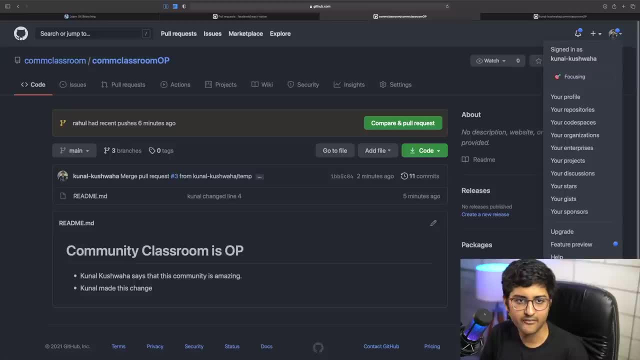 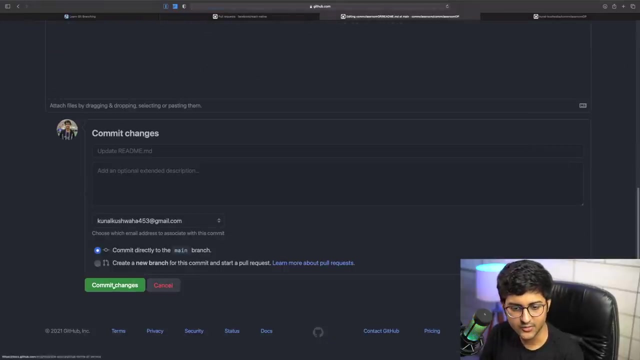 sample that i share in community classroom. so basically, here we have the. so first thing i wanted to do is actually create a pull, make a pull request in com classroom op. so i actually make some changes over here. i'll basically make some change like: uh, make some changes over here. 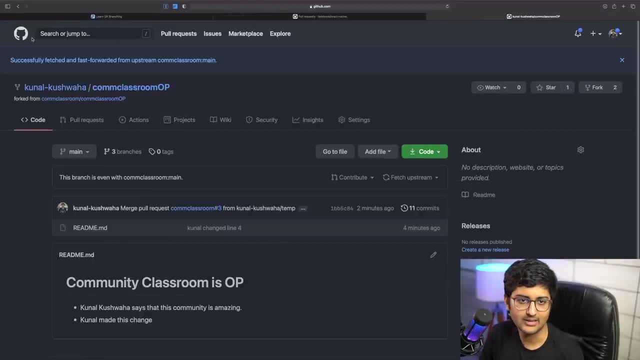 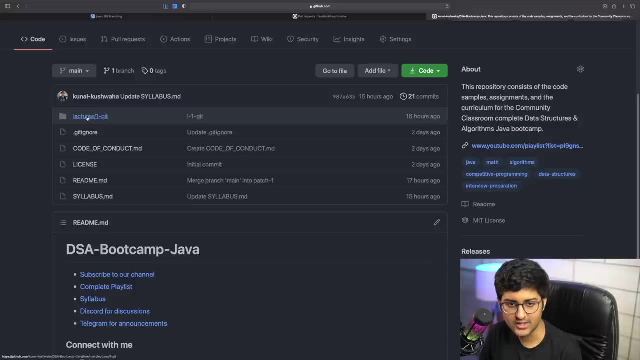 okay, share about what you liked and everything. and the next thing is: uh, all the changes, that are all the code sample and everything i'll be submitting. it will be over here. so in the lectures folder here i'll be sharing all the lectures. you can see, git cheat sheet is already updated, so all 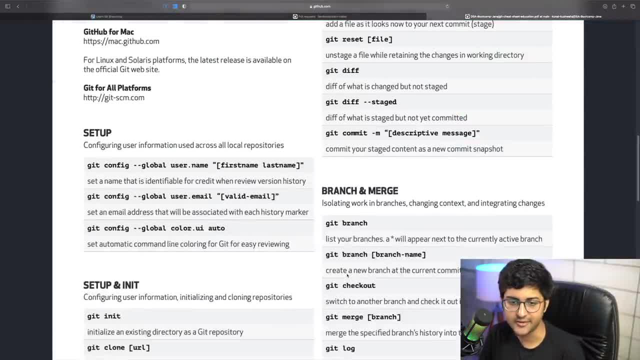 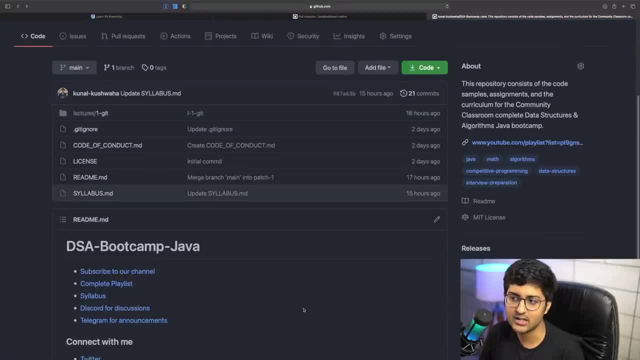 the commands and everything that we mentioned are available in this cheat sheet by github. okay, so rewriting history and everything, some some more advanced concepts, but this is more than enough for you to get started and everything you need. all the code samples i'll be uploading over here for. 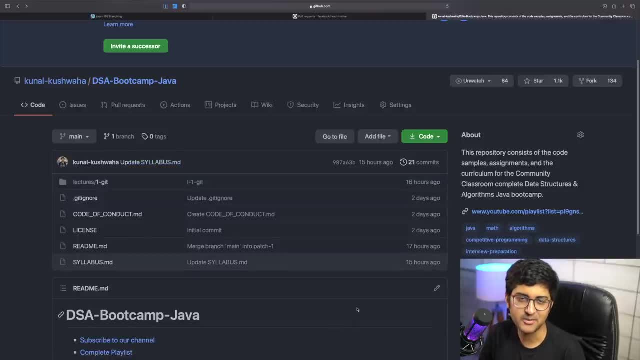 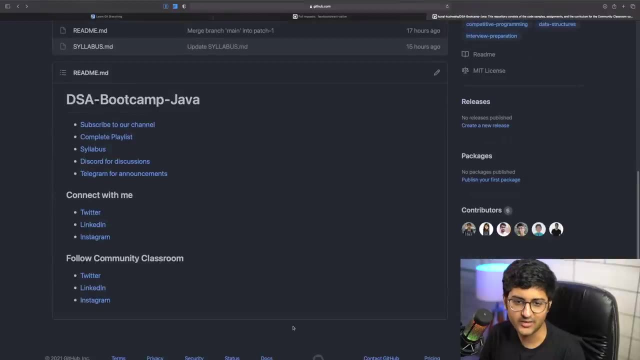 the complete data, such as bootcamp. make sure you share and subscribe to this video and like. if you have any questions, we have the discord channel. all the links are in the description and, uh, looking forward to your pull requests and everything you know and yeah, thanks a lot for watching and do check out the links in the description.